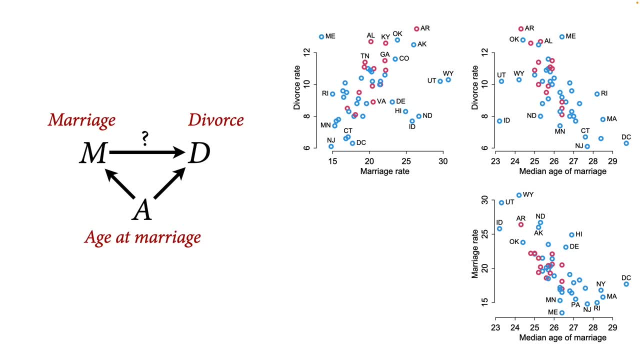 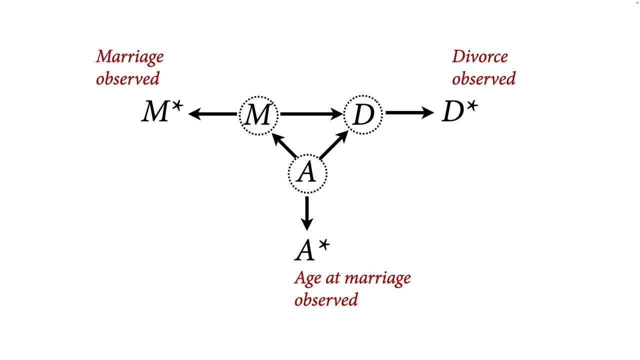 posterior distributions, And the most practical way to do those calculations, to do the calculus, is with random numbers. So let's revisit, for example, this marriage-divorce-agent-marriage problem that I used to introduce. the elemental confounds What I disguised from you in this. 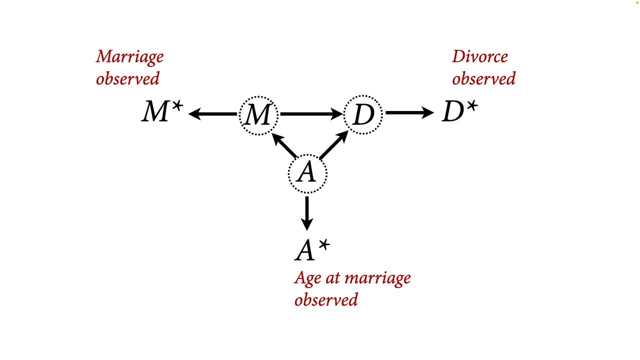 example is: we haven't actually measured any of the three variables in the example. We've only observed their descendants, some error-prone estimate of it. any particular region of the United States. There's age at marriage. There's a distribution of the ages of marriages that 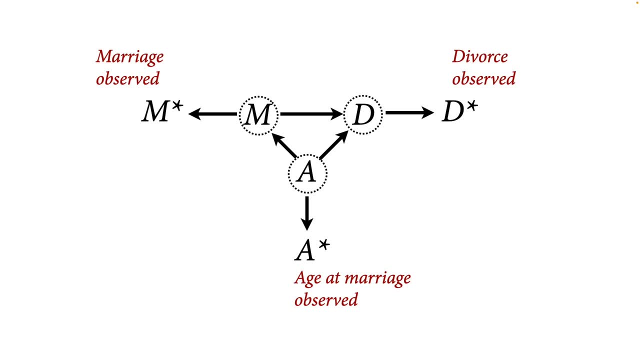 people tend to get married in that region. There's the marriage rate And there's the divorce rate, But the data that we have available, that I've made available to you as part of the course- are only finite samples of data that are used to estimate those things, And 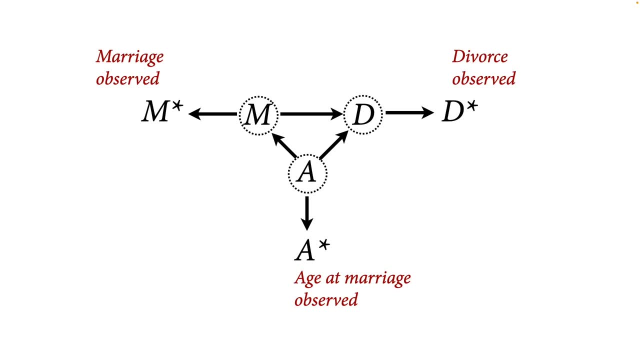 so these are actually estimates And the true things we have not observed, but only the estimates marked here with the asterisks. how do we take into account the inaccuracy that is part of these estimates and do the statistics honestly? This gets even more complicated when we realize that 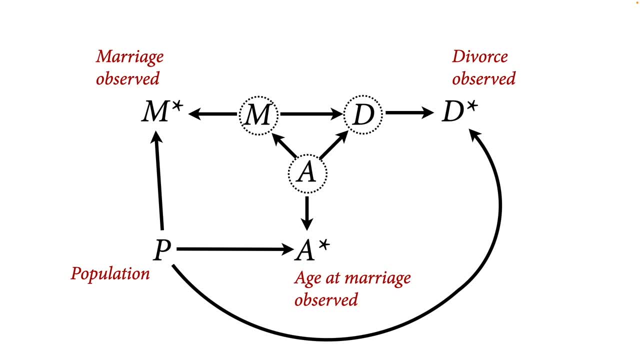 of course, there are other variables that are influencing the inaccuracy in different regions, like population. Smaller states have more inaccurate estimates of these three variables than larger states. Why? Because there's just less data And therefore there's different amounts of. 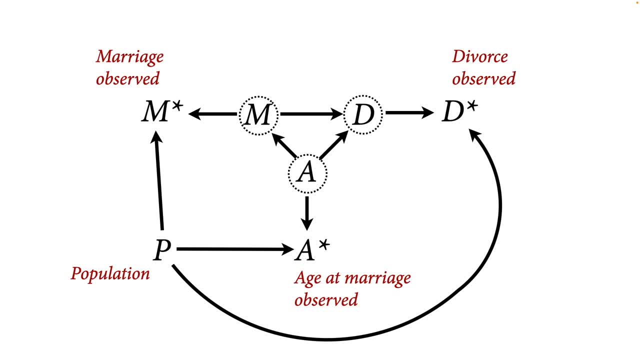 reliability, but there's also different ways of estimating the accuracy of the data. So if I for for the different amounts of data in each row in the example i gave you, we can solve this problem statistically. well, solve is a strong word. we can address it honestly and transparently statistically. 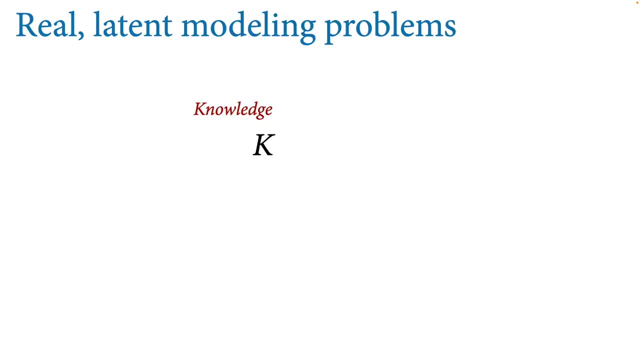 but in order to do that we're going to need some new machinery. another example, and one we'll deal with more today there are a large number of important measurement problems, inferential problems in science that have the same basic structure, and it goes something like this: suppose you're teaching a class and there are a bunch of students in the class and what you want. 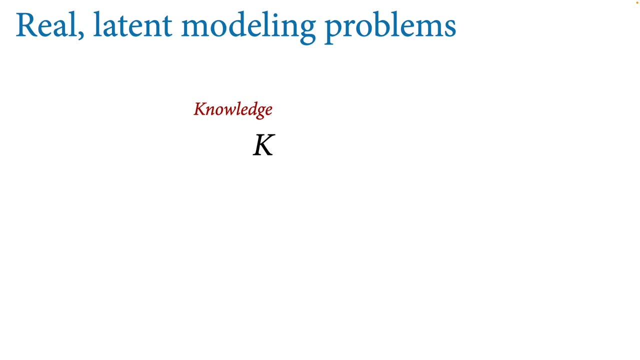 to do as an instructor is well: instruct them first of all, but then you want to assess their knowledge. is the course working? should you quit your job? so imagine there's some variable k here that represents the knowledge of a student, and what we'd like to do is assess their knowledge, but we can't do it. 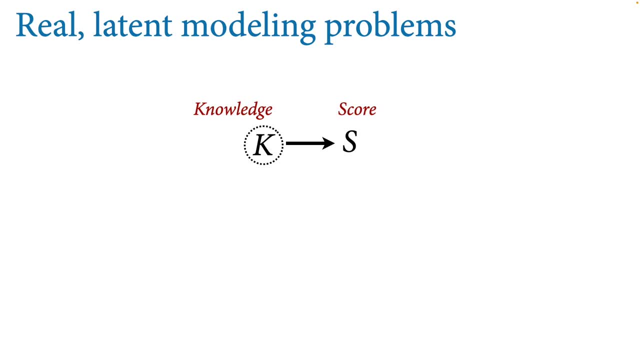 directly because we can't read their minds. there's no way to peer into their brains and know what they've learned. instead, we can do it right away, can only ask them questions or give them tests or homework assignments and we can score those homework assignments. but this is obviously just a proxy for their knowledge. it's not 100 correlated. 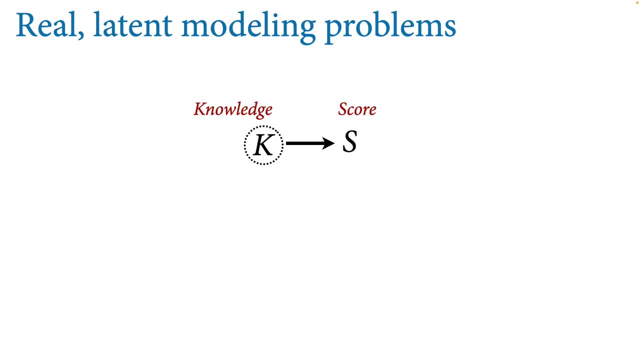 with it. it's a pale reflection of what they know. um, it's also true that the test or instrument you use to assess their knowledge has its own hidden properties which we may not be aware of, like, for example, how hard it is when you- just when, when you or i- design a test or homework assignment. 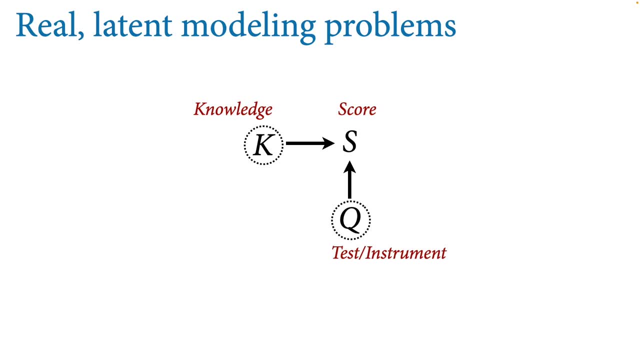 we have some sense about how difficult it is, but we're often wrong about that. and then there are features of the person taking the exam that may influence their knowledge, how much they've learned and so, for example, how hard working they are, how much they study and there. but there also may be features other than that directly influence the score. 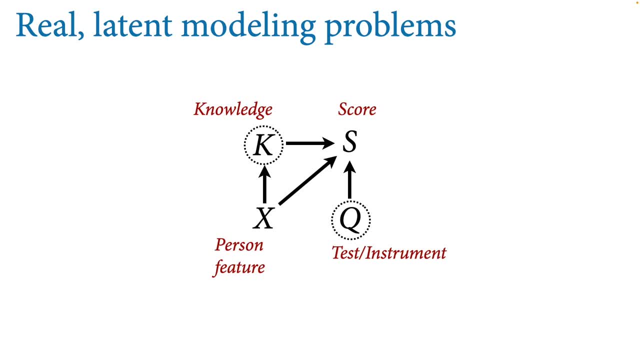 because of the biases of the tester instrument, right things that aren't actually a reflection of their knowledge but nevertheless lead to biases in scoring lots of important measurement problems, both in science and outside of science have this same causal structure where there are unobserved or latent 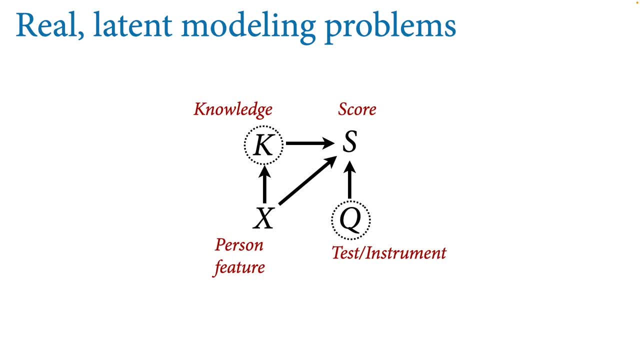 variables like knowledge and the features of the test or instrument or assessor or judge that influence the scoring, and so scores are hard to interpret but we must interpret them. for example, many people end up being judged for promotions or jobs or grants, or their papers get refereed for journals, and this sort of setting has the same basic structure. there's the 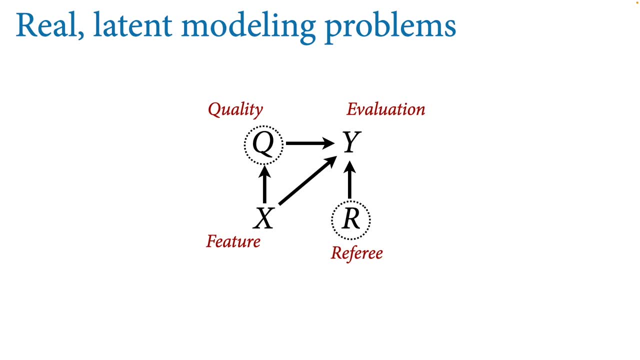 quality of some item, whether it's a job candidate or a paper or a grant proposal, and those items have features and they're assigned evaluations by some referees. those referees have hidden properties, like how harsh they are or their biases, and those things interact with the features and the quality of the item itself. to produce an observed evaluation, we want to infer 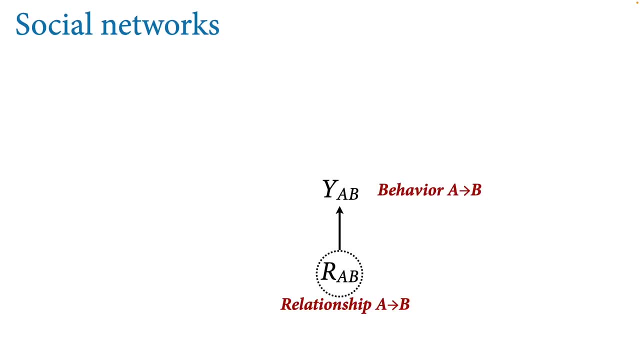 quality. how do we do that statistically? one more example, and then we'll get to the meat of the work of this lecture. i'm just trying to prime you for the things that we're going to be doing going forward, using the tools that i'll introduce to you today. social networks- very important part of the 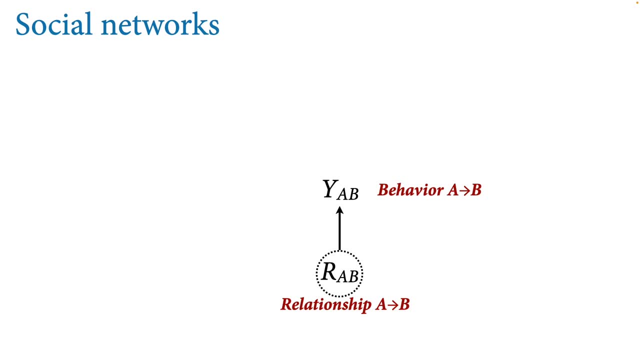 behavioral research, because people have relationships and when you study those relationships there are lots of awkward statistical things that arise. for example, suppose we have observed some behavior here: y a, sub a, b. the a b means it's a behavior from individual a directed at individual b. this could be a gift, yeah, or a christmas card, or taking a takes b to the airport, and we think that. 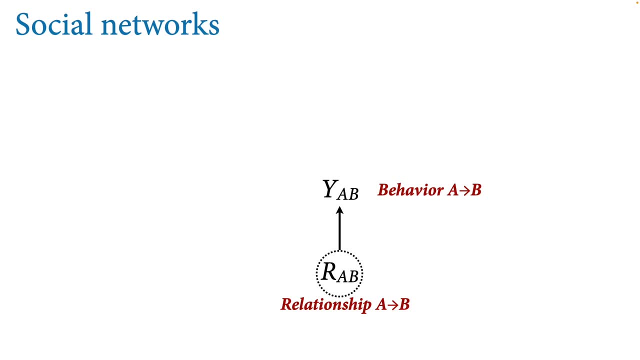 people do nice things for specific other people and not uh, third individuals say c or d because of the relationship in the dyad, this relationship of a and b, but we can't observe this relationship directly. this is the network. are these directed ties that are the, the invisible relationships? 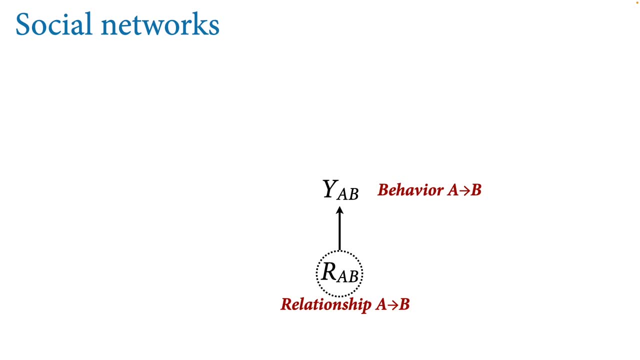 that explain social behavior, and we want to infer the network. what we mean is we're inferring some, some complicated structured latent variable, and it's not just, uh, the relationship of a towards b, but also the relationship of b towards a, because it doesn't have to be symmetric, right you might? 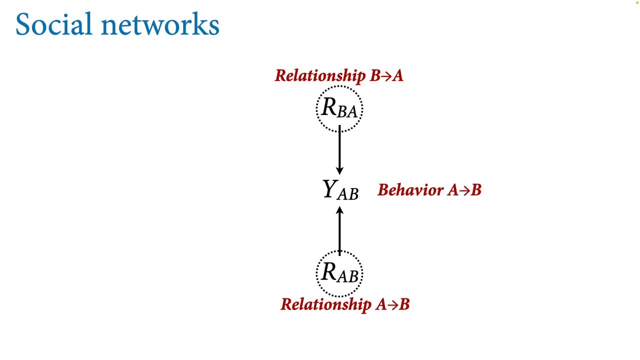 think that someone is your friend, but they may disagree. and then there are a bunch of other features of these individuals which could also explain the observed behavior, why, and also lead to the formation, or prevent the formation, of the relationships that we're interested in estimating. and these things are confounds in the narrow statistical sense. there are variables that we'd 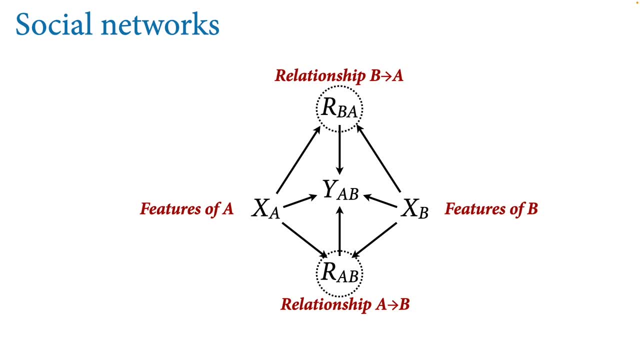 like to stratify by when we try to estimate the influence of, or merely estimate the social network And the thing about these features which I've marked here as X on both sides, X sub A- features of individual A and X sub B- features of individual B. 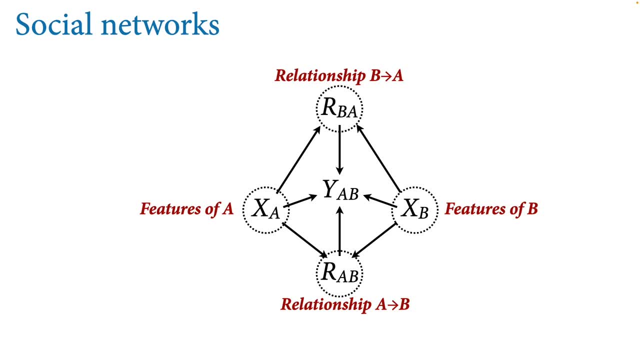 is. they're also often unobservable. They could be things like personality. We don't even know what to measure. How do you make progress in a case like this, where the only thing that's been observed is behavior, but we're imagining a bunch of latent variables that are actually causally driving all of that behavior? 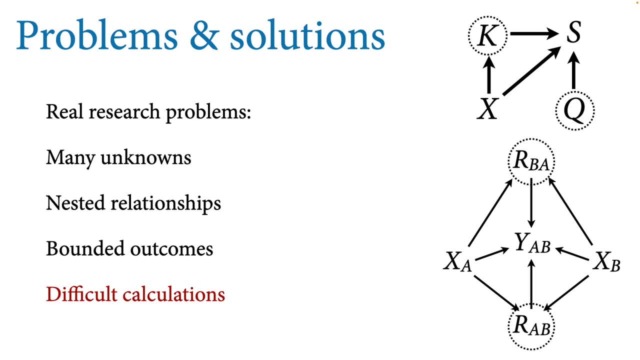 Well, you can make progress. All of these areas of statistics are very well developed. They depend upon models that have a number of inconvenient features. First, they have many, many unknowns or many parameters, sometimes more parameters than observations, And some of you will have been told that it is impossible to estimate more unknowns. 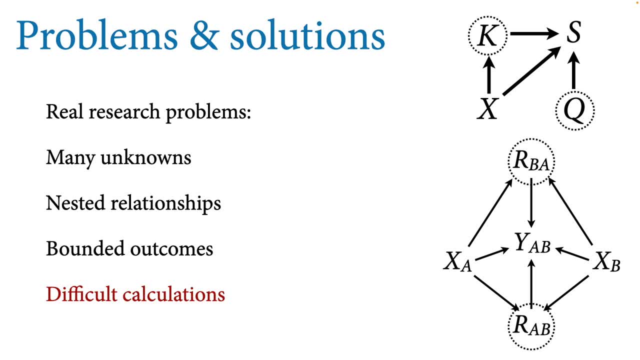 than you have observations. but it's not impossible. It's very possible and we will do it. In fact, we have to do it to solve important scientific problems. Second, there are nested relationships among these unknowns, All the models we've seen so far in this course. 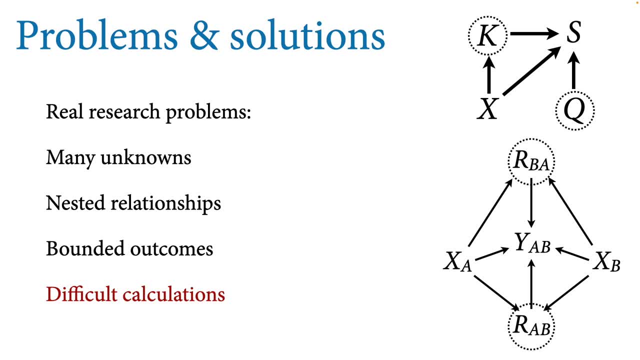 the unknowns interact in a purely additive way, But there can be multiplicative or nested relationships among unknowns and that makes the calculation of posterior distributions more challenging. There are often bounded outcomes As well in realistic science problems. so far I've tried to be nice by avoiding 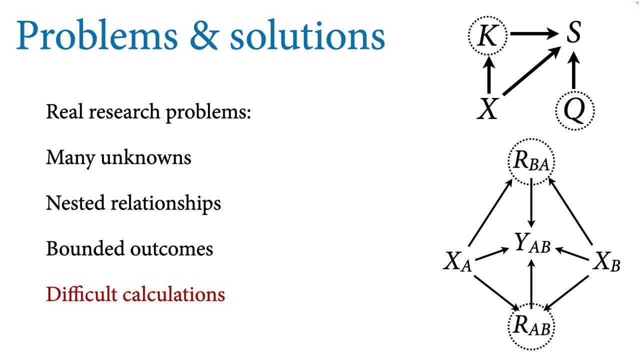 thinking about boundaries on observed variables. Everything's been nice, smooth, Gaussian outcomes. But soon we're going to start dealing with count variables, and those are bounded. A count can't go below zero. All of this mounts up to make the calculations quite difficult. 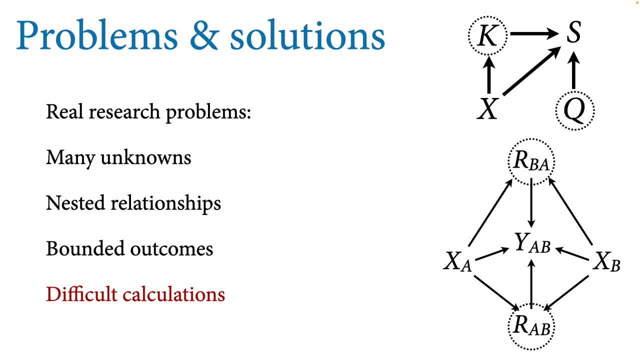 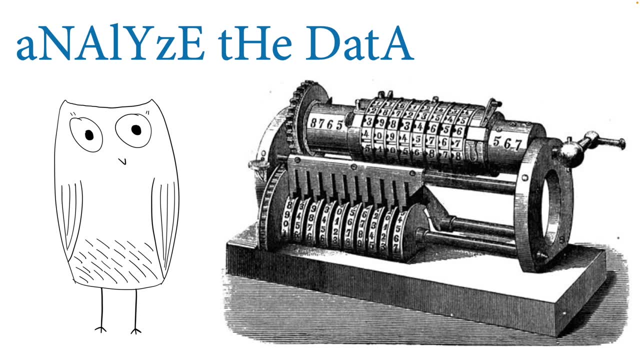 and so we're going to need a more general framework for computing posterior distributions, And luckily it already exists and is likely already on your computer. Yeah, so when we reach the stage in my drawing-the-owl workflow, there's this analyze-the-data stage, and that's always left a bit vague. 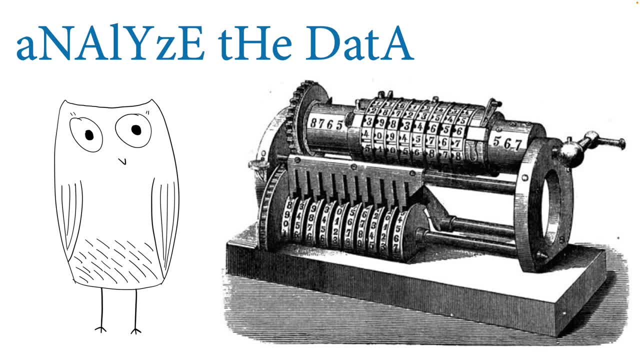 I'm telling you we're going to draw every step in the owl, but then I've blackboxed what really goes on in computing, the posterior distribution. So in this lecture I want to give you an introduction to what is going on inside the box. 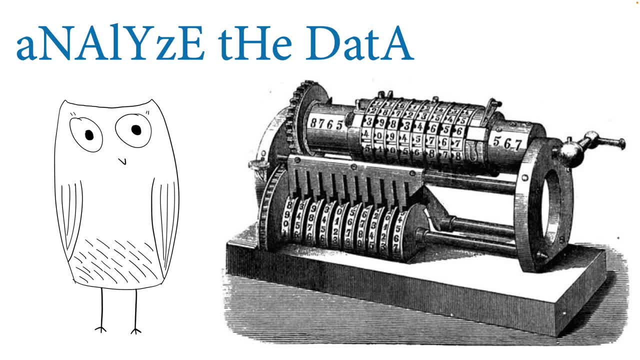 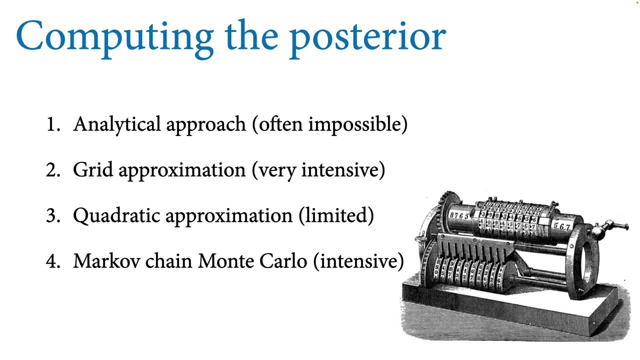 when the posterior distribution is calculated for the more advanced models we're going to be using going forward, which means I'm going to introduce you to Markov chain Monte Carlo. So at the very beginning of the course, in the first week, when I computed the posterior distribution, 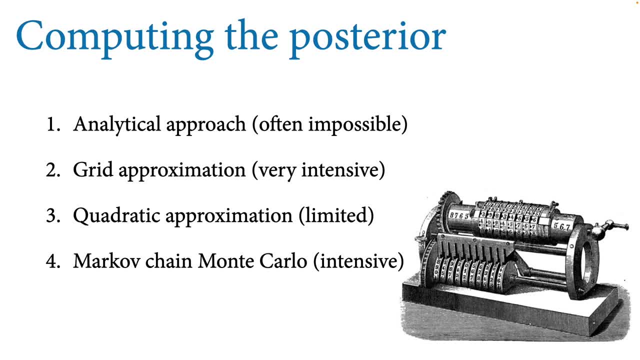 did the Bayesian updating? we did it analytically. We could just count paths through the garden of working data and in those cases, the simple cases from week one, we could actually do everything analytically because the integrals are easy to do. 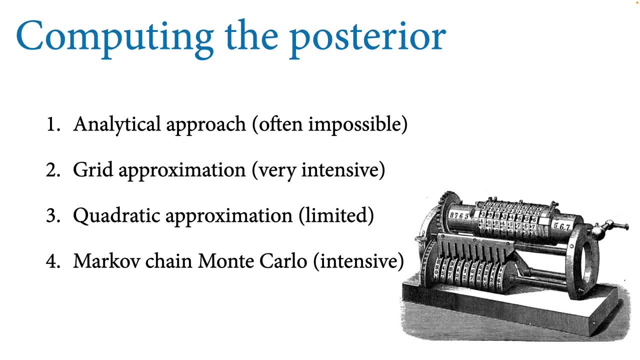 and you can get a closed-form, little function for the posterior distribution. I also showed you in week one this trick called grid approximation, which is easy to do. It's easier to understand for a lot of people, where you divide up a continuous space of unknowns into a grid of any density that you like. 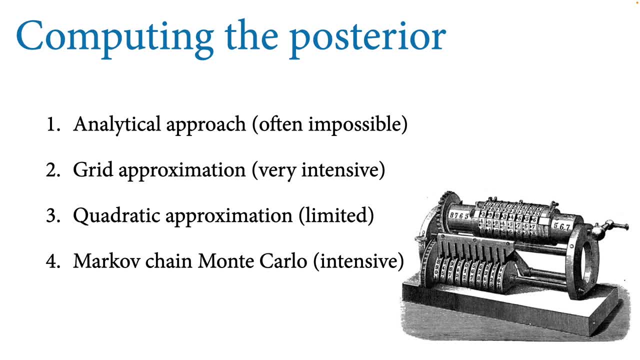 and then just count paths through the garden, and you can always compute posterior distributions this way as well. It's just that it's very intensive. So the first approach, the analytical approach, is only possible in the simplest sorts of problems, and usually you have to structure them in awkward ways to even make it possible in that case. 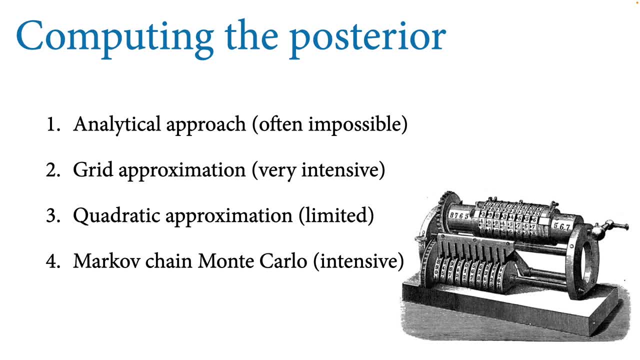 The grid approximation process is, in principle, always used, always, always possible, but it's in practice hardly ever useful because it just takes too much calculation time. As the number of unknowns grows, the dimensionality of the grid grows. 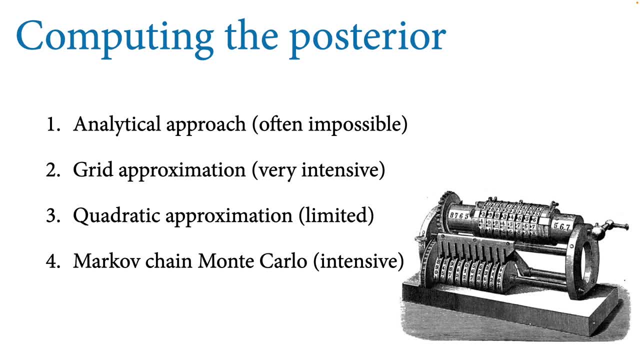 and it's just not practical in terms of computing time. The approach we've been using up until this week is called quadratic approximation or Laplace approximation- you may have heard it called. This is an extremely useful technique and I don't have anything against it. 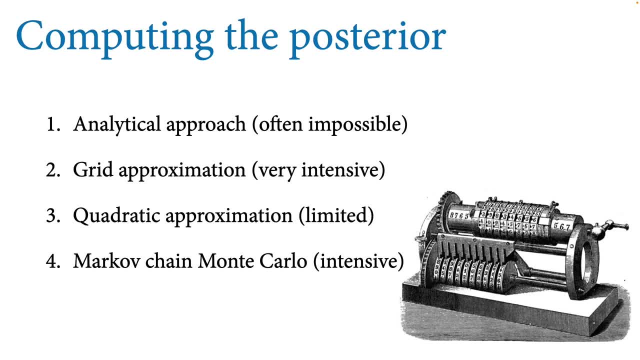 There's a very similar uh algorithm that's used in non-Bayesian statistics: uh, maximum likelihood, uh, which is basically the same thing, although people won't like me saying that, uh, but it's the same algorithm. 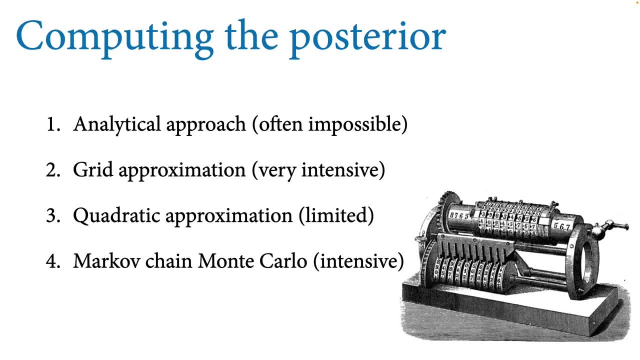 and I even use the same engine. This is a great technique, but it's it. it's limited in the kinds of problems it can do well, and there are lots of important posterior distributions that are not approximately multivariate Gaussian, and so we want something more general that doesn't make strong assumptions about the 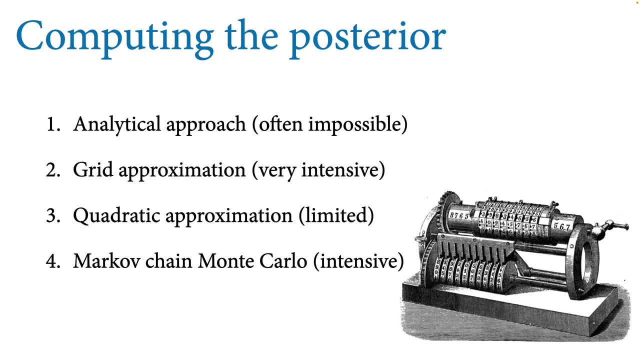 uh, approximate shape of the posterior distribution. And so we come to this technique, which is the workhorse of um, of modern desktop statistics: Markov Chain, Monte Carlo. It's also intensive, uh, but you can use it on a wide range of arbitrarily. 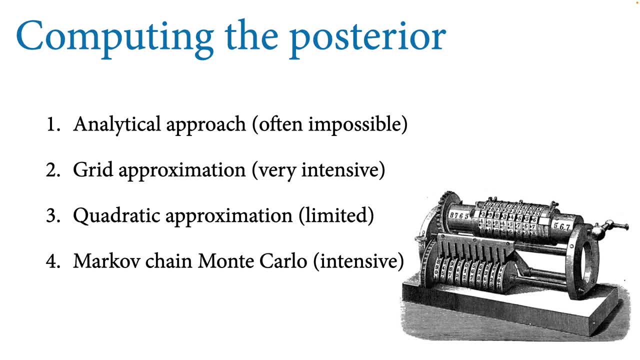 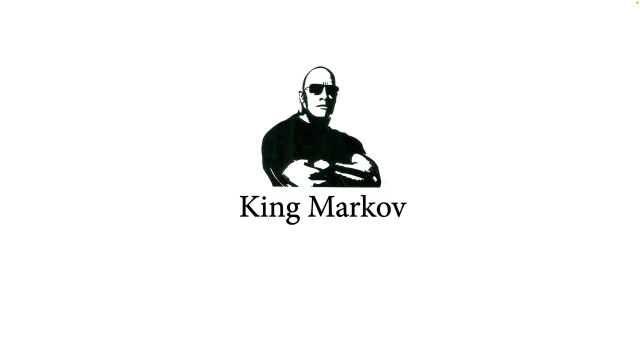 uh, scientifically complex and realistic problems. uh, and increasingly it scales really well too. So, for example, in my own work, um, I've used this technique on models that have tens of thousands of parameters, with no problem at all To introduce Markov Chain, Monte Carlo to you. 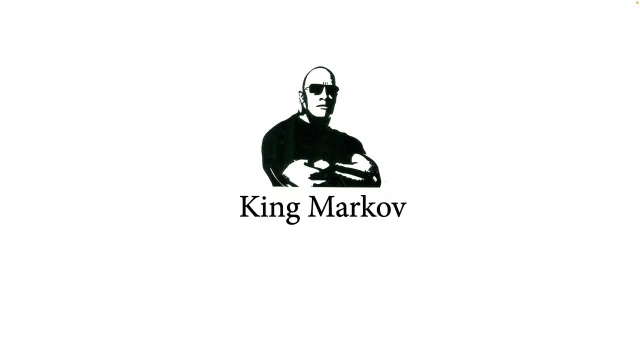 I want to tell you uh a parable. uh, leave the mathematics uh aside for a moment. So the the parable goes like this: Uh, suppose there's some uh uh, Polynesian kingdom. 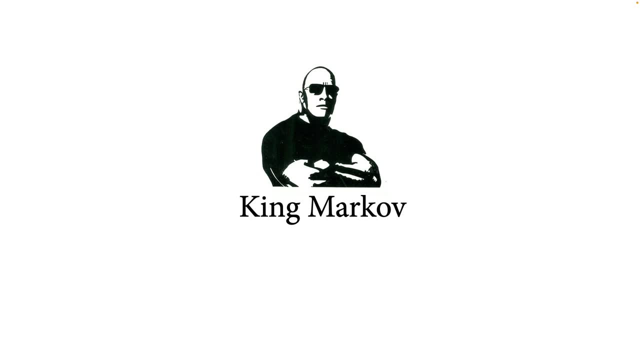 and it has a, uh, benign monarch named King Markov seen here showing his smoldering intensity. And King Markov, King Markov is benign, Uh, he loves his people and his contract with them is that, uh, he will visit them. 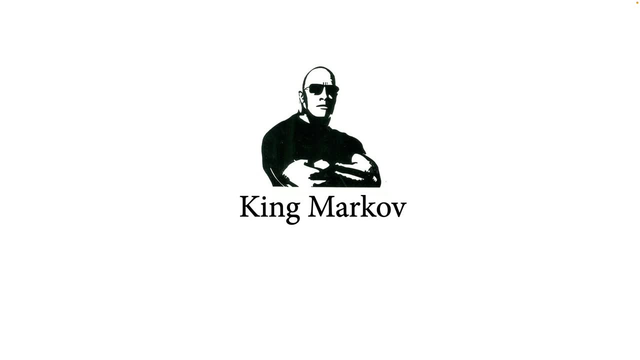 um, so that they can uh meet their monarch from time to time and feel watched over. There are a number of islands in King Markov's kingdom, which is called the Metropolis Archipelago. I show you one, two. 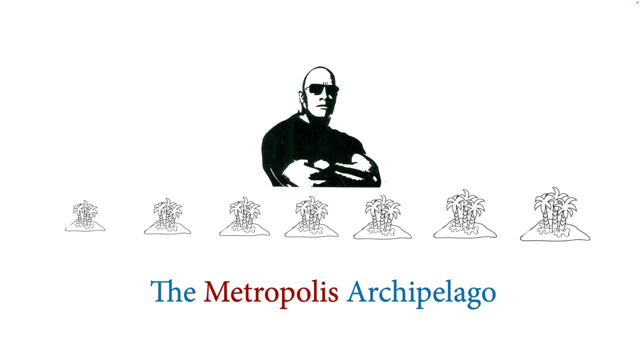 three, four, five, six, seven islands here And his agreement is that he will tour these islands um uh and spend time on them in proportion to their population sizes. So the larger islands have more people and he will visit those islands more often. 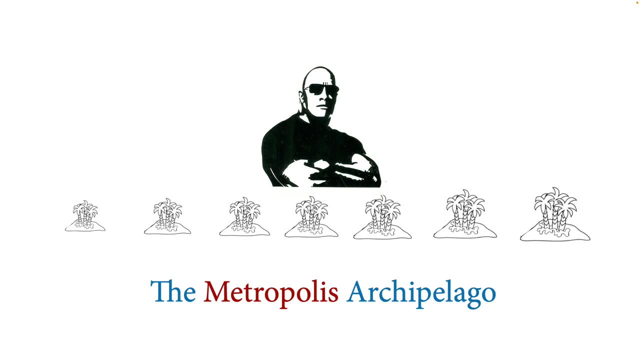 uh, wave it, wave it. more people kiss more babies and so on. And the smaller islands he will visit, um uh, much less often, But always in proportion to the number of people there. So this is his contract and this is what he has agreed to do. 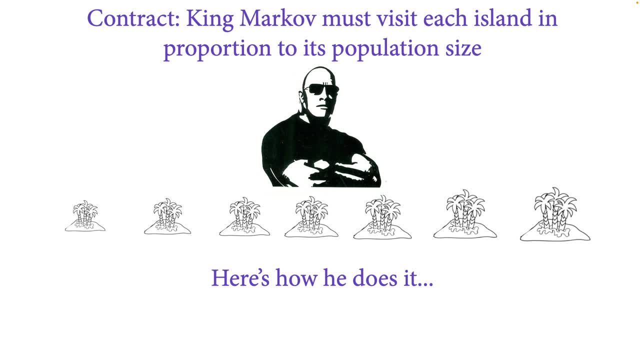 And he's an honest man and he wants to do it, Uh, but he's also, um uh, not interested in careful record keeping or having a calendar. He likes to live in the moment, And so his demand he makes to his advisors is that 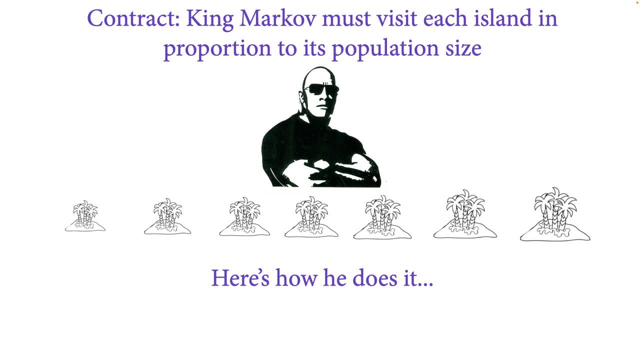 uh, he doesn't want to have some calendar about which island he's going to be in at any time. He wants to have some simple rule of thumb. he can use um on any given day to decide whether he stays on the same island or moves to another. 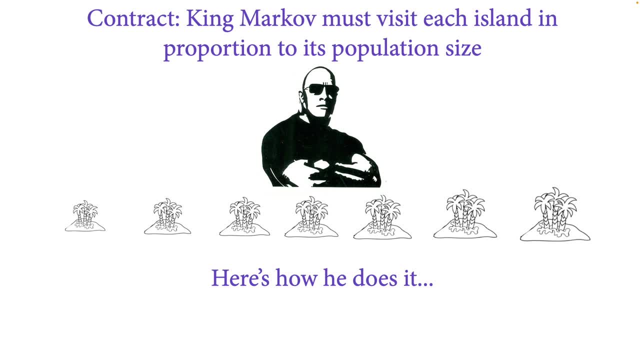 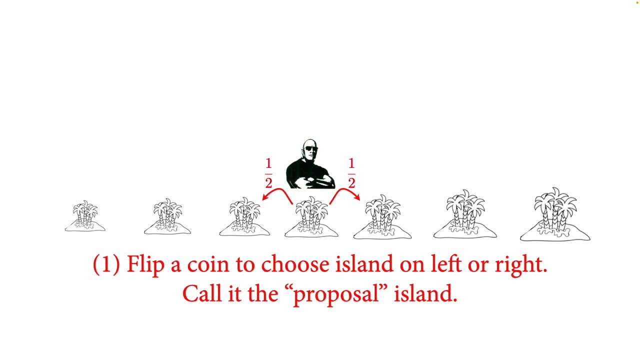 Uh, and this algorithm? there is an algorithm, it turns out, that will let him do that and still keep his promise. It has a series of steps, Uh. so first he's uh needs to flip a coin or some other. 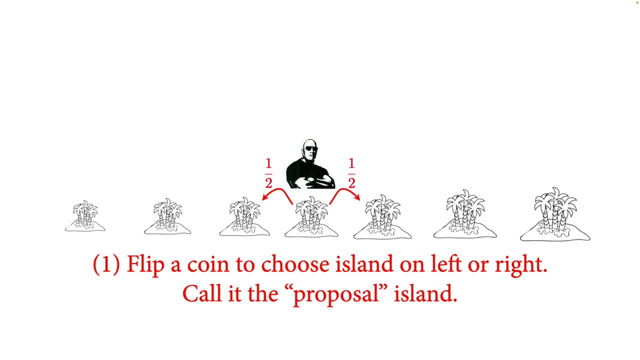 uh randomization device to choose an island, uh left or right. Remember, this is an archipelago, so the islands are in an order. Um, this gives him a uh proposal island, an island, that is, the coin has proposed. 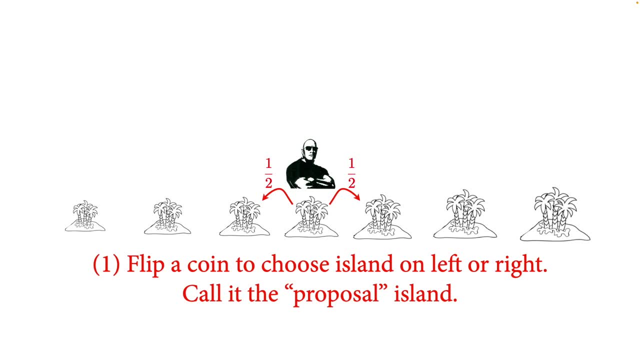 that he moved to Um and since it's a fair coin, uh, there's a half chance that he will go left and a half chance that he will go right. That's step one. So let's say it chose to go to the right. 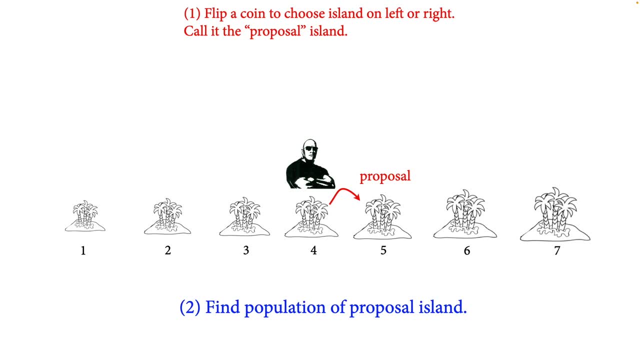 Now we have a proposal island. uh, he say he's on island four. The proposal is to move to island five. To decide whether he accepts the proposal, he needs to find the population of the proposal island and he can ask someone or he can send an advisor across to island five to do that. 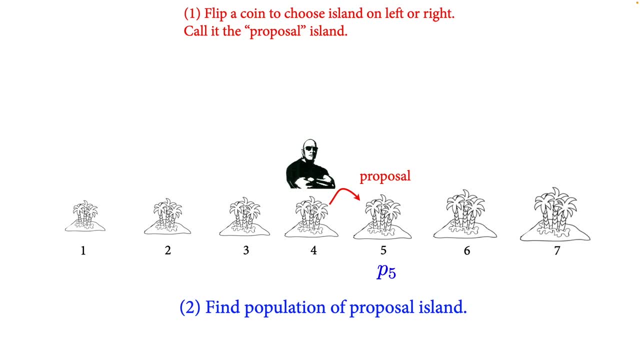 Um, and let's call that number p sub five, the population uh of the proposal, island, island five. in this case He's on island four, so he needs the same information for island four and that's easy to get as well. 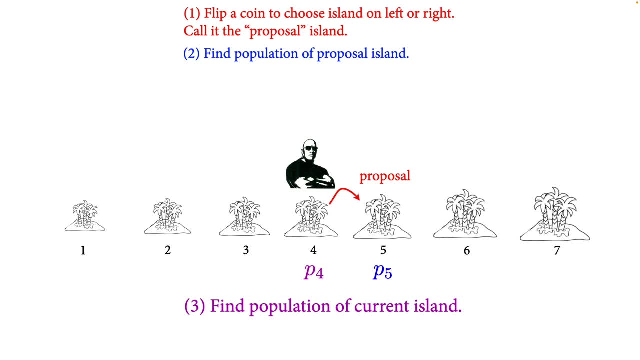 Uh, let's call that p sub four, the population of island four, the island he's currently on, And then the rule is he moves to the proposal island with probability um p five divided by p four, That is the. 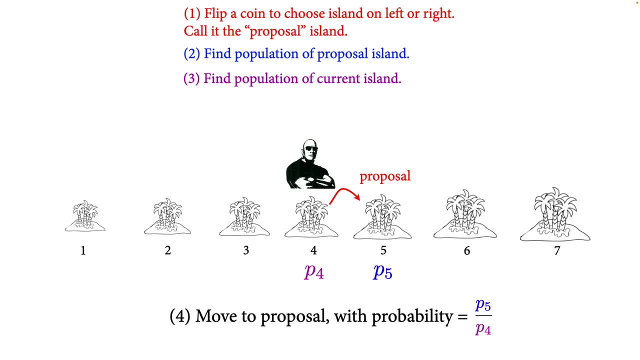 the- the population of the proposal island divided by the population- uh- the population of the proposal island divided by the population- uh- the population of the current island he's on And he needs something like a spinner, uh, or a bag with. 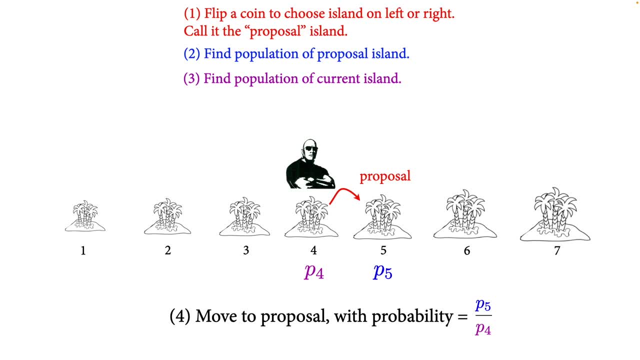 uh, rocks in it or something like that in order to um uh move with this probability. But there are lots of of natural randomization devices, like dice, that can do this. This seems wild, I know. uh, uh. 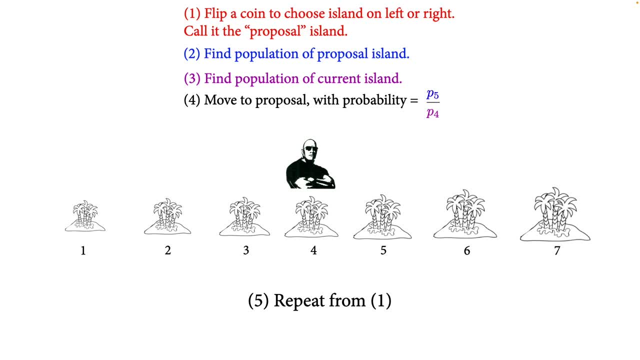 but it works. Uh and uh. step five is, of course, to just repeat it every day, And in the long run, if he follows this algorithm faithfully, he will visit all the islands and he will visit them in proportion to their population sizes. 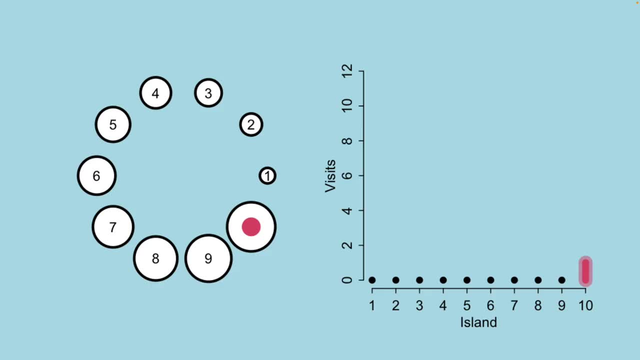 but only in the long run. Let me show you what this looks like in animation. So what I? what you're seeing on your screen here on the left is the- uh- metropolis archipelago, but I made it into a ring. 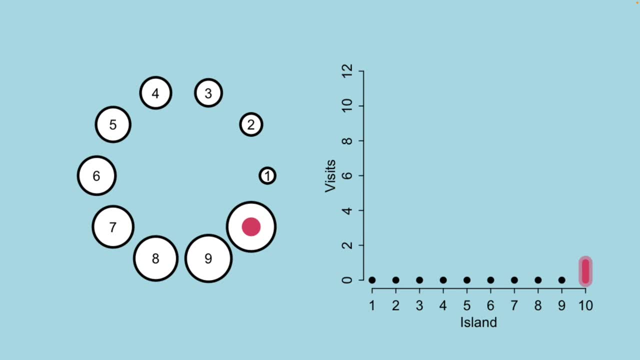 So it's easier to think about looping around. so that, uh, the biggest island, which which we're going to start the simulation on there is 10.. It's got the red dot on it. um, has got an island in each side of it as well. 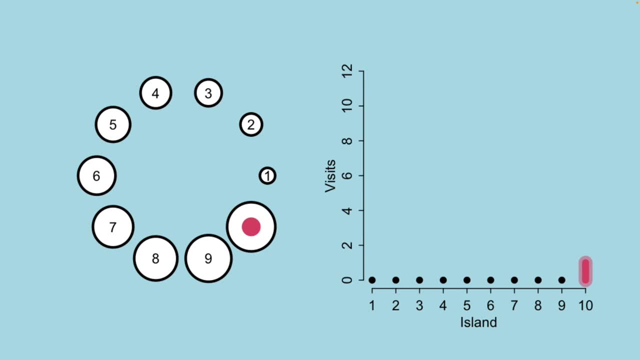 And uh, you'll see that, um, some of the islands are bigger than others. And, uh, from one one being the smallest and 10 being the largest on the right, we're going to just kind of a histogram of the number of visits that. 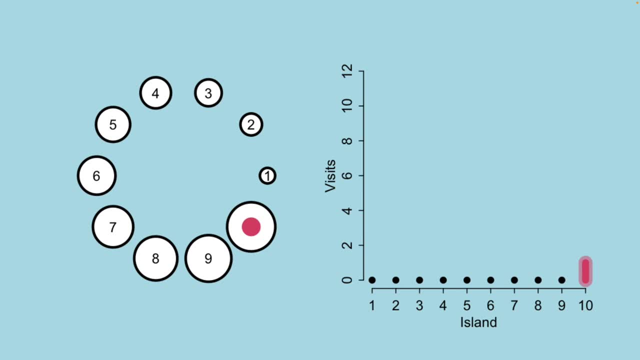 uh. King Markov visits and shares his smoldering intensity with the citizens. So start the animation and you can see what happens. They jumps around, goes back and forth between islands, sometimes makes long tours, and we're starting to build up. 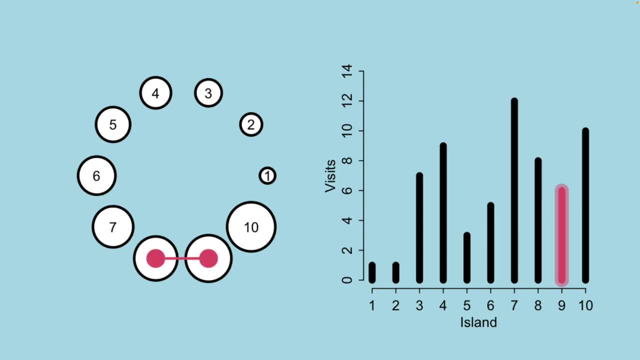 The counts doesn't look very proportional yet, Uh, but remember, I only promised in the long run there's a mathematical proof that this works. but in any particular simulation it can take you a while to reach that expectation. but you see, 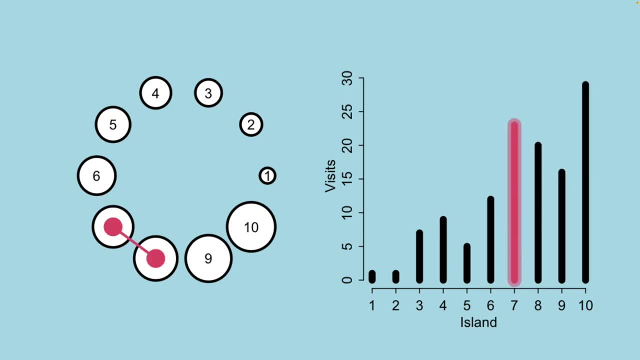 it's already starting to take shape, Um, and what happens is he tends to stay on bigger islands, um, and tends to move from smaller islands to larger islands, Uh, and in the long run, then ends up visiting in proportion. So I can do. 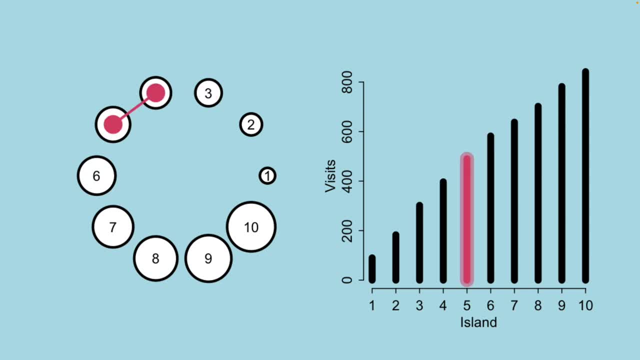 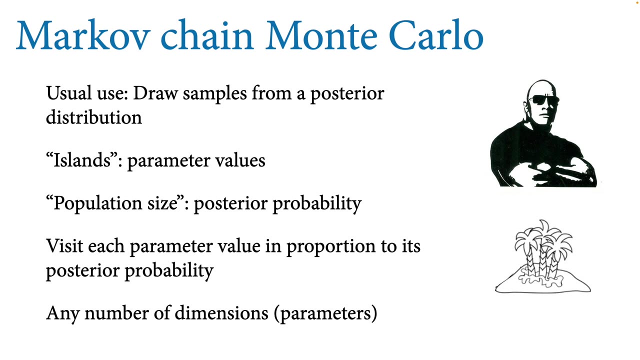 here's the what it looks like in the very long run and you can see after running it for thousands of of days. um, we get an almost perfect proportional representation and the citizens feel cared for. Okay, Obviously, the Metropolis Archipelago doesn't exist and King Markov doesn't exist outside the realm of fiction. 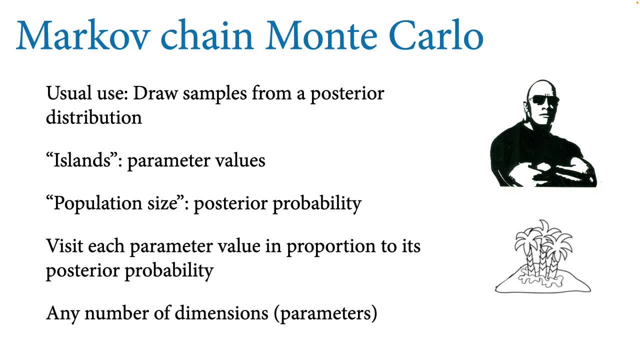 Uh, what you're seeing is the the oldest and simplest Markov chain Monte Carlo algorithm. That's called the Metropolis algorithm And, uh, this algorithm is used a lot. Uh, it has been used a lot for decades Now. it's usual use is to draw samples from posterior distribution. 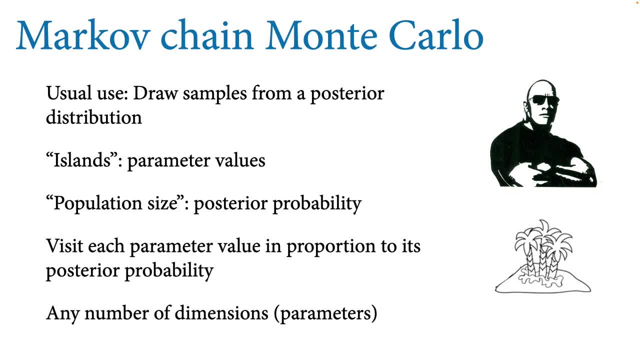 but it can be used for lots of other things to any uh. uh, it's used to take integrals, It's used to do calculus, uh, without having to actually do the calculus. Um, your computer, sort of like tricking your computer into doing difficult calculus for you. 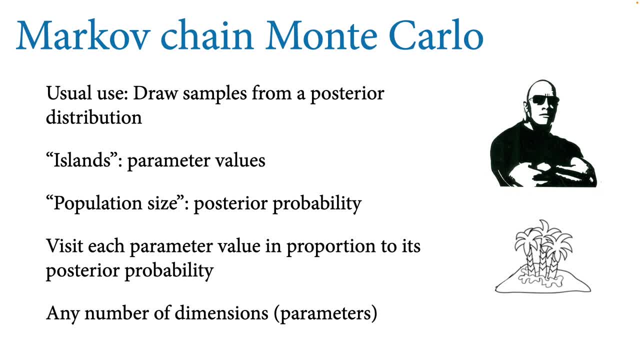 Uh- the islands um metaphorically- are unknowns or parameter values. They are the candidate explanations of the observations that that define the dimensions of the posterior distribution, the parameters in your models, the uh population size In this example. 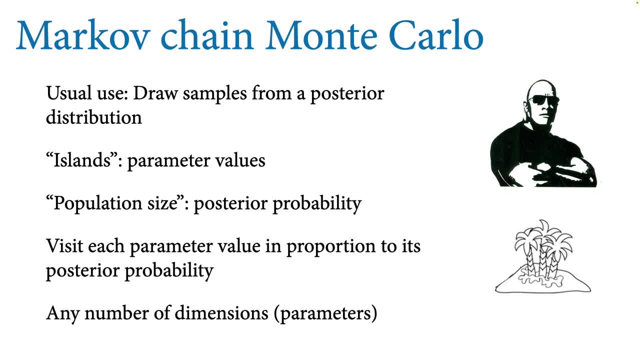 is posterior probability. Uh, what we want them, the, uh the Metropolis algorithm- to do is to visit parameter values more often when they have higher posterior probability, And that means we'll get more samples from them, where the samples mean days visited. 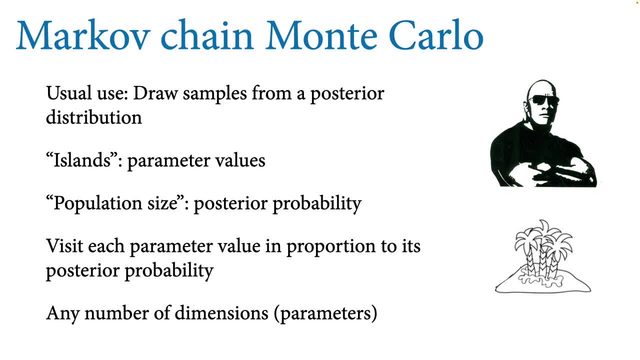 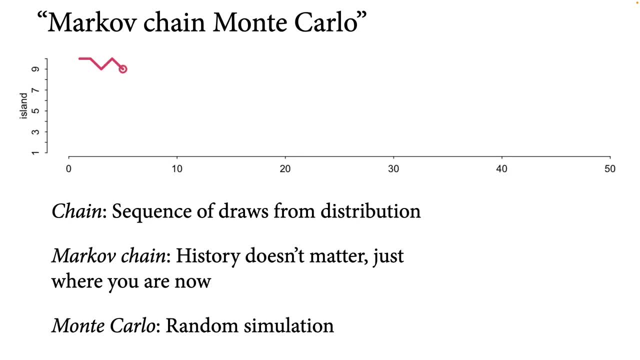 Um so, uh, and this actually works, and it can work for a very larger numbers of dimensions of parameters as well, if you have enough computer time. Uh, so this is the way we usually view these things called Markov chains. It'll give you. 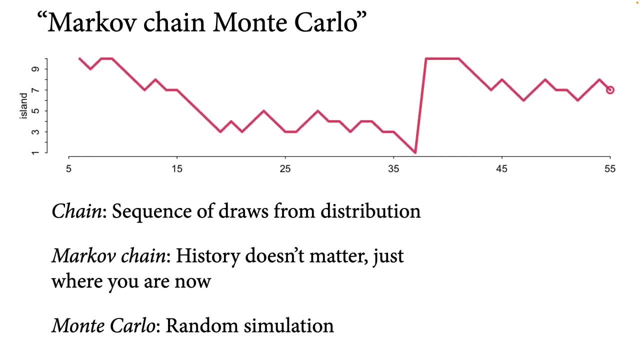 you an idea why we call them chains? Chain just means a sequence of draws from some distribution, And what I'm doing here on the screen is animating it. where the vertical axis is the, the island visited at, the position or the parameter value of King Markov. 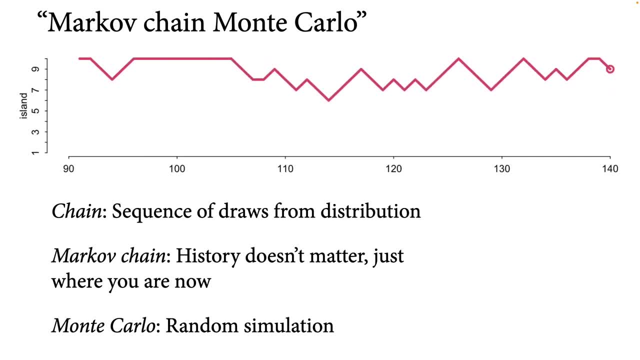 And the horizontal is the day, And you see, he wanders around from island to island but he collects a bunch of island samples in this And this is the Markov chain. It's the chain of these random samples, his position on any given day. 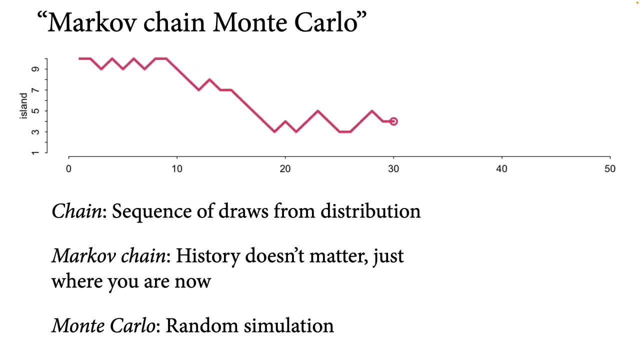 Um, Markov chains have a particular property. There are lots of of sequences of draws, You can call it chain, and Markov chain has an interesting property. and that the history doesn't matter. All that matters for the probability of what happens next is where you are right now. 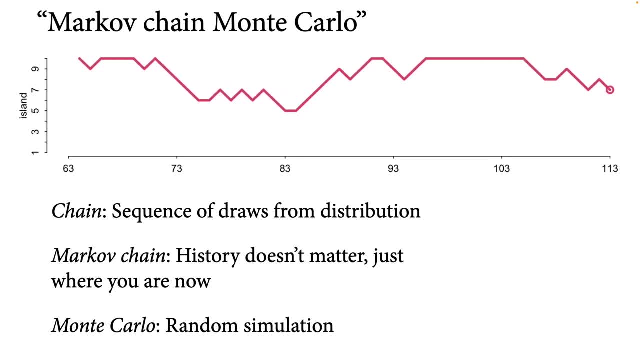 It doesn't matter what happened 10,, 10 days ago- And Monte Carlo is just a cute name that some mathematician decided that it means. random simulation has to do with a particular city where people gamble a lot. Okay, so if we scrunch up this Markov chain, 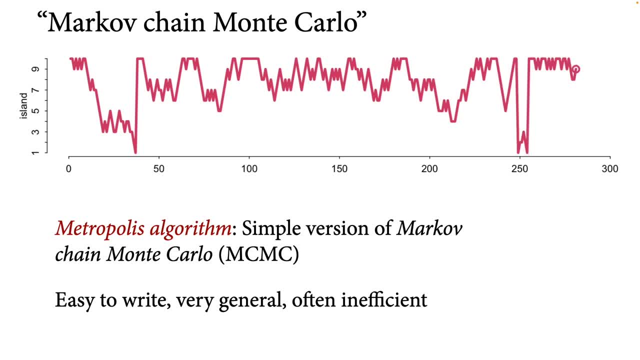 you can see it a little better how it makes a sample over time. And if you take all the values that make up that red zigzaggy line and stack them up as a histogram, you'll have a posterior distribution. And if you let it run long enough, 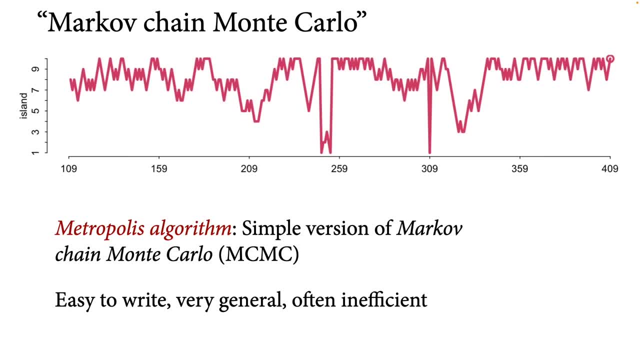 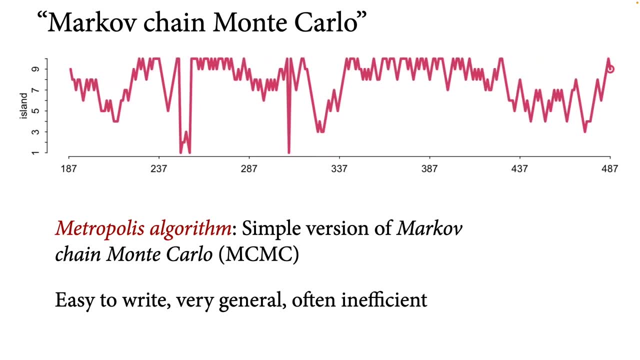 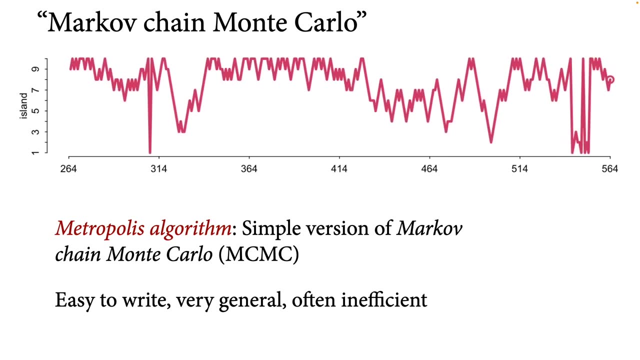 you'll have an excellent, arbitrarily good estimate of the shape of the posterior distribution, And this is the so-called Metropolis algorithm, named after a man, Nick Metropolis, who headed a group that was the first to use this in a scientific application. It's very easy to write. 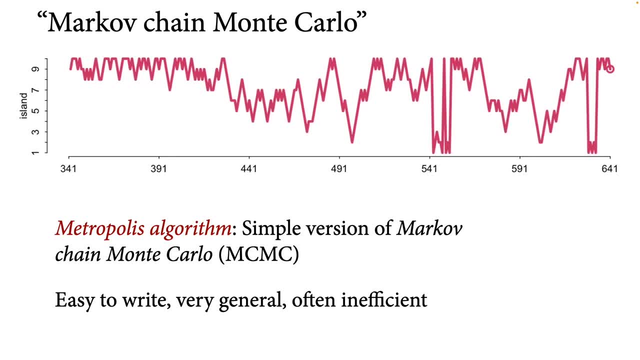 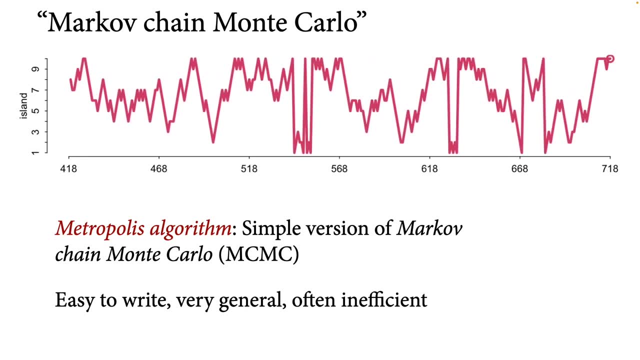 but it's often very inefficient And it's not used so much these days. We're not going to use the Metropolis algorithm, but it inspired all the other methods And so and it's easiest to understand, So it's worth knowing a little bit about. 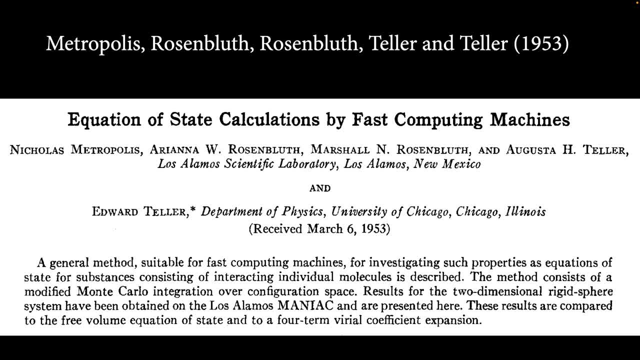 I want to say not so much about exactly how the Metropolis algorithm is programmed, but more about who programmed it first, because I think the history of this is really interesting. The Metropolis algorithm is now something you can teach to undergraduates, and you can 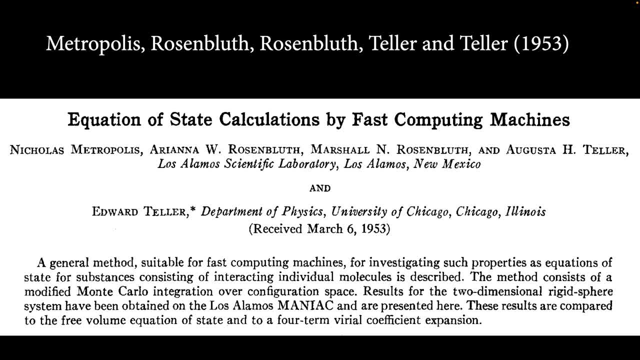 you can do it in a few lines of code- Actually it's so simple, But when it was first used, computers were much more primitive back then, And of course no one knew how to do this, And so it's worth saying a little bit about the development of that. 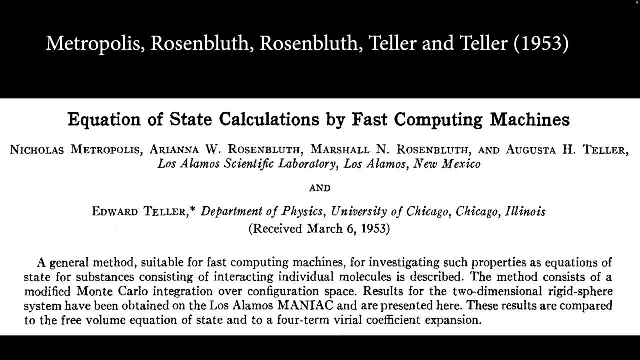 So it. this is the paper that's usually recognized as launching the Markov chain Monte Carlo computing revolution, This paper with this very awful title: equation of state calculations by fast computing machines. fast computing machines for the time. This was 1953, when computers took up a whole rooms and 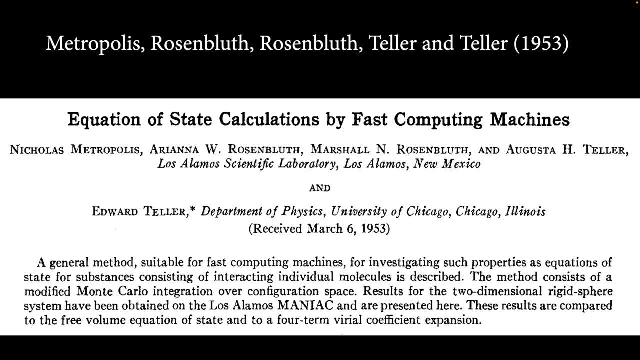 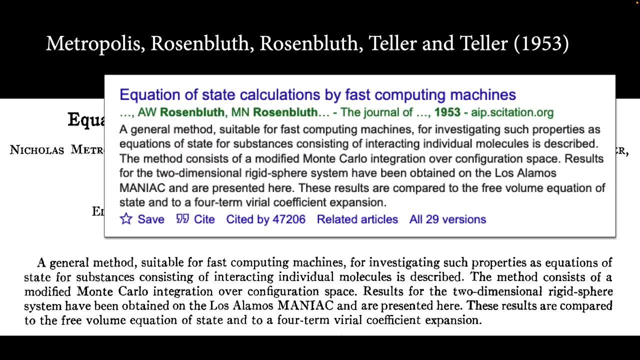 and this is the paper Metropolis, Rosen booth, Rosenbluth, Teller and Teller that gives the Metropolis algorithm its name. This paper has been cited last time. I checked over 47,000 times It's. it's kind of a one of those papers that starts a whole field. 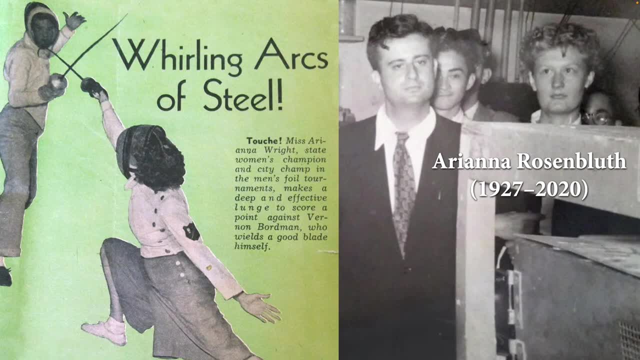 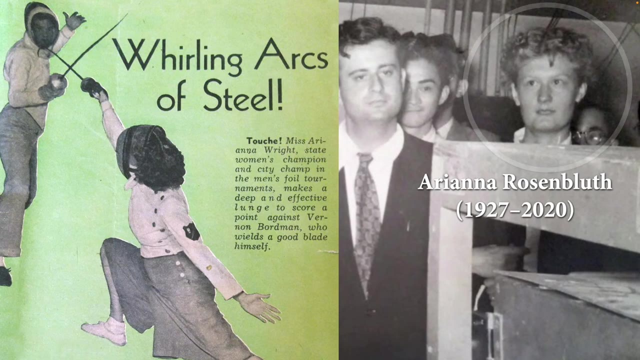 The person who really did almost all the programming is this person in the upper right here, Ariana Rosenbluth. should also the fencer on the left when she was still had the last name right And Rosenbluth contribution was to take the mathematical derivations and make a machine do them. 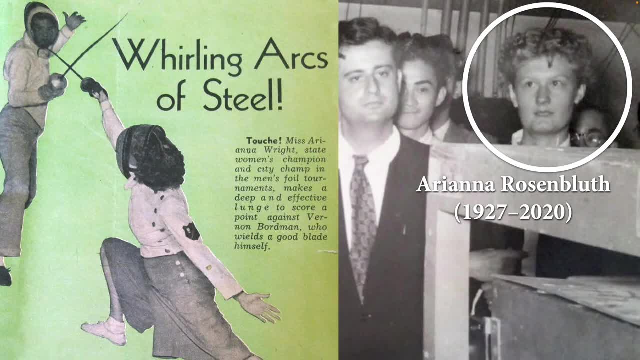 And anybody who's ever tried to do mathematics with a, with a computer, knows that there's a whole bunch of other stuff that comes into play. So there's a great achievement when nobody knew if this was going to work at all. to actually take the mathematical theory: 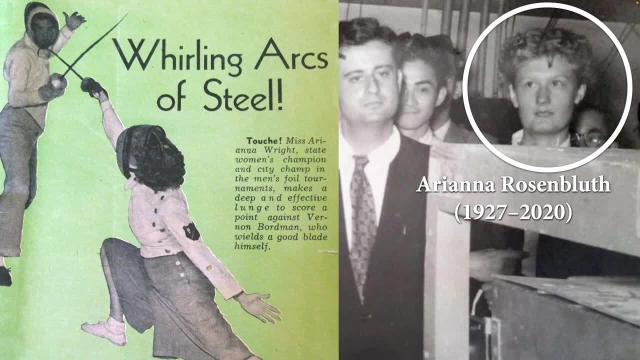 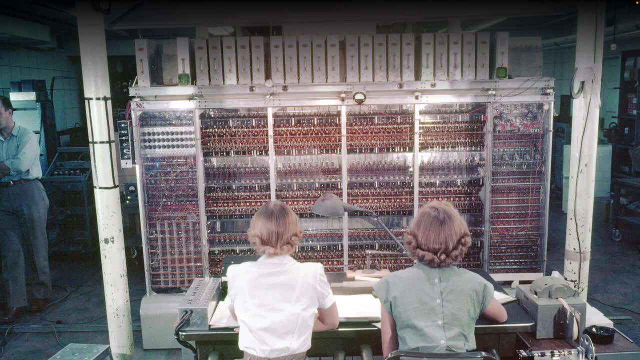 and make it work in the machine in silicon. This is the machine that she did it on. This is machine is called maniac. Maniac took up a whole room. This thing had vacuum tubes and a whole fleet of people constantly replacing them. 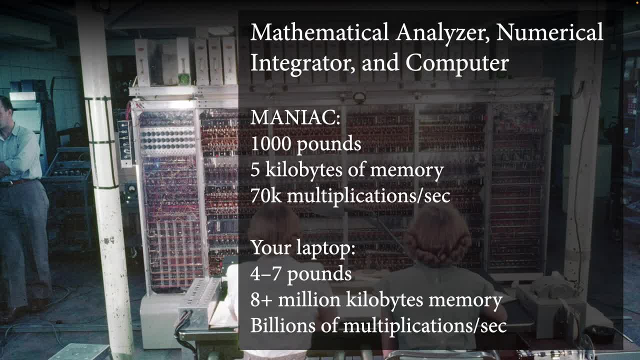 One of those kind of computers, Yeah, from the 50s, and maniac, which was one of the fastest computers in the world at the time, stands for mathematical analyzer, numerical integrator and computer. You can guess they worked really hard on that acronym, and maniac weighed a thousand pounds. 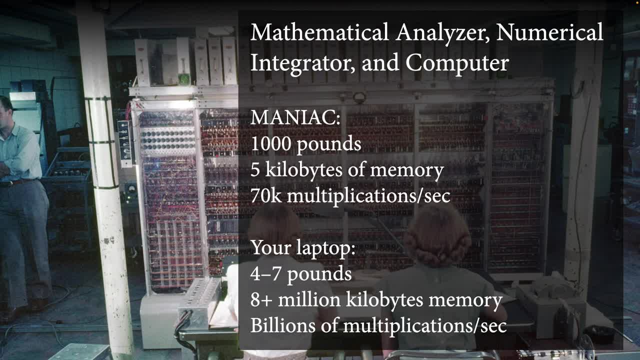 It only had five kilobytes of memory and it could do 70,000 multiplications per second. That is a lot. I don't think I can do 70,000.. Multiplications per second, at least not consciously. but if you compare that to a bargain laptop that you might own, 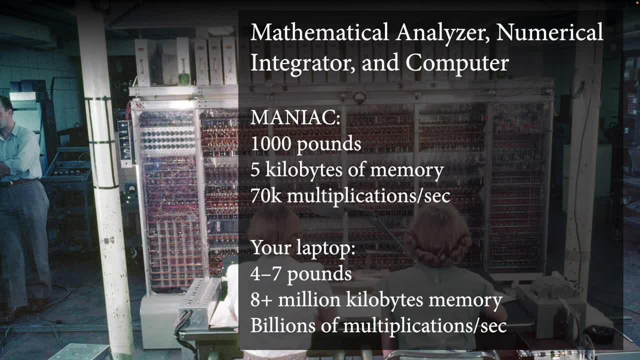 which is 47 pounds. it'll have more than 8 million kilobytes of memory and could do billions of multiplications per second. No problem, but they made it. They made it work on this vacuum to monster, These days, Markov chain. 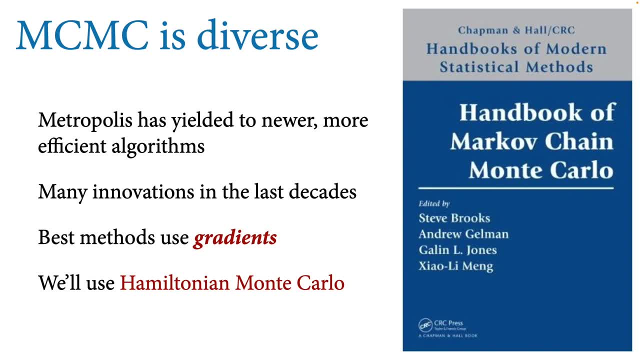 Monte Carlo is a diverse range of algorithms, is not just a metropolis algorithm. People have worked really hard and the last couple decades Especially, things have gotten a lot better because there are many more people working on it and also computers are faster- The best methods these days- and are ones that use something called gradients. 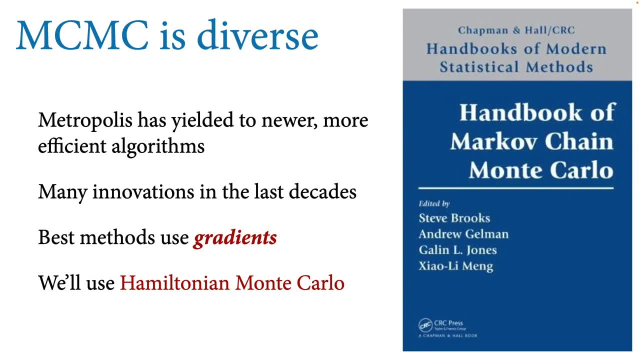 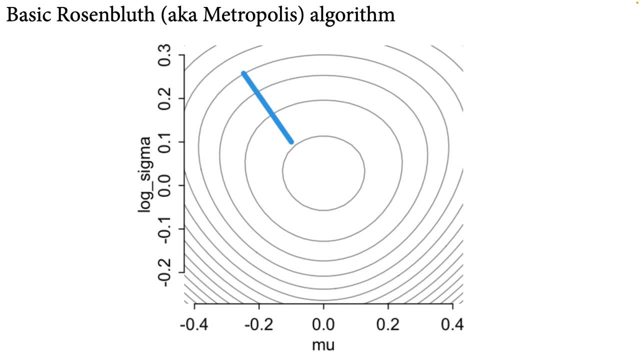 I'll explain them what that is as we get into the lecture. and in particular, we're going to use a gradient based method called Hamiltonian Monte Carlo. So to understand what Hamiltonian Monte Carlo does, it'll it'll help to understand the metropolis algorithm a little bit more. and let's take an 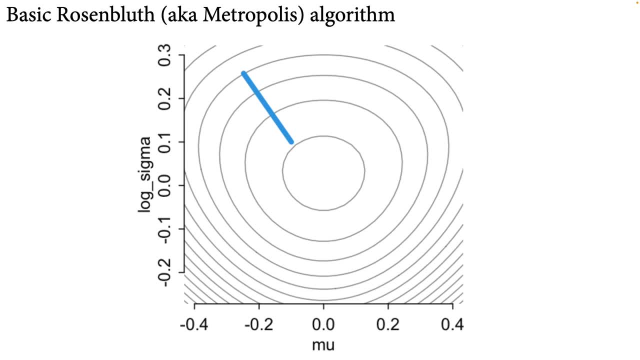 Animated view of it. So what I'm going to show you is the basic Rosenbluth algorithm, better known as the metropolis algorithm, but this is this is the fetch I'm trying to make happen right now. Let's see if we can get people to start calling it the Rosenbluth algorithm instead, because Nick Metropolis didn't write any code. 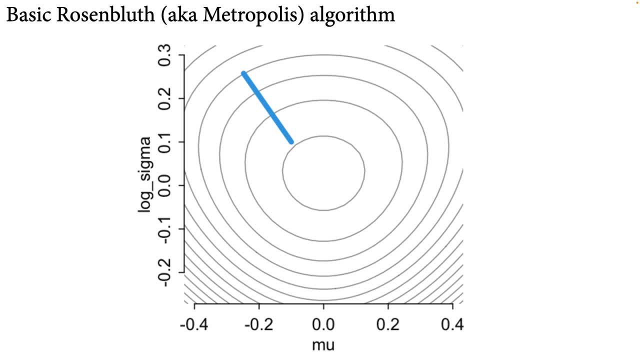 And the way the Rosenbluth algorithm works is well, as I explained it with King Markov. you make proposals, You have a position in parameter space, So in two dimensions, like on the slide here, we've got a mean mu And then some Sigma value, and I'm here. 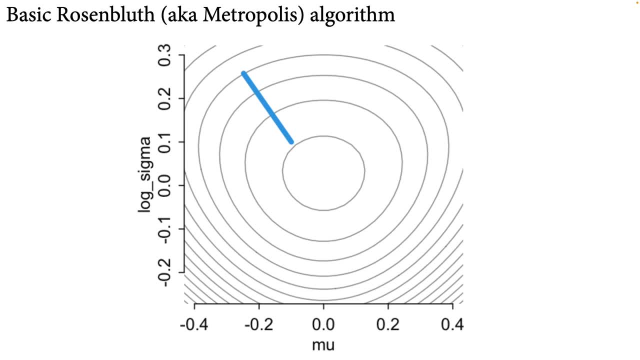 I'm drawing it on log Sigma, So there's no boundaries, is a smooth space And what we have, a position, and then we make a proposal and the blue line here is a jump from starting position to a proposed position And you'll see the. the blue lines indicate proposals. 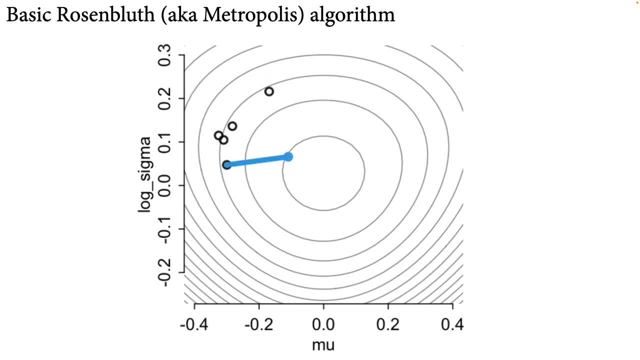 And when they're rejected there's a red dot and we go back to where we were and we make a new proposal. But when they're accepted, the individual crawls along the proposal line and moves and these circles that are left behind, There's a trail of samples through the posterior distribution and in the long run, 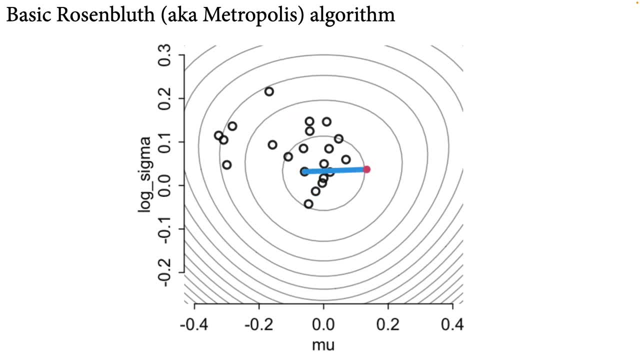 These samples are combinations of parameter values which are drawn from the actual posterior distribution that we want to sample from. that's great about an algorithm Like this is that we don't know mathematically the distribution. We've defined its constraints and we have some data that that logically decides what it must be. 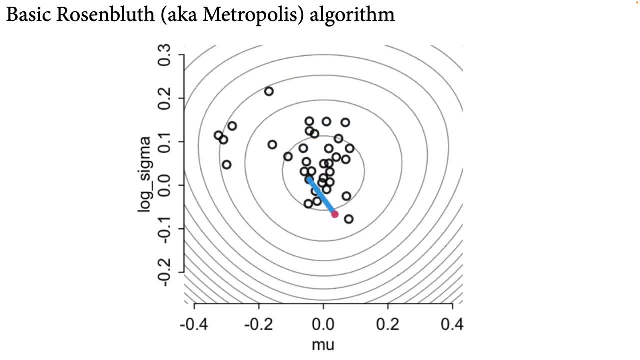 but we can't do the integral calculus. Nobody can that can tell us what the distribution is mathematically, but we can still sample from it using an algorithm like this. This is a huge accomplishment, and it's incredibly non-obvious that we would use random numbers to do something like this. 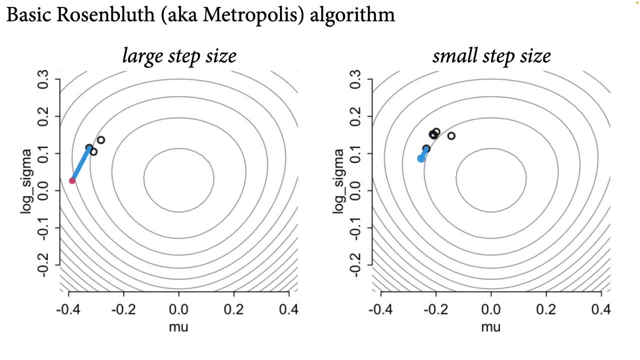 Okay, the Rosenbluth algorithm has a bunch of tunable properties that can make it more or less efficient, And when you try to use it in practice, usually you have to worry about these things. So I'm going to show you one particular thing about it. 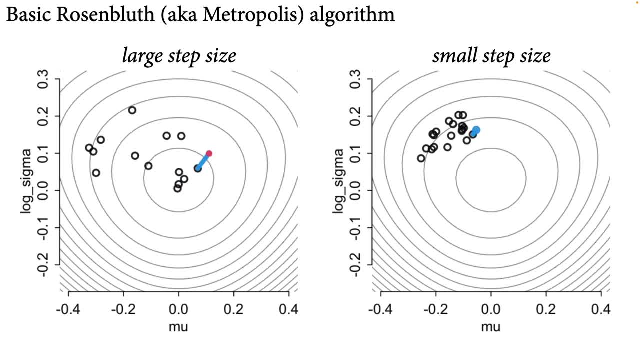 It's a trade-off, this thing called the step size, and you can think of this as the distribution of proposal Lengths: how far away from your current position you're willing to move. and when it's large, like on the left, you explore the posterior distribution faster because the possible jumps are bigger. 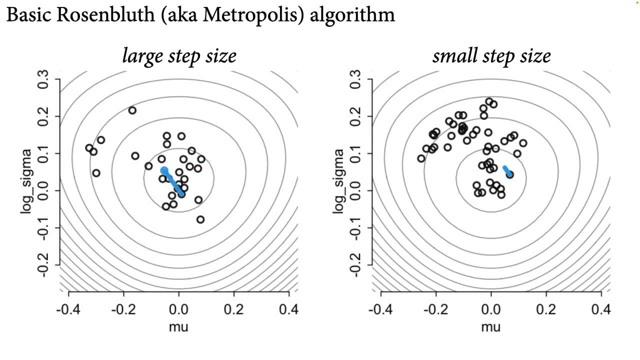 but many, many more of your proposals are rejected because you will make bad proposals into low probability spaces on the edge of the posterior distribution. And that's what you see on the left. It's. it tends to get stuck in an area and make repeated rejections. 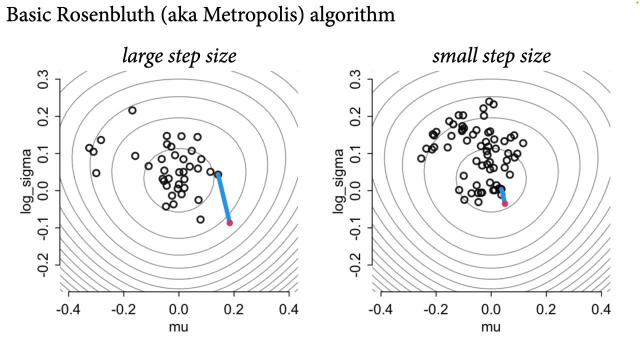 Those little red Dots over and over again before it moves and then again, and this wastes a lot of computer time, but you can traverse a big posterior distribution more quickly with larger steps. in contrast, on the right We have the same distribution, the same algorithm. 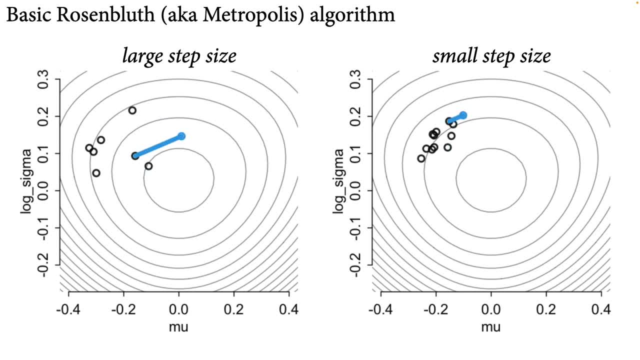 but now the step size is smaller, So the maximum size of the posterior distribution of the proposal distance is much, much smaller And in this case proposals are much more likely to be accepted, because proposals aren't into into some wacky neighborhood with very low probability. 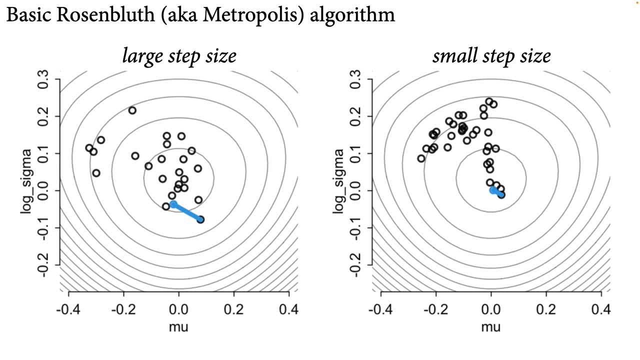 but it takes you a very long time to explore anything because you're taking a bunch of samples that are right next to one another and contain essentially the same information about the distribution, And so the total to see the total shape of the distribution takes much longer this way. 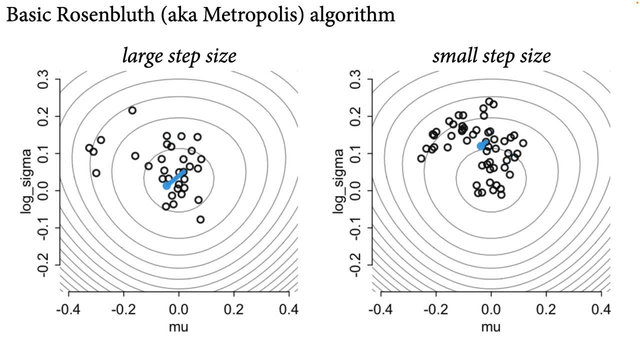 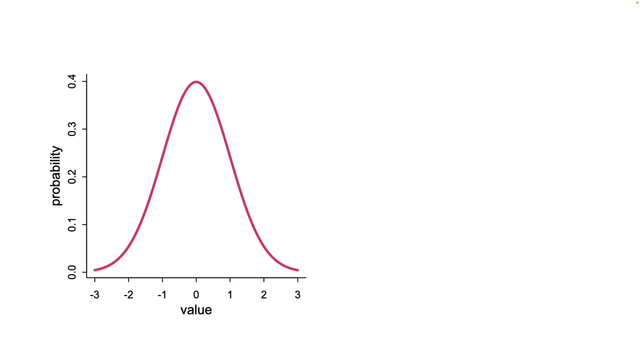 This fundamental trade-off cannot be avoided in the Metropolis algorithm, which is built into. how its logic works Doesn't make it wrong, It just makes it very inefficient, sometimes So inefficient that it's it's not practical to use. Okay, Now we're going to talk about gradients and where they come in. 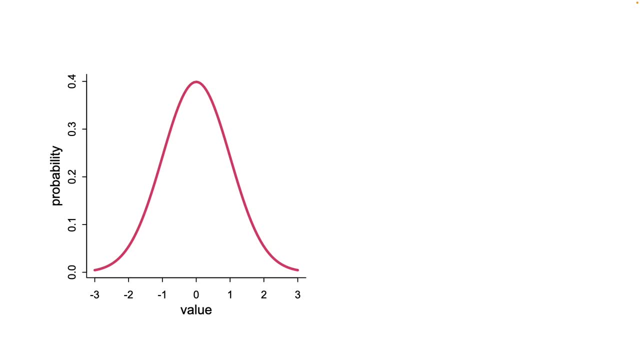 So what I'm showing you on the screen here is a Gaussian distribution, the familiar bell curve. If we take the logarithm of a Gaussian distribution and multiply it by minus one, we get this which I'm going to call a bucket or a skate park. 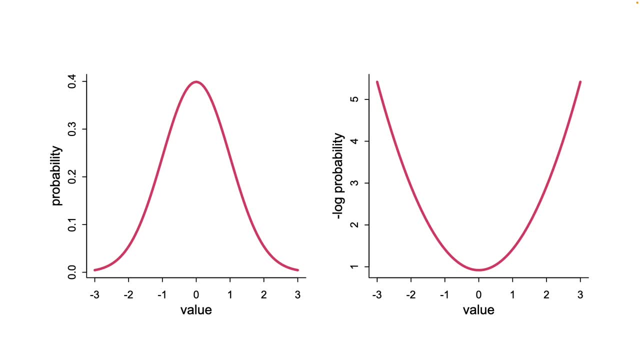 It's a parabola actually, because Gaussian distributions are quadratic, which is why we call it the quadratic approach. It's an approximation. This is a perfect parabola. and the width of the parabola has is proportional to Sigma and its location on the horizontal axis is mu, its mean. 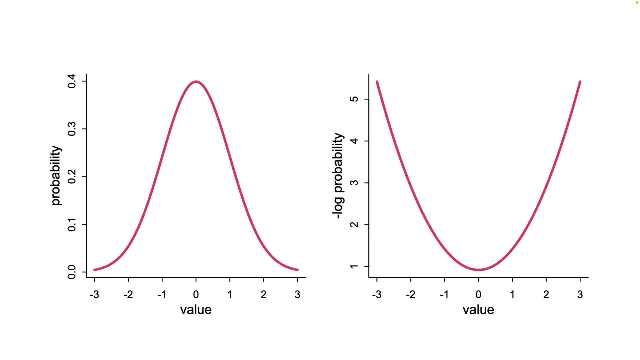 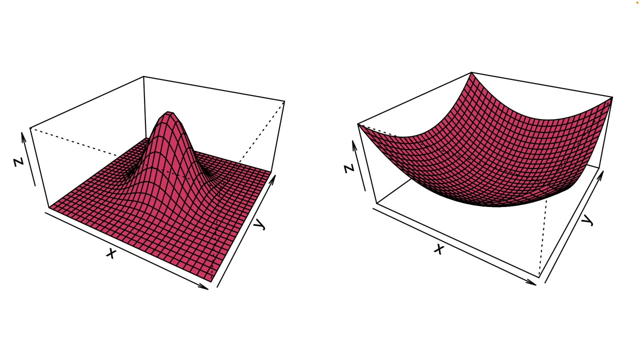 So when we view probability distributions in this log probability space, they're like. they're like buckets, and and these buckets have a gradient in the sense that if you rolled a ball inside them, it would roll downhill towards the bottom of the Gaussian bucket, And this analogy works. 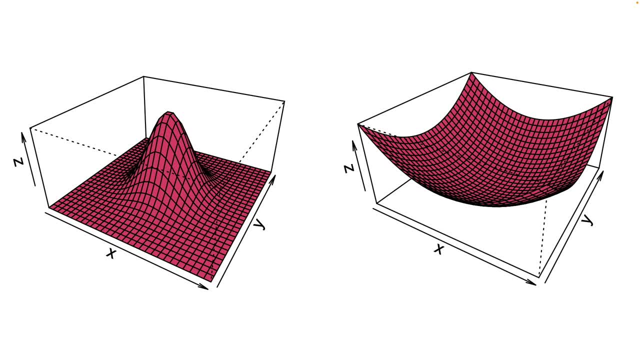 Also in two dimensions. So on the left of this slide I'm showing you a two-dimensional Gaussian distribution. It's now a hill, a Gaussian Hill, in an X and a Y dimension, and the Z is the probability If we take the logarithm and multiply it by minus one. 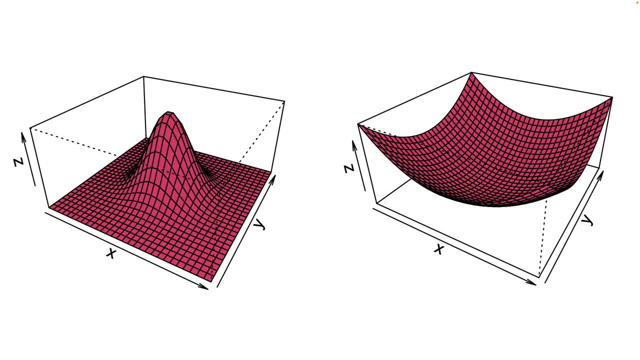 Now we get a two-dimensional Gaussian skate park, as you know, the right of this slide, and, again, if we rolled a marble into that thing, it would roll downhill towards the high probability space, And so this is a hint of a strategy We'd like to use. 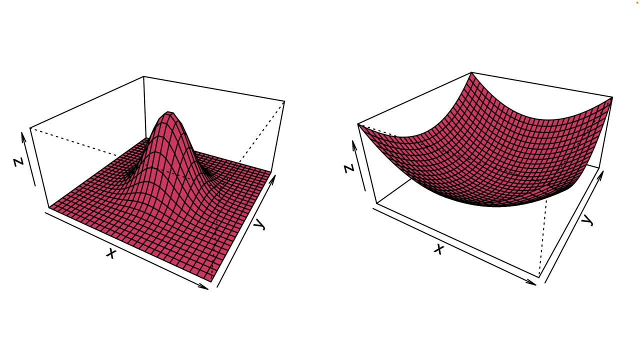 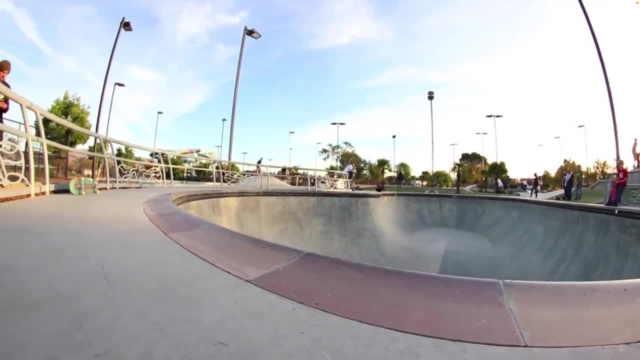 And we will- of basically well rolling marbles inside the log probability distributions. So let's bring this metaphor home a bit. This is an actual skate bowl. I would call this a big bowl. I don't know what people in Europe call these things. 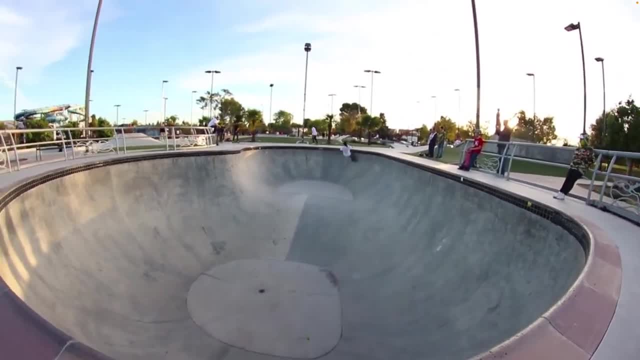 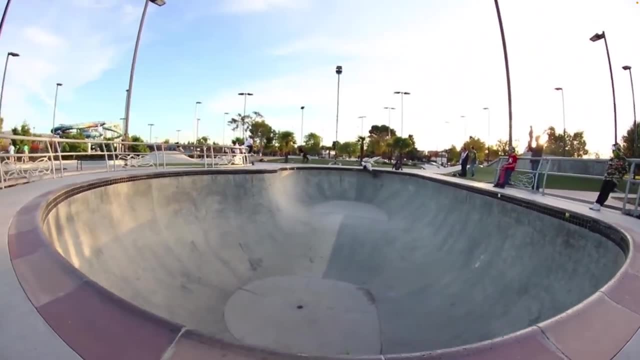 And the very talented fellow who's who's skating through it is, of course, just exploiting physics. His skateboard doesn't know anything, in a sense, about the global shape of this bowl. but it doesn't have to. it just has to know Which direction is up and which direction is down at the point. 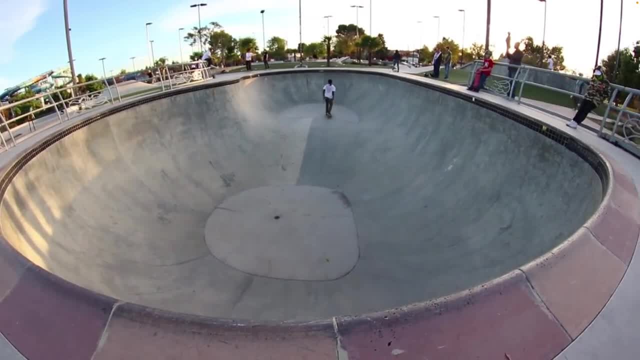 It's at now and gravity takes care of the rest. Well, there's some planning involved, of course, but you know what I mean. So the in with our analogy you can think about this is: this was a log probability distribution. The bottom of the bowl is the high probability space. 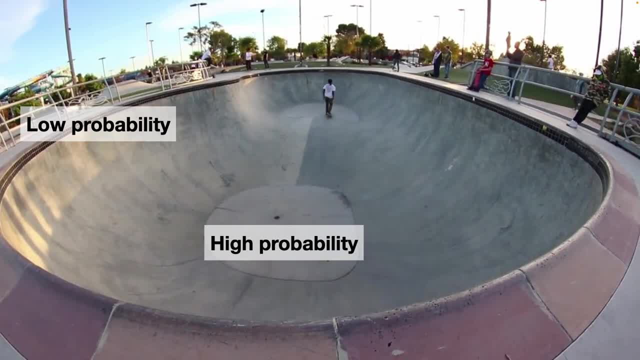 That's where the marbles going to roll if left to its own devices, and the edge is low probability space. So how can we fling a marble or a skateboarder around this thing and collect information on there? Well, we're going to have to find positions over time, such that those positions will be valid samples from the posterior distribution that the bowl represents. 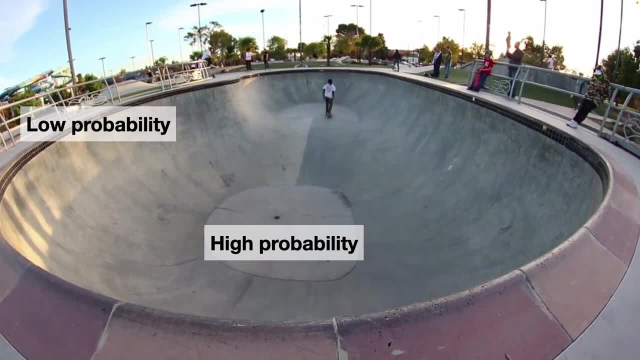 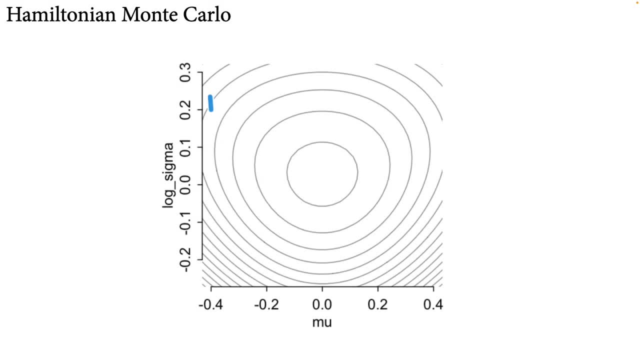 And that's the algorithm We're going to use, as weird as that sounds. So here's the actual algorithm, not a virtual skate park, but for a posterior distribution that I've made. So the book has all the computational details for this, if you're interested, and there's many papers written on this method. 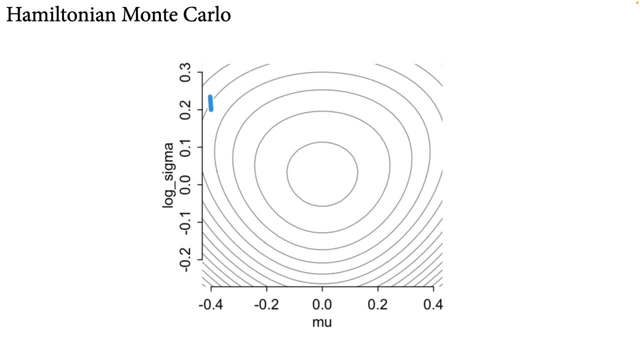 I want to give you some Tuition about how it works. This technique is called Hamiltonian Monte Carlo. The word Hamiltonian merely comes from a certain way of representing a physics simulation, a classic Newtonian simulation with velocity and so on. So same distribution as you had before with mu and log Sigma. 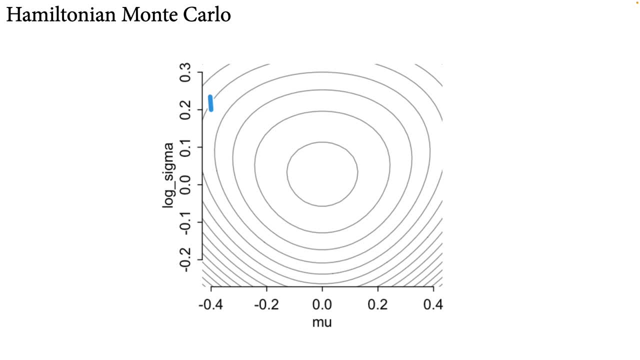 And now, what I'm going to do, though, is I'm going to release a marble into this bowl, And the way we're looking at this top down, the center of this distribution is downhill, And the edges where the Contours are closer together are the edge, that is, higher elevation with higher potential energy. 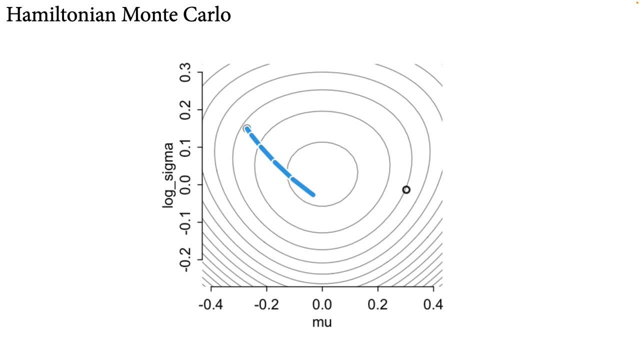 So if we fling a marble from a random initial starting location and just let it roll according to the physics and then stop it at a certain point and record its location, and then do it again from that location where we stopped it, We flick it again in another random direction at a random velocity. 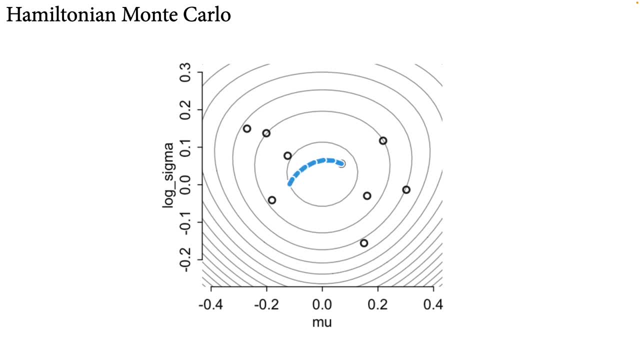 Let her run and then stop it. You see, these simulations are going. each of the black circles, which are the recorded in positions, The of the trajectories that these little simulated rolls through the skate park, Each of those is a sample from the posterior distribution that gives it shape to this physics simulation. 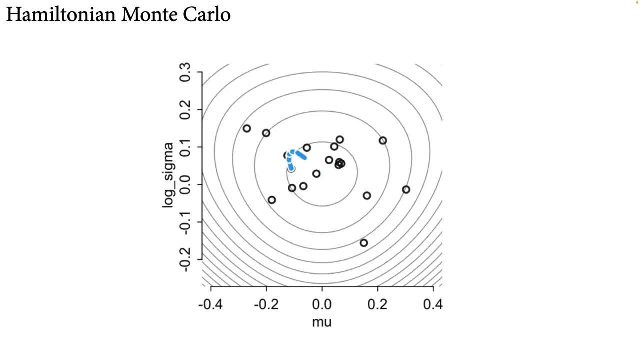 And in the long run or the not so long run, you get a pretty good description of the shape of the bowl that our virtual marble is rolling around in. This is in two dimensions, but the algorithm works in any arbitrary number of dimensions. You just can't visualize it. 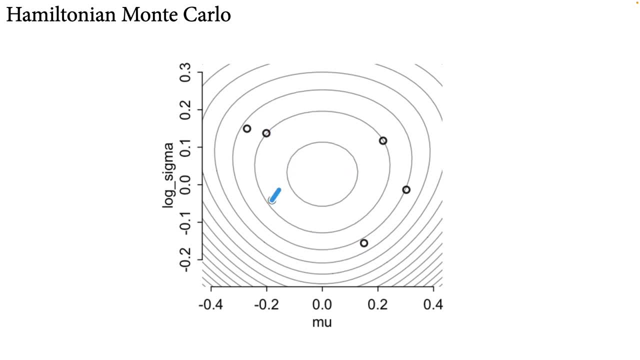 Right. So in three dimensions it's pretty hard to visualize it. in four It's impossible. but we're we can do this for tens of thousands of dimensions. The computer doesn't mind because it doesn't need to visualize it. but it's the same basic principle. 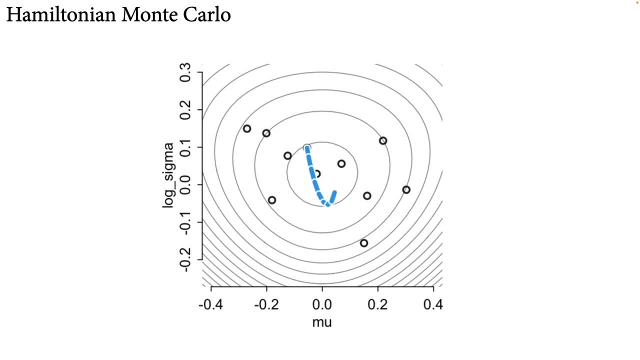 There's this in dimensional surface and it's got some curvature and we're going to run it like a physics simulation and let things roll around on it and record their positions. It's amazing. again, This actually works. It's exploiting randomness, but it's also exploiting the, the physics metaphor and the fact. 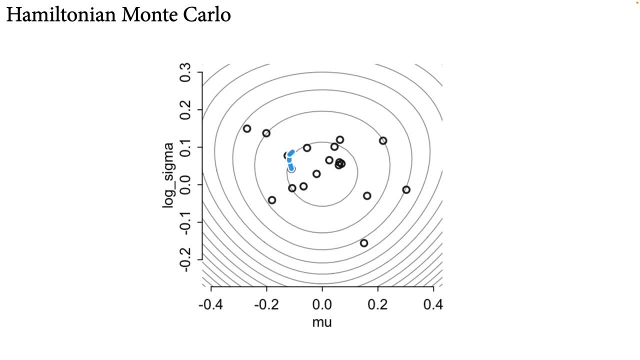 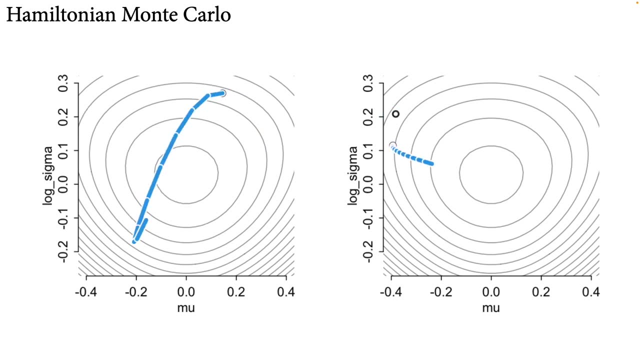 that we can do, do analysis on that thing to prove that this works. So just to show you, there are things to tune about this as well, like step size. So the the little segments in the blue trajectories are individual linear approximate steps in the physics simulation. 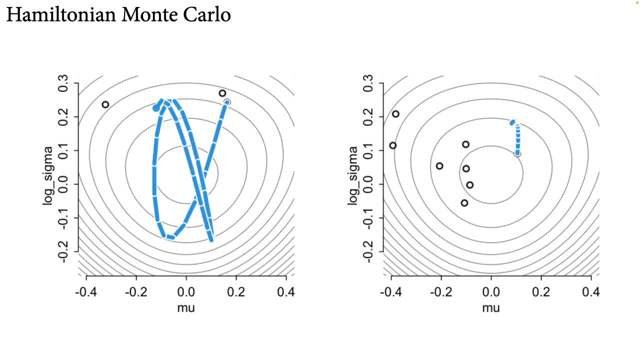 and they define sort of the coarseness and speed of the of the virtual particle that we're using to take samples from this bowl. And and if you make those steps and the trajectories, the steps big and the trajectories long, having many steps, then the the skateboarder tends to loop around a bunch of time. 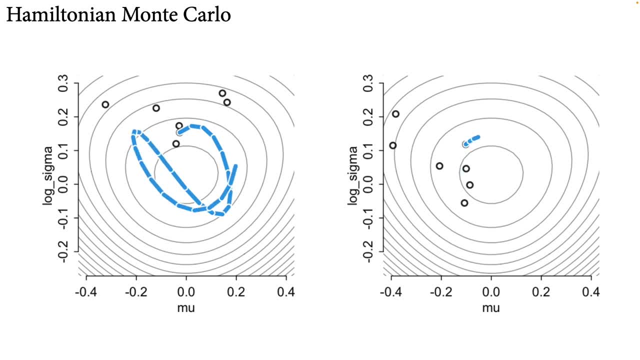 and do a bunch of tricks before reporting his position. Finally, one of the side effects of this is if you, if you tune it badly, is you tend to return to where you started, and that's what you're seeing on the left. This is a so-called you turn, you turn phenomenon, where the trajectory turns around. 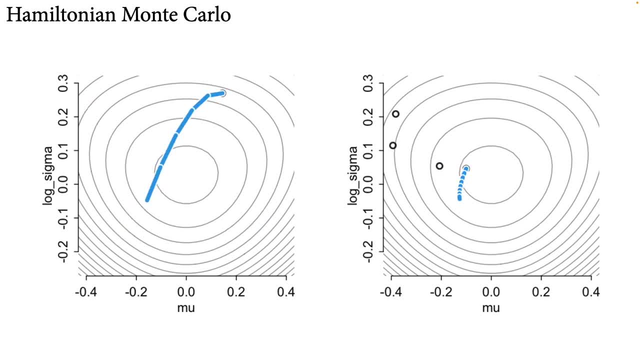 and comes back to near where it started, and this is inefficient. We don't want to do that. We want to stop in a different place And so to use these algorithms in practice, you don't have to tune them, But if you do, you get much better performance, because they won't return to where they start on the right. 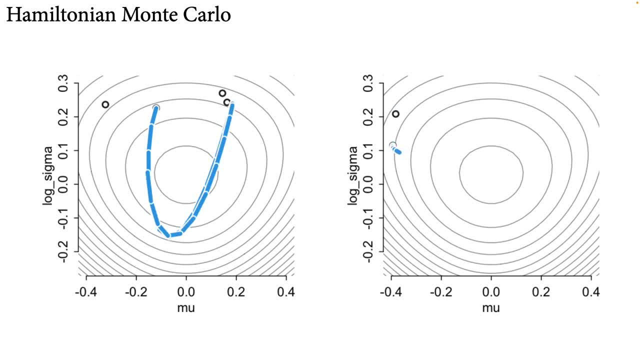 We have a simulation that doesn't tend to do the u-turn, but it also takes a much longer time to explore the whole space because we're taking really small fine steps and we're not moving very far in any particular simulation, which means it takes much longer to get a good overall picture. 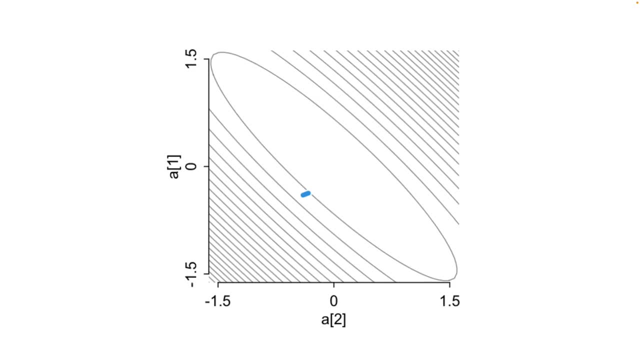 Of the shape of the bowl. But one of the great virtues of this algorithm, the Hamiltonian Monte Carlo, is that it finds a path through the curvature of the shape. So here's a posterior distribution need two parameters that are highly correlated with one another. 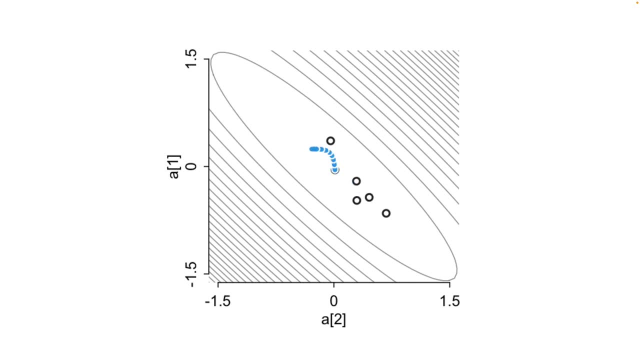 which is fine. parameters can be highly correlated with one another. that doesn't break any law of probability theory. but Metropolis algorithm often has a problem sampling from such distributions because it keeps it doesn't know anything about the global shape, It's just making completely random. 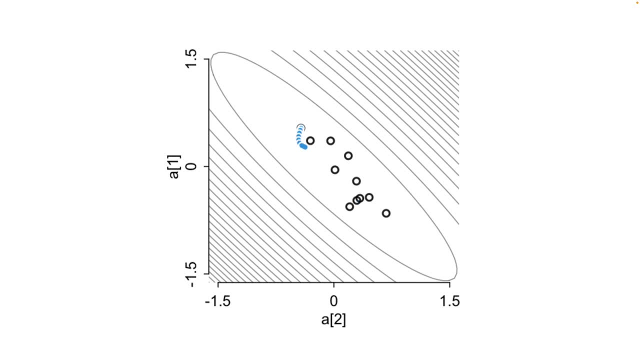 The proposals, and so it keeps making proposals out into the low probability space outside The, the, what you call. that surfboard shape or pickle shape in the middle of the slide here, Hamiltonia, Monte Carlo and contrast, as you can see- moves around according to the curvature of the space in the middle. 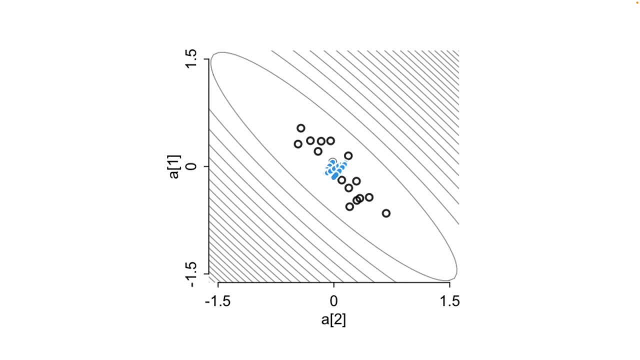 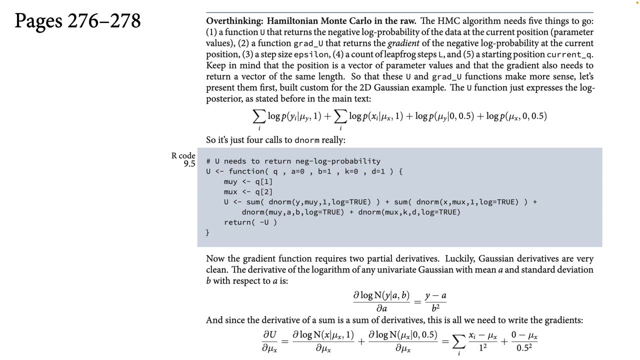 and take samples from the high probability region where it wants to be. So if you're interested in all the details of this algorithm and how I made those animations, it's all in the book. you want to look in on pages starting at 276 and there's a long overthinking box that has a complete code example is not even that much code and relates it to the mathematics behind it. 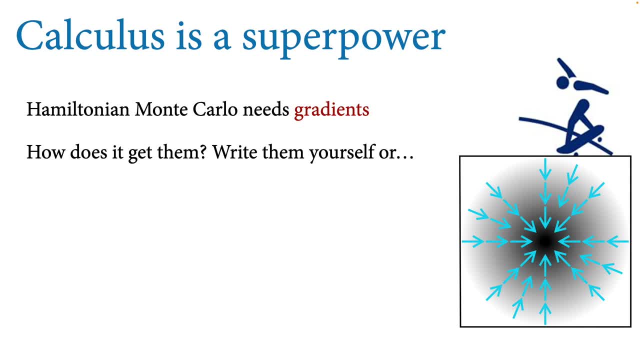 But by no means is it necessary to understand exactly how it's programmed to use this algorithm. That's not your job, That's the, that's the engineering job that's been done for you, And we're going to use a math library that does all this for us. 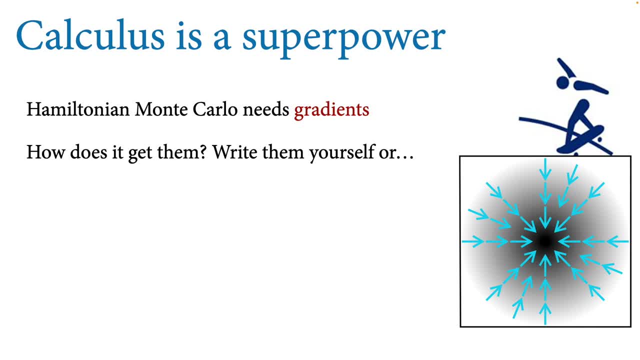 And what the math library does is? it gives us the most important ingredient: the gradients. So the gradients tell us where, which direction, from any given point, is uphill and downhill in every direction, in the, every dimension, in every parameter dimension. That's the gradient. 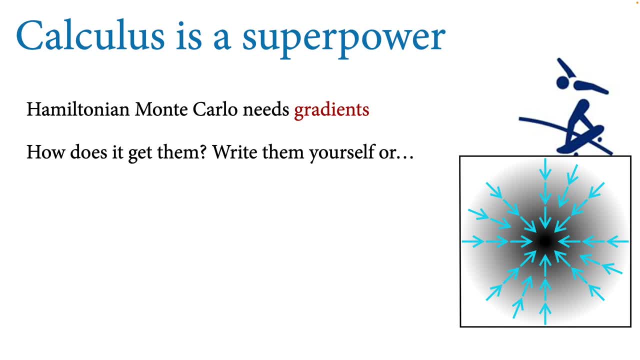 So we need some way for any combination of parameter values to know which direction is uphill or downhill. Yeah, and so how do we get those things? Well, you can write them yourself by doing calculus. You can take the probability, the definition of the 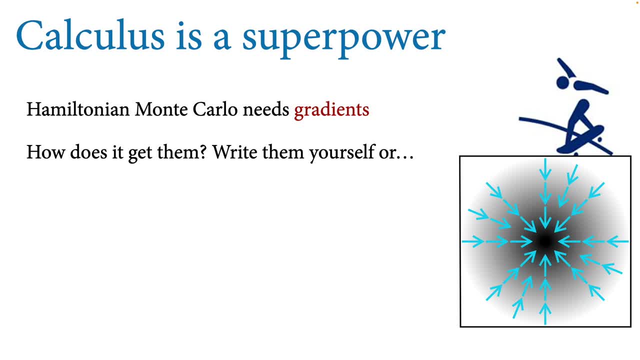 of the posterior distribution for your particular model and you can use calculus like the chain rule to take the derivative of it in each direction with respect to each parameter. You can get your gradients that way. That's a lot of work and it means you have to rewrite your code every time you change your model. 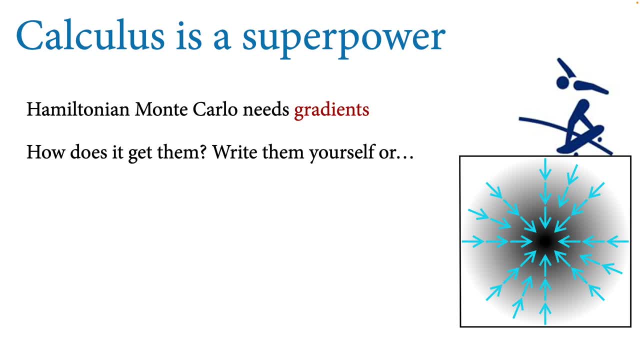 We'd rather have something that's just kind of like plug-and-go right that works. There are lots of algorithms that try to use approximate gradients numerically by something called finite differences, And in fact that's what we've been doing so far with crap. uses finite differences to estimate gradients for big models and especially for Marco chain, Monte Carlo. 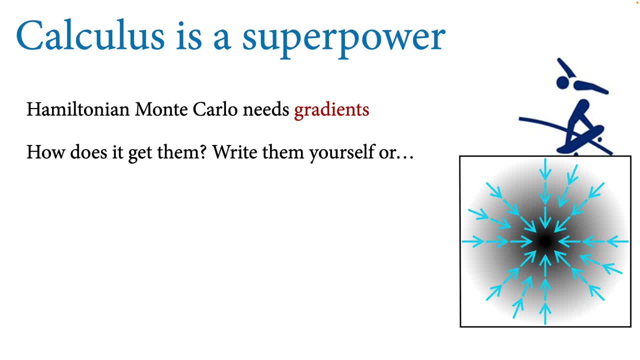 That's not going to work because it's not accurate enough and it descends into merit, to numerical nightmares. So we're going to do instead is use this really slick technique called auto diff, which stands for automatic differentiation. What automatic differentiation does is it's a set of methods that actually takes derivatives of code. 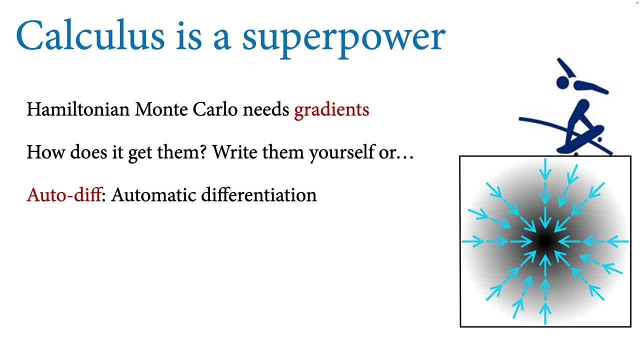 So you can program your model as code, as you've been doing, And then the auto diff library will find the derivative of your code. I know it sounds wild, but the reason is possible is because every, every component function in your code has a known derivative. 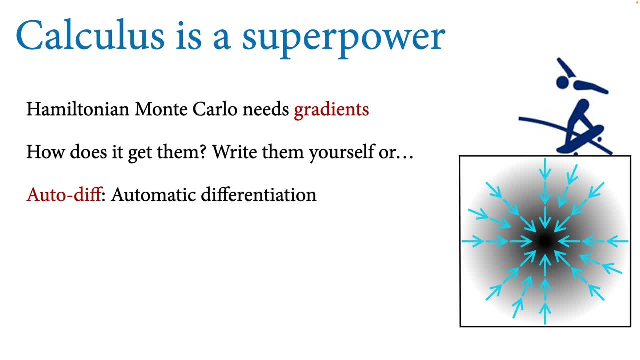 And it's a wonderful thing about derivatives is that there's this thing called the chain rule that lets them, lets us break them down into a set of smaller derivatives, And that's how an auto diff library works. You get, gives you symbolic derivatives of your model code so that they're accurate. 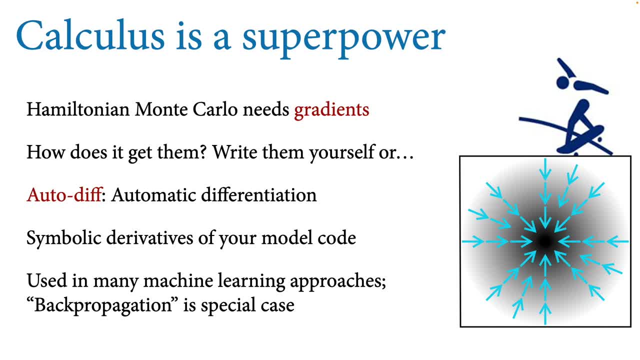 This is your code. This is used in, not just in, Bayesian statistics these days, So it's a workhorse in Bayesian statistics. It's used all over in machine learning. If you may have heard the term back propagation, which is used a lot in neural networks, back propagation is the same thing. 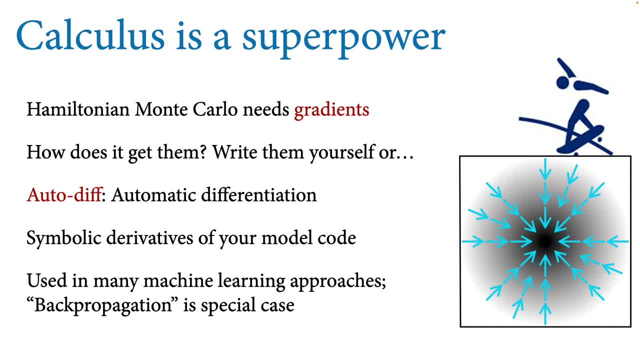 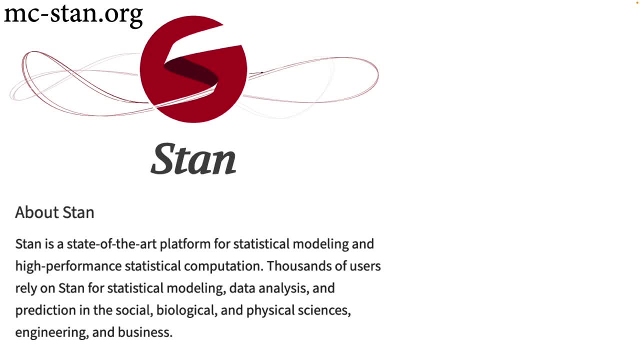 It's just a particular application of it. The library we're going to use is the is called Stan. Well, Stan is kind of the whole ecosystem of software. The Stan math library does the auto diff and Stan is a set of tools, Tools and interfaces for using that library. and this is what we're going to use. 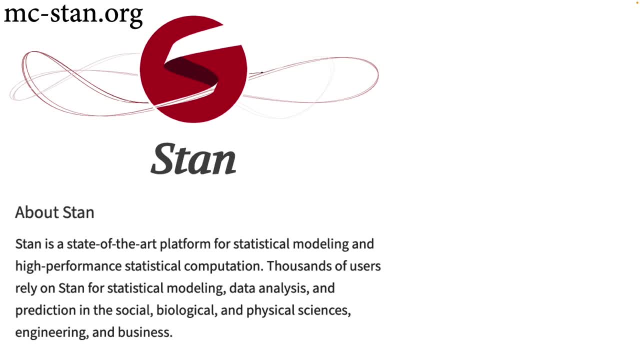 It's already on your computer, probably, and you can use it. They're also really good libraries, like touring in the Julia environment that also used the same kinds of algorithms but uses a different math library. Those are excellent as well. Stan is not an acronym. 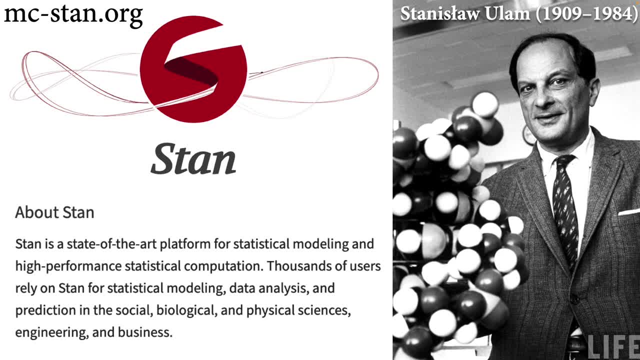 Usually things in computing are like this or an acronym, but Stan is not an acronym, It's a name. It's named after this fellow, Stanislaw Ulam, who, who lived until 1984 and made many, many important contributions in computing and mathematics and biology. 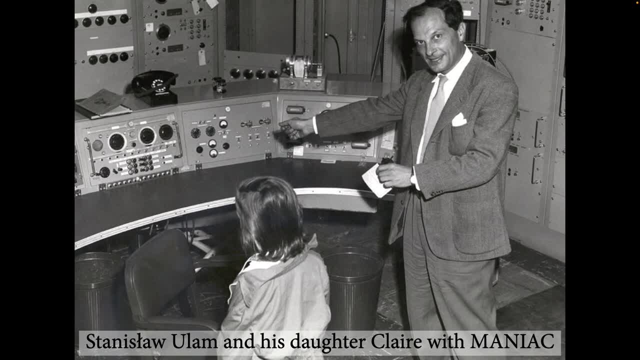 And he actually worked on the maniac project at Los Alamos. Here is an old photo that I quite like of him in one of the maniac control rooms with his daughter, Claire, who was fairly young at the time and I'm not sure what he's gesturing at. 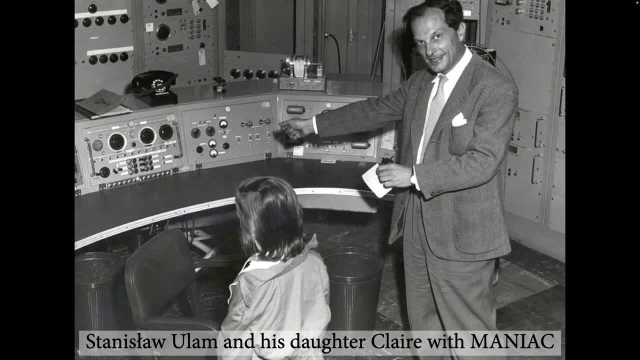 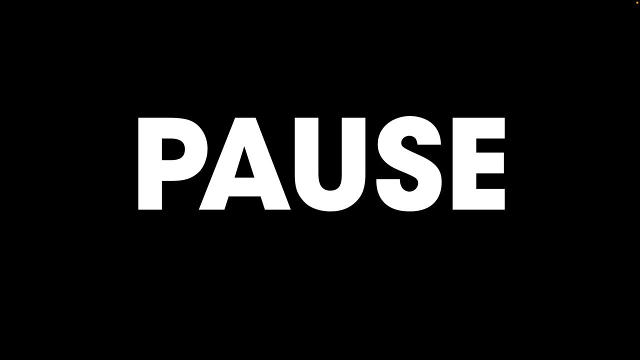 but that terrible control panel I would not like to operate a computer with. Okay, that has been your introduction to, conceptually, to Markov chain, Monte Carlo, why we need it and a cartoon version of how it works. Let's take a break now and purge some of that from our minds. after you've relaxed a bit and come back. 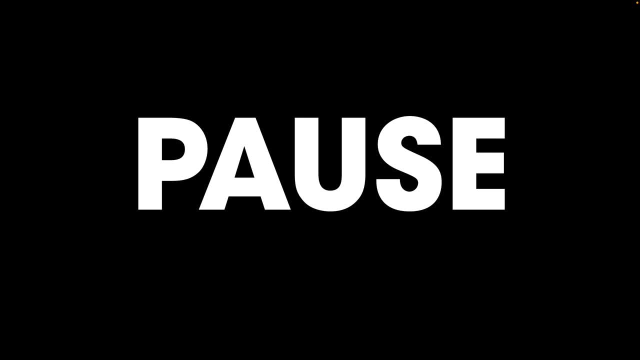 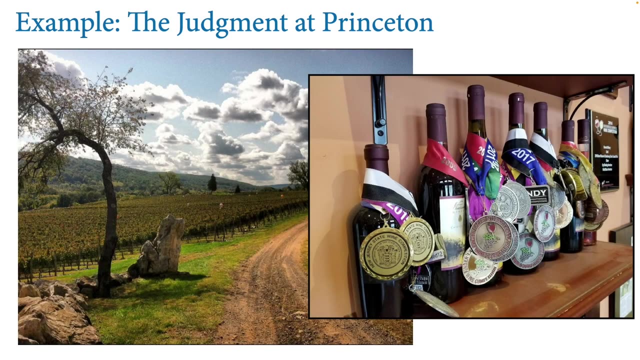 We'll continue forward and I'll show you actually how to actually use it. Welcome back Now. most people don't think of New Jersey on the eastern coast of the United States, as a home of good wine, but it is. New Jersey grows and has grown for decades. 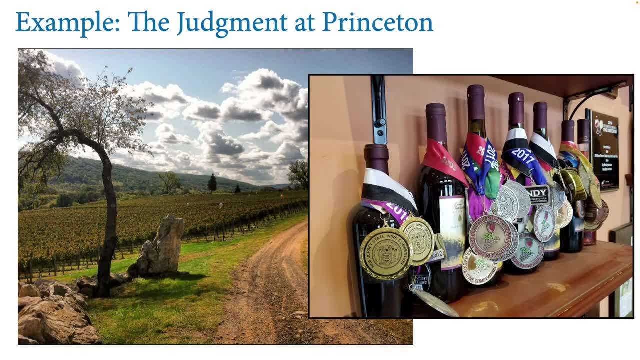 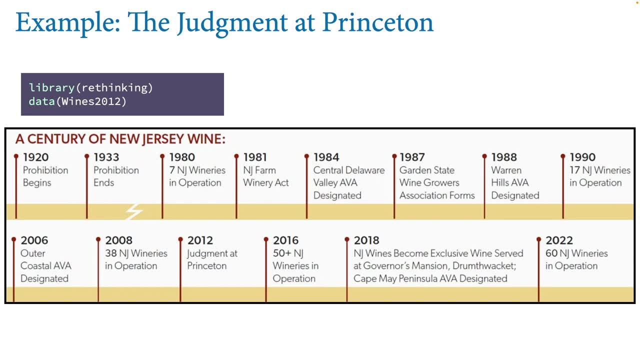 Now some of the best wine in the world, that is, according to international judges. It's a long history of how this happened. It hasn't always been true. There's not, as in some parts of Europe, hundreds of years of wine culture in New Jersey. 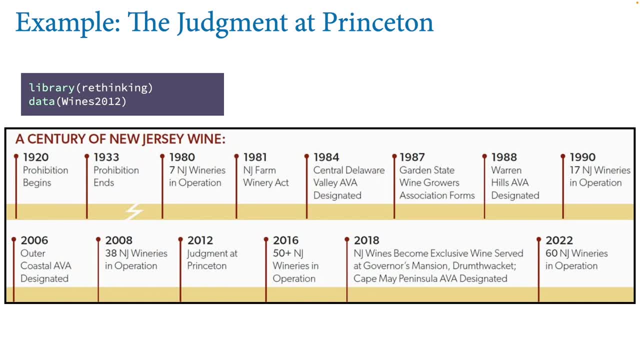 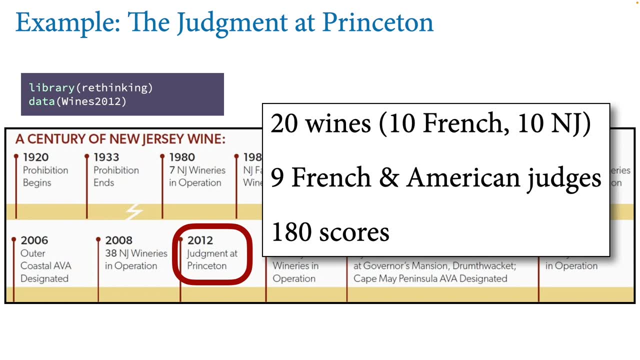 but there's a very particular moment in this timeline of the development of New Jersey into a world center of wine growing. That is, in 2012, in 2012.. Something happened in Princeton called the judgment at Princeton, and the judgment at Princeton is when an international panel of professional wine judges both French. 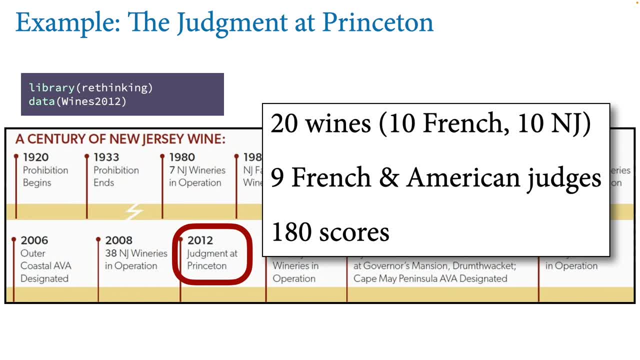 and American, Judged 20 different wines- 10 French and 10 grown in and produced in New Jersey, and assigned 180 scores to these wines, And this is the judgment that put New Jersey on the international wine map. We're going to look at this data set as an example of how to use Markov chain Monte Carlo. 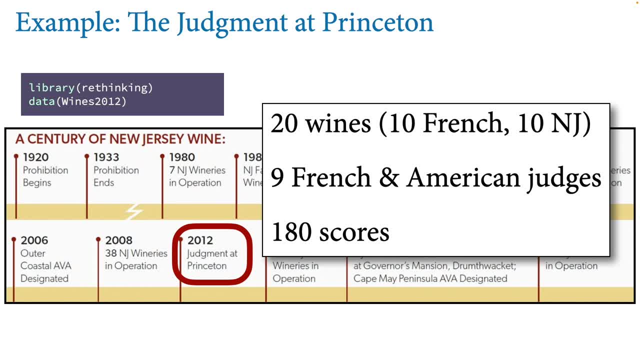 So I can introduce you to some of the due diligence involved in running Markov chains, but also a way for me to introduce a new kind of model to you, Something called an item, A response model that is used to model scoring events like this. 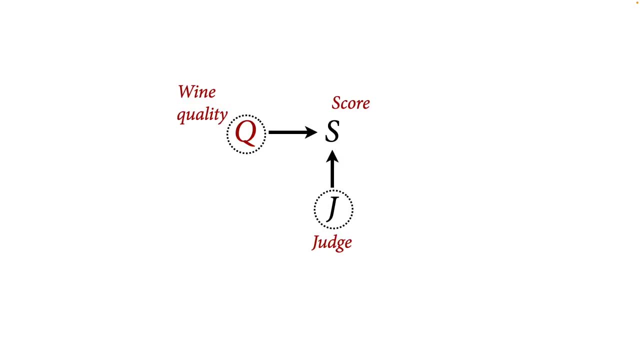 which are incredibly common. So let's make a dag. as always, We're interested in measuring the quality of individual wines, which I'm going to represent here with Q and Q's in a dashed circle because it's unobserved. We cannot directly determine the quality of the wine, because that is determined by the people, preferences of judges. 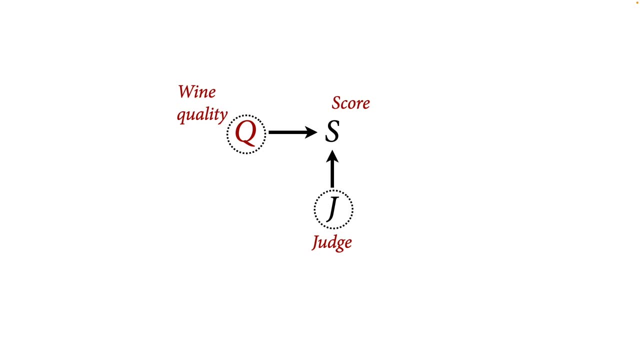 What we do get to observe is a score That is assigned, and each score is assigned by a particular judge and judges. Judges also have unobservable characteristics which influence the kinds of wines that they like, And so the score is a cause of both the quality of the wine and the disposition of the judge. 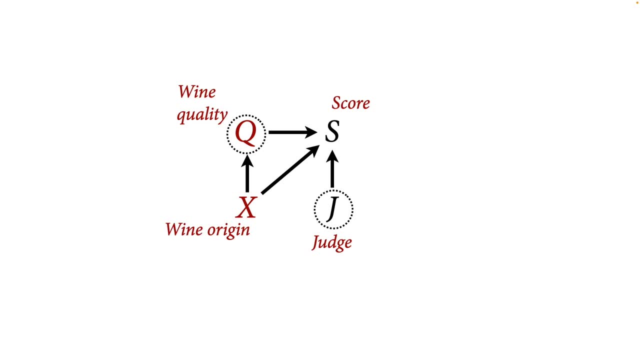 And then there are aspects of the wine which may also influence its score, either indirectly, because, say, like wine origin, whether it's grown in New Jersey or in France, the wine origin will change the nature of the grapes and the kind of wine you get, and how the wine is produced in different places as well. 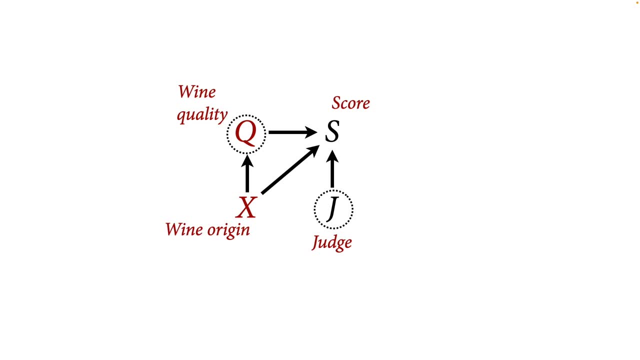 And so that may affect the quality, which influences the score indirectly, or there may be direct influences of the origin of the wine on score. How would that happen? Well, the most obvious way is through the bias of judges. If a French judge knows, by reading the label, that the wine was grown in New Jersey. 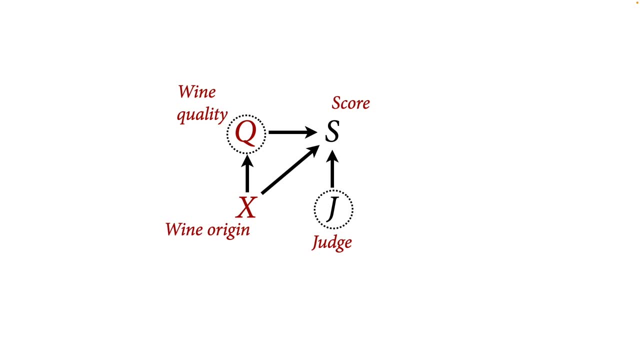 that may actually reduce the judge's enjoyment And result in a lower scoring. And that's why, in things like at the judgment at Princeton we have this: the origin of the judge is a likely cause of those preferences, of those biases. New Jersey judges are probably more likely to like New Jersey wines and French judges French wines. 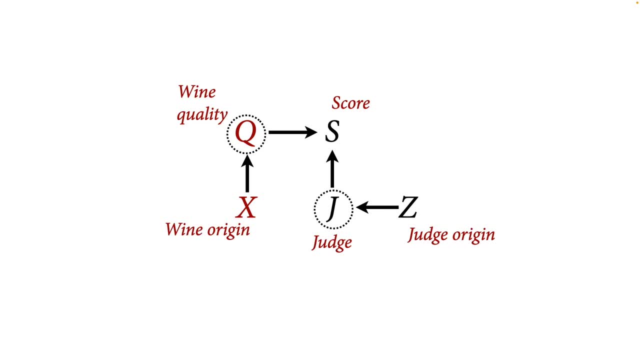 And that's why in these sorts of judgments they blind the judges to the origin. They remove all the labels, They don't have them in original containers Or decanters, And that's to remove any direct effect of the origin of the wine on the scoring. 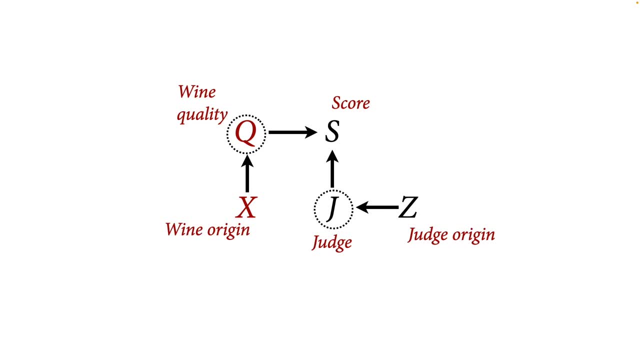 So in the DAG I have on the screen here, there are no confounds. really We don't. there are no backdoor paths to close, But our S demand is still going to require estimating wine quality and stratifying it by wine origin. 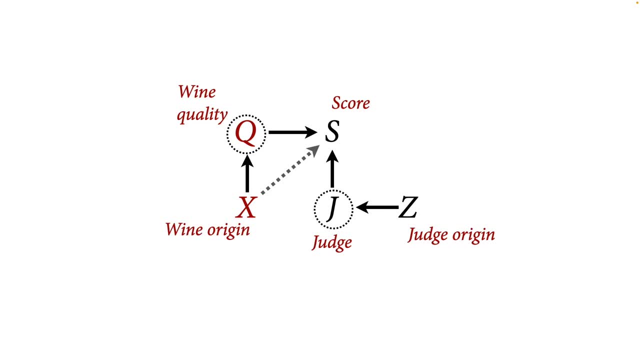 And maybe we want to, can do that anyway. stratified by wine origin, because there might be a confound If the blinding is not 100% accurate, as I've tried to indicate here with the dashed arrow. if judges can kind of taste some of the characteristics of a New Jersey wine and guess. 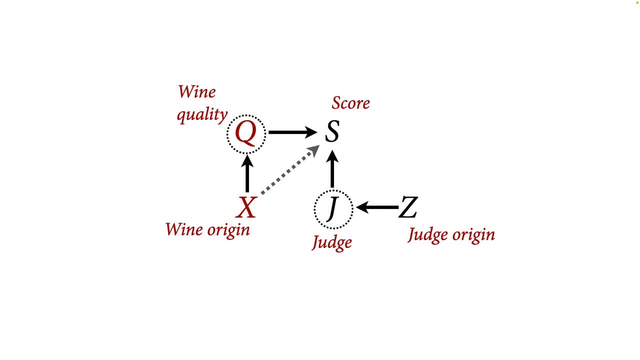 or maybe the colors are a little different because the grapes are different, then they might. that might activate their bias as well, And so stratifying by the wine origin could be useful. for that reason, because it's a confound, Remember we're trying to isolate the quality differences here. 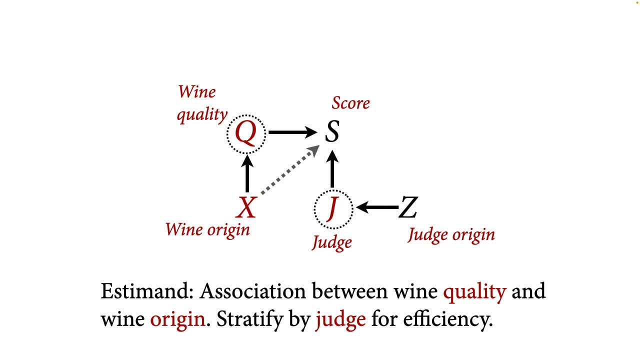 Our S demand in this analysis is going to be the association between the quality of the wine and its origin as scored by the judges. And now, judge is not a confound right. You learned the backdoor criterion in previous weeks And there's no reason we have to stratify by judge in this analysis. 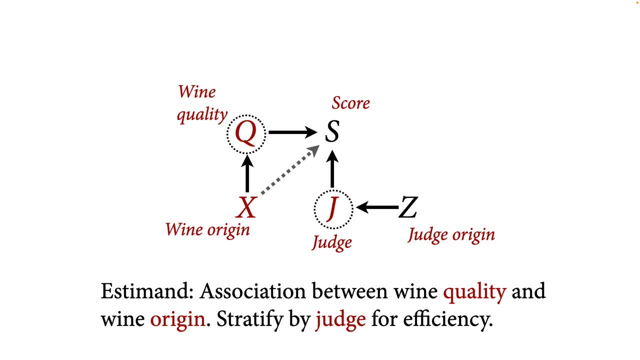 But we're going to do so because judges is a competing cause of the score And judges have their own biases. Some of them are harsh, Some of them are easy, Some of them are discriminatory. Some of them are non-discriminating, meaning that they give wines that are even a little bit different. 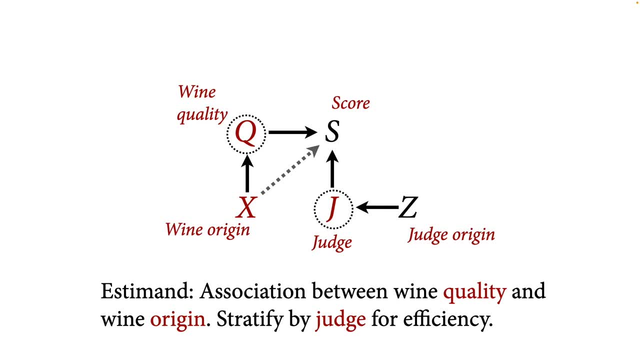 wildly different scores. Some judges are non-discriminating, meaning they give almost all wines the same score, And those differences in the judges obscure our ability to measure the quality accurately. So if we can estimate those features of the judges, we can possibly do a better job. 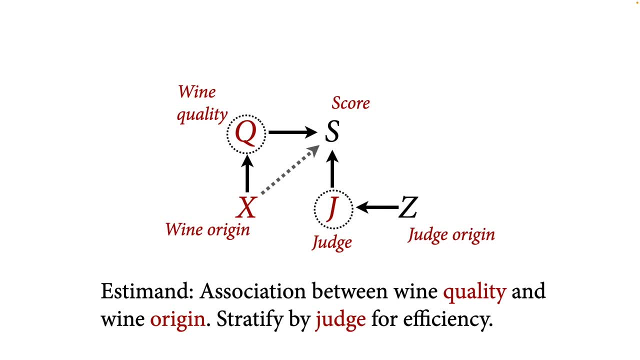 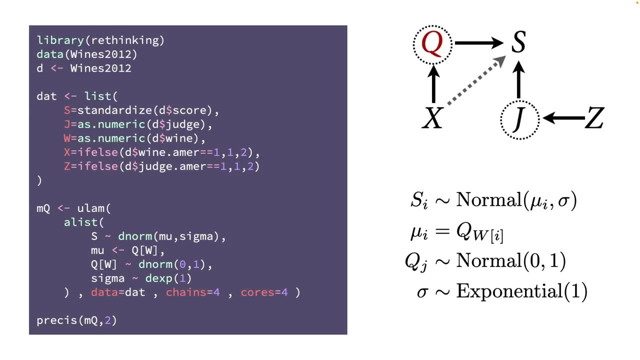 And there's a whole family of models- latent variable models, item response models- that are designed to deal with data structures, which are exactly this kind. So let's do an example of one. I'm going to build it up in components, I'm not going to do the in-goal model all at once. 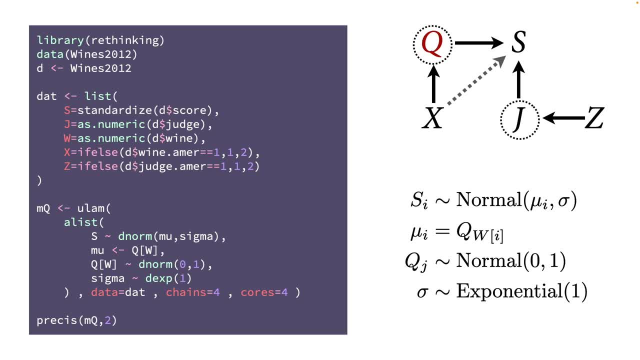 And that's because that's not how I work and it's not how you should work. You should build a small, simple model with one little explanatory variable, first make sure it works and then add in the next bit, and so on. These golems can get pretty complicated. 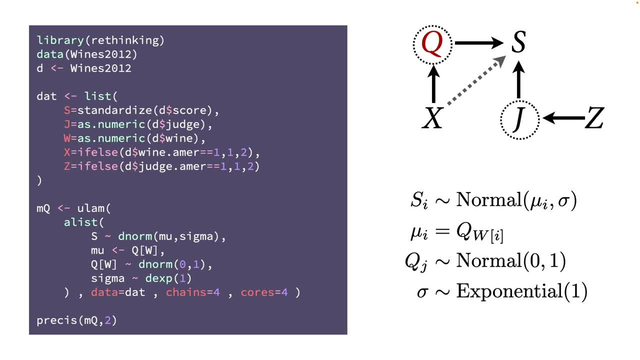 And if you try to build them in one go, something will not work and you won't know what it is. And if you build them piece by piece and make sure after each little adjustment it still runs, you'll be in much better shape and you'll be much happier. 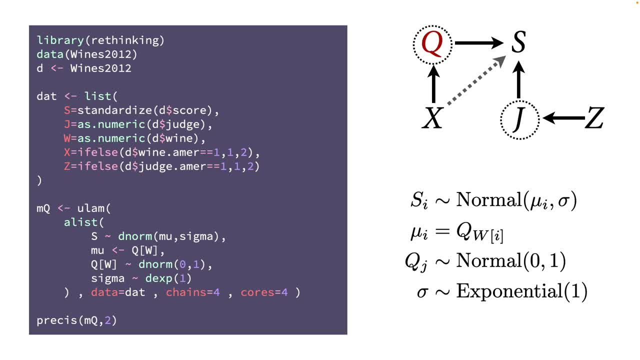 Okay, So on this slide. first we just load the data wines 2012 as part of the rethinking package, and I make a shortened data list with variable names to match the DAG in the upper right. here I've standardized the score. 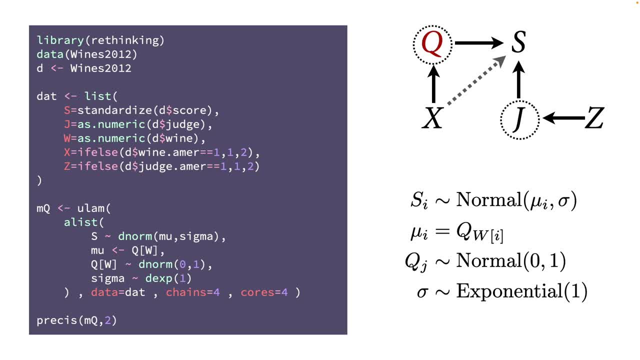 So in the original judgment they could assign a wine between 1 and 20 points. I've just standardized that variable, which means I've made the mean 0 and the standard deviation 1.. This is useful for defining the priors when we get down to the model below. 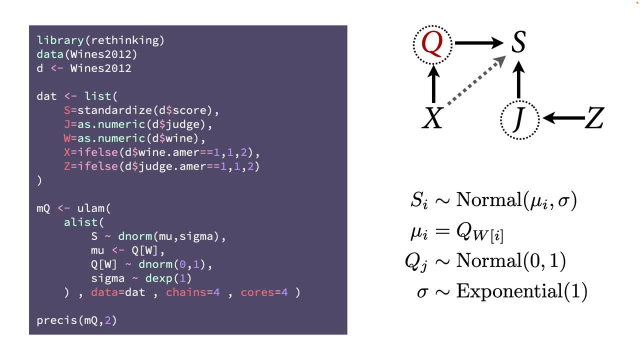 After all, 1 to 20 is an arbitrary scale. Then we get to the model. This is still linear regression. We haven't really learned how to use anything else yet, but we will next week, Empowered by Markov chains, we will do all kinds of stuff. 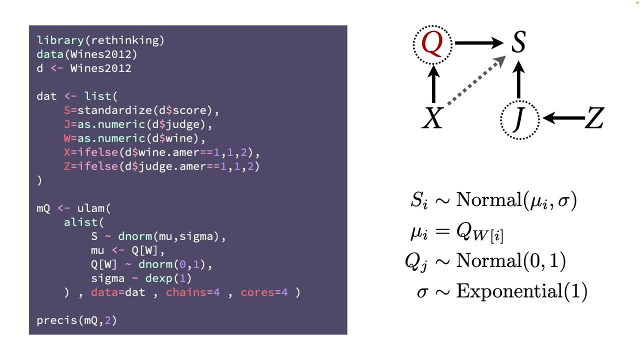 And we make the mean of each. So the way this data works is there's 180 scores and each score has an associated judge and wine, And the variable w is the index of the wine and the variable j is the index of the judge. 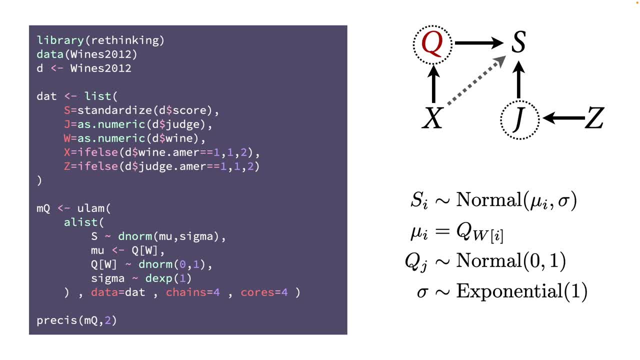 That's their name, so to speak. And then x is an index for the origin: New Jersey is 1., France is 2.. And z is an index for the origin of the judge. Again, 1 for American, not just New Jersey. 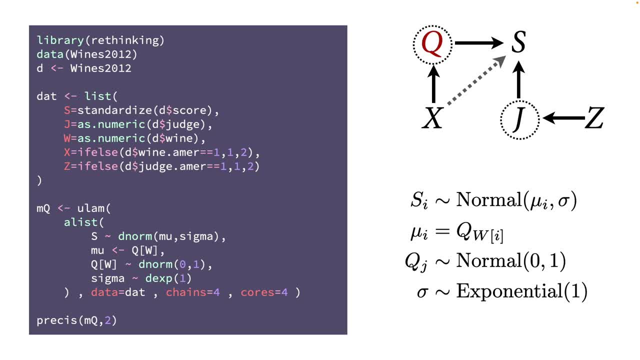 And 2 for France or Belgium. I think there's one Belgian judge, And then the model at the bottom. What I want you to notice is this looks just like a QAPP model, but the function is named Oulam, after Stanisław Oulam. 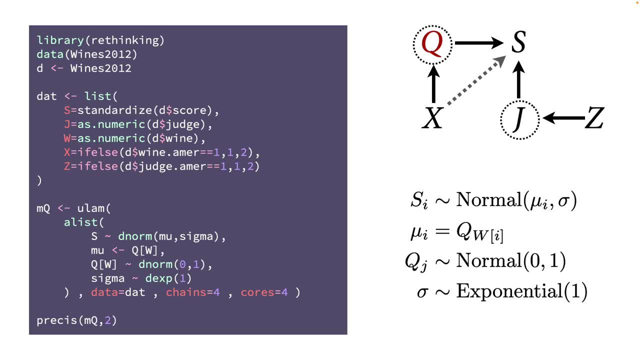 And this will take the same kind of model formula that you used in the first part of the course and it will build a Markov chain for it to sample the posterior distribution. And the Oulam model will return only samples, but you can interact with it in most of the same ways. 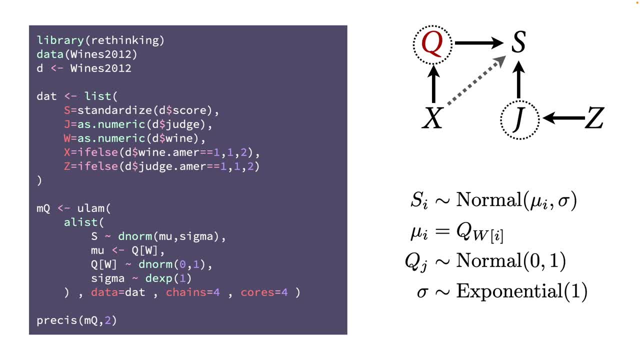 You can interact with a QAPP model fit. So the expected value of each score s is given by the quality parameter q for the wine that received that score. whichever index w refers to, You remember categorical variables from weeks ago. 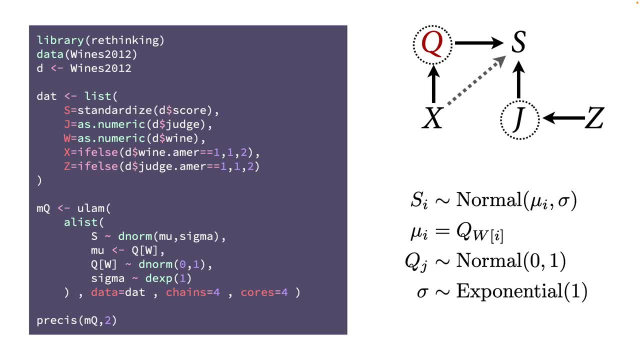 And then I assign that whole vector of q variables. There are 20 of them because there are 20 wines A normal 0, 1 prior. Why normal 0, 1?? Well, because the average score is 0.. 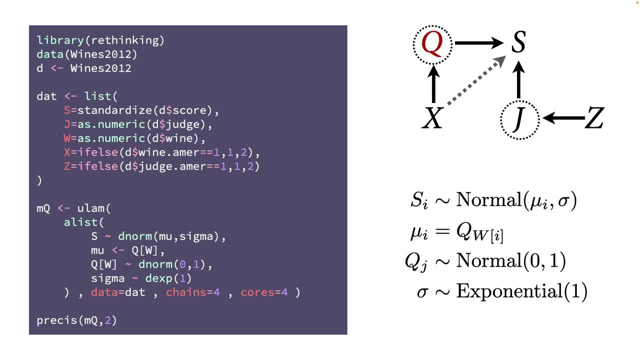 So the average wine must have a quality of 0.. And the standard deviation of the scores is 1.. So the quality dimension is latent and it's arbitrary, and so its scale is arbitrary. so we can do this effectively. So we pass the data, and then there's a couple of additional function arguments. 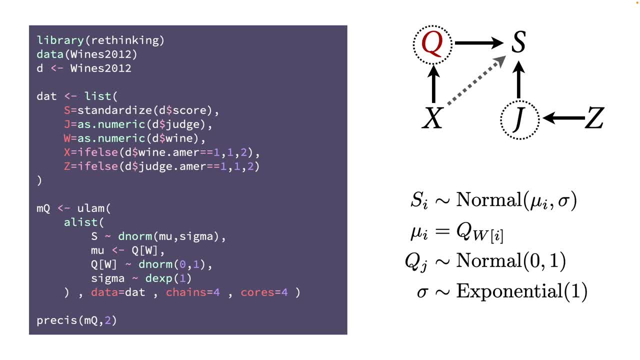 that you use when running Markov chains. The number of chains- chains- equals 4, and the number of cores- cores- equals 4.. And I'll explain these two things a little bit later as we move through, So just hang on while we get there. 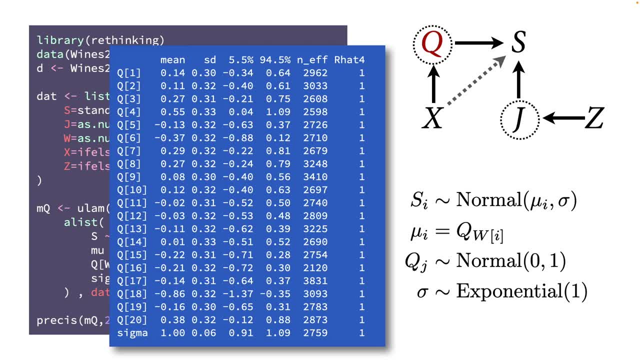 First let's look at the pricey output. just the summary. So you run this model Again. it'll do some sampling, It'll build the Markov chain all by itself. You don't have to do anything And do the automatic differentiation to find the gradients. 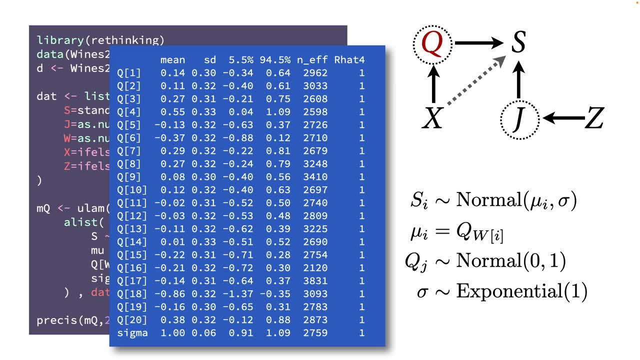 and then it does the Hamiltonian simulation. you know the virtual skate park, And then you can look at the parameter summary with pricey, just like you could with a QAPP model, And you see here the 20 wines, the 20 q values. 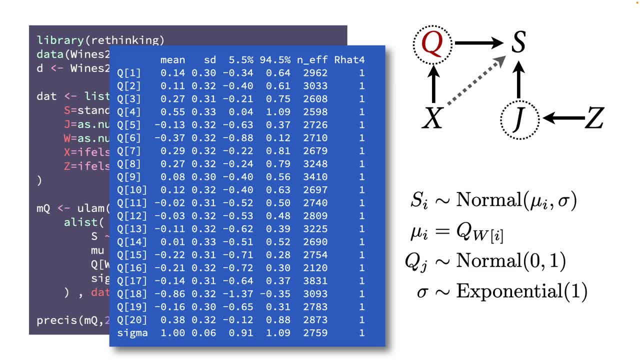 And one lone sigma at the bottom, And you'll see the wines do vary. That's the only thing I want you to get from this, And I also want you to notice that there are two new columns in the pricey output for an ULAN model that weren't present for QAPP. 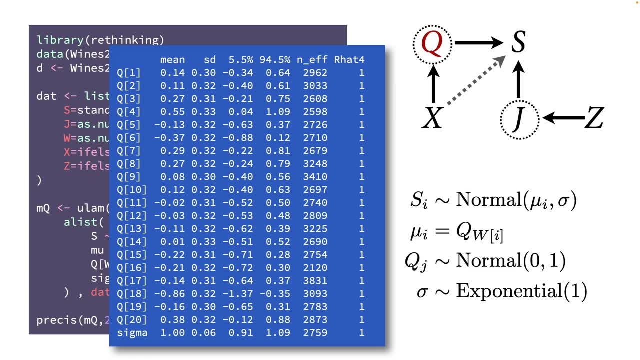 and those are NF and R, hat 4 on the far right, And we're going to explain those in a few slides. Just hang on. But these are there because they're diagnostics, to help you know if the Markov chain is efficient and how good the approximation is of the posterior distribution. 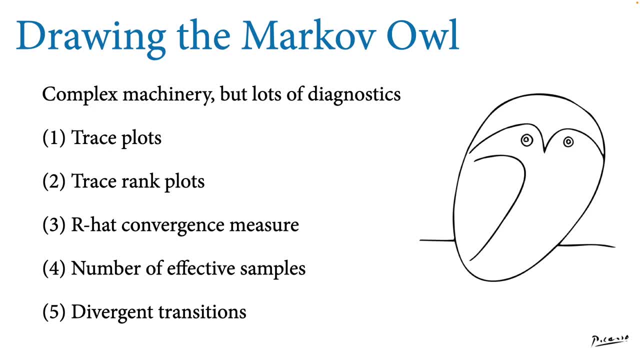 Okay. So when we draw the owl and we're using Markov chains, there's a certain amount of due diligence. after you run an ULAN model, You make some minimum checks to verify that the Golem worked correctly, because Hamiltonian simulation is complex. 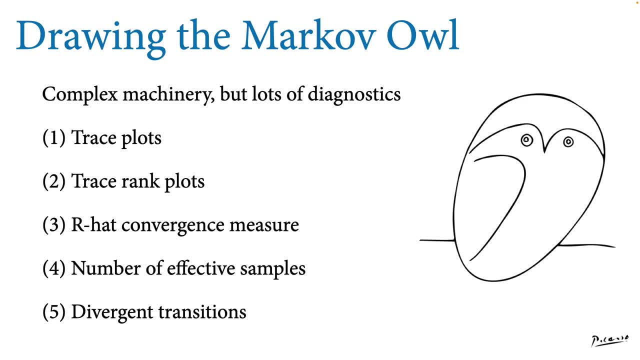 It works unreasonably well, But we still have to check it, And I want to introduce you to five different ways, five different things to think about and ways to check the efficiency of the chain and assess whether you need to adjust the model structure to make it run more effectively. 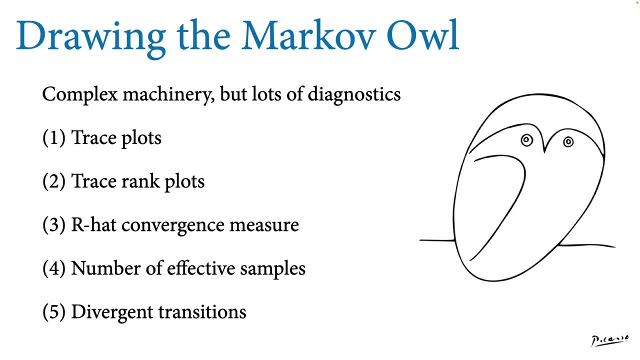 And we'll deal with problems like this throughout the rest of the course, where I try to give you advice on how to make your code more efficient, to debug common problems and making these things run, Because the truth is, for scientifically realistic, analytical problems, there are always coding problems and problems getting the thing to run. 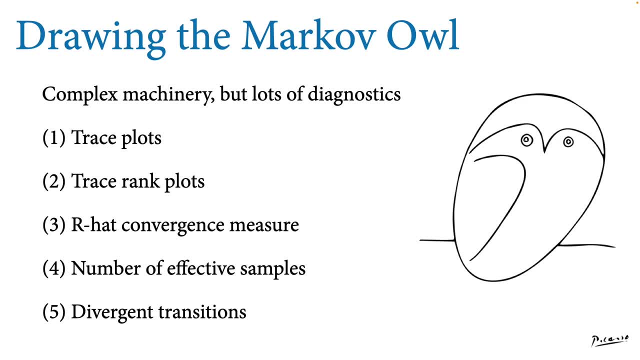 and there's no avoiding that. You can't fall back to some worse approximation Without making even bigger problems for yourself. It's better to work a little bit harder and get an answer to the question you really want to ask. Okay, So we're going to work through these one at a time. 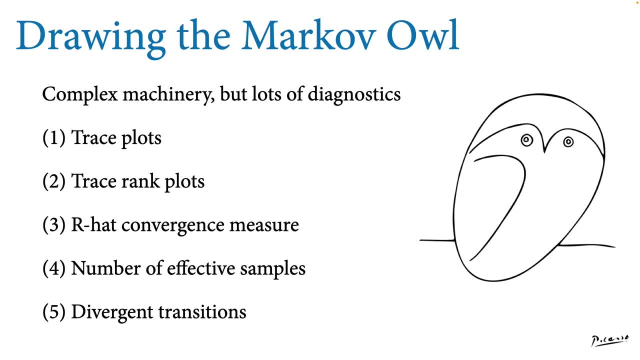 We'll talk about trace plots, and then something called trace rank plots, And then this famous measure, R hat you may have heard of already, and this thing called the number of effective samples, And then, finally, I'll merely mention divergent transitions, but I'll explain them in later lectures. 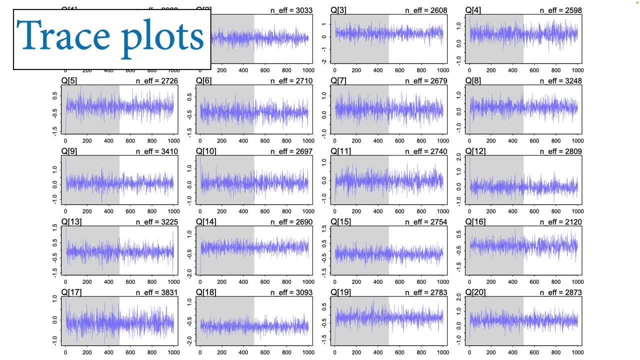 Okay, So the first thing is trace plots And these plots maybe you've seen before. They're very commonly associated with Markov chains. They're just a visualization of the Markov chain. You just take the sequential samples, the chain, and you plot them with sample number in the sequence on the horizontal. 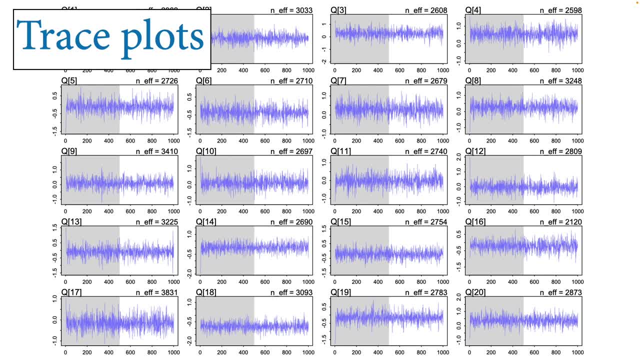 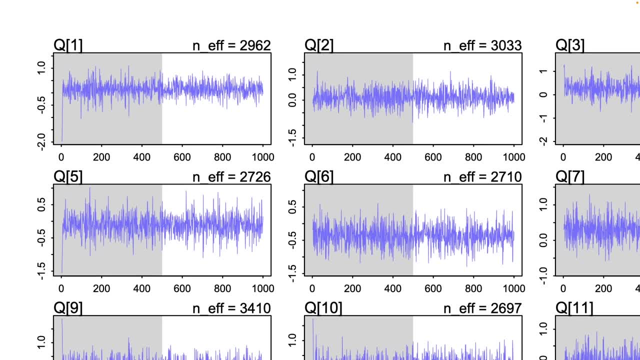 and then the value of the parameter on the vertical. And here you see the trace plot for all 20 Q values from the model we just fit, And when you zoom in to any one of these you can see what you want to see. 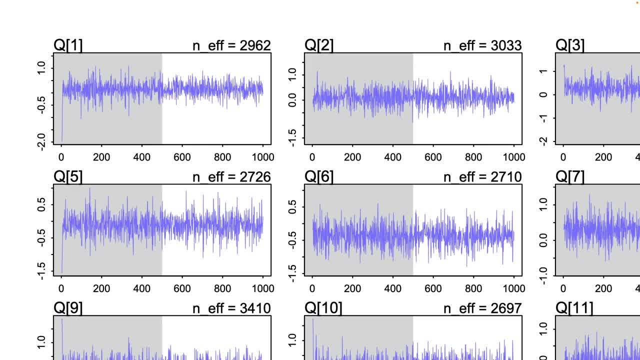 For a good, healthy Markov chain is that it rapidly moves around the whole high probability region of the parameter space, zigzagging a lot Sometimes people say like a fuzzy caterpillar is the idea. It looks like a noise pattern. I'll show you what a bad chain looks like in a moment. 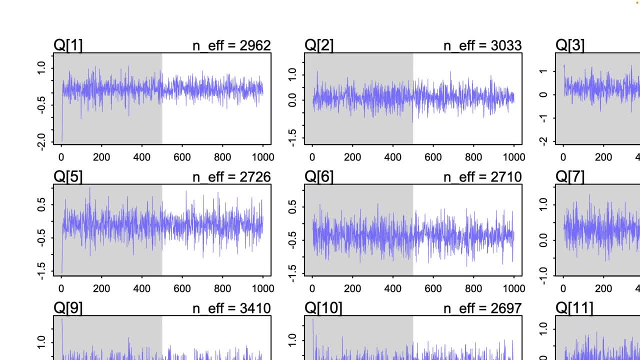 On these graphs. this is the default trace plot for the rethinking package for Ulam. You'll see it also shows NF at the top, the number of effective samples. Bigger numbers are better. I'll talk about that a little bit later. 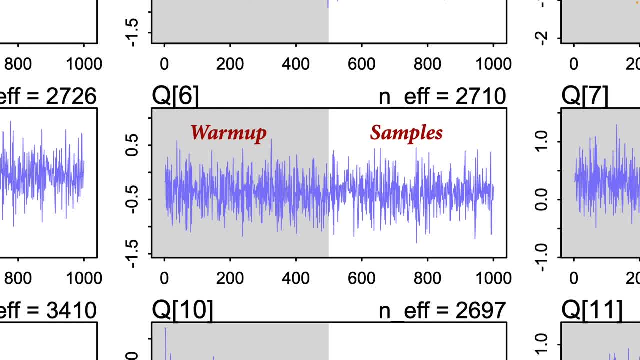 Inside each of these plots you notice there's a gray region and a white region. The gray region is the warm-up region. Those values are not samples from the posterior distribution. When Stan is trying to develop the Markov chain, it spends a lot of time warming up. 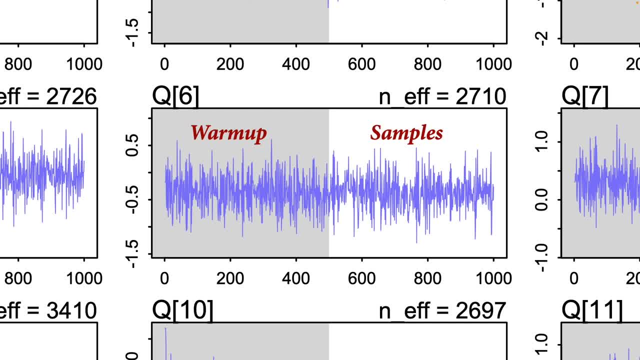 which means it's adapting the step length and the other things I showed you before the break that change the efficiency of the Hamiltonian Monte Carlo. It's nice to visualize these because they give you an idea whether warm-up is effective or not, but it's the samples in the white region that you actually get to work with. 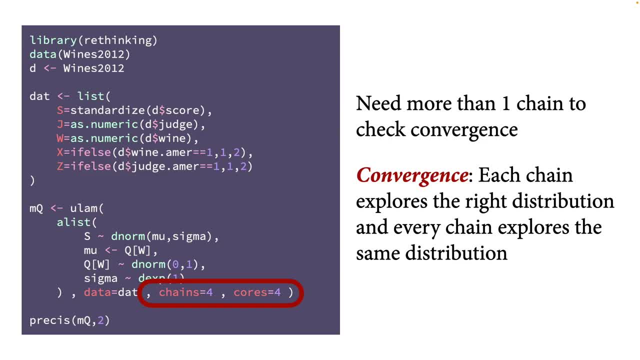 that are valid draws from the posterior distribution. What I just showed you is one chain, that blue hairy caterpillar- but we fit four chains. You usually want to fit more than one chain. You have to, because it's the only way to assess something called convergence. 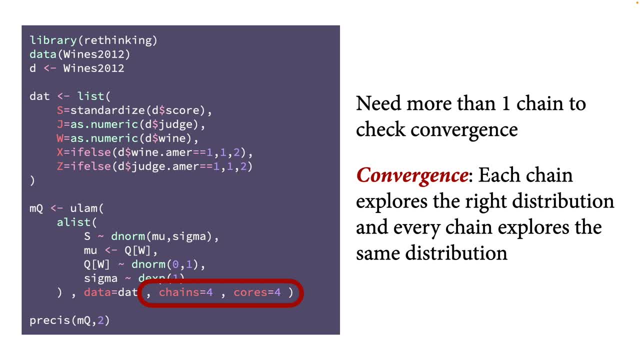 Each Markov chain is initiated from a different chain. It's a different random starting location in the total space of possible parameter values. What you want to see is that from widely dispersed random starting locations that all the chains converge to the same posterior distribution. 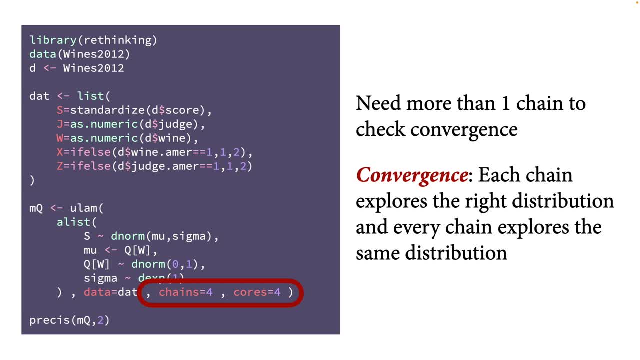 That's what's called convergence. It's that each chain explores the correct distribution and the same distribution. We're going to say chains equal four for four Markov chains. This is optional- but also cores equal four. Your computer almost certainly has between four and eight. 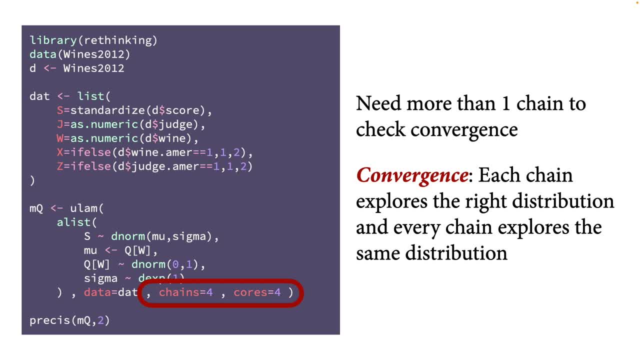 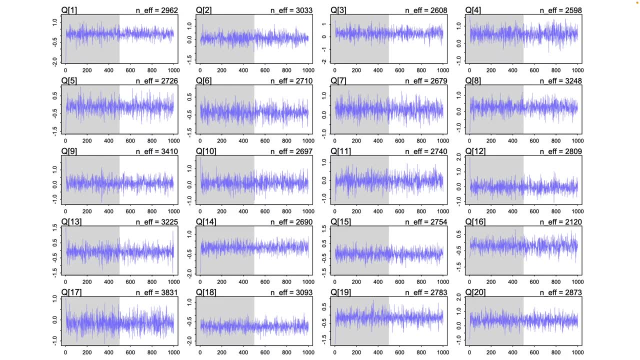 different sub-processors called cores. You can run a parallel Markov chain in each of them. You usually want cores to equal the same number of chains. Let's layer on the other chains. Here's the figure you saw before. Then here's the second chain. 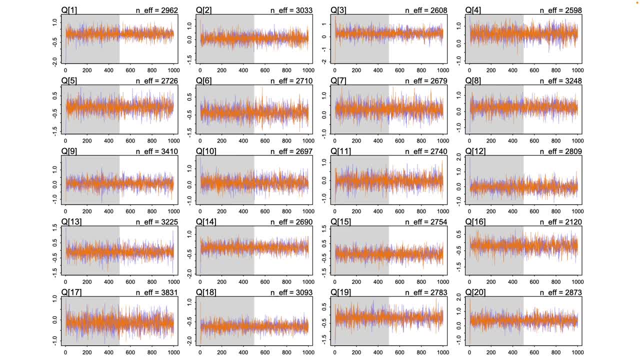 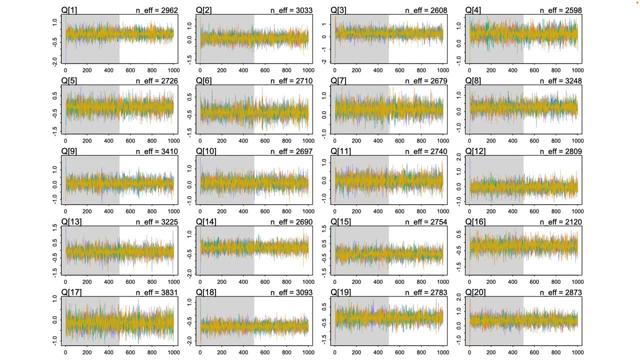 What you want to see is that it overlays. It's exploring the same space as the first chain, Then the other two. Here's four chains all laying on top of one another. Now it really does look like some kind of colorful, hairy caterpillar. 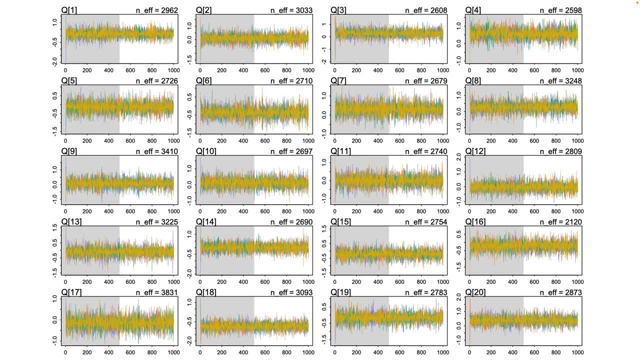 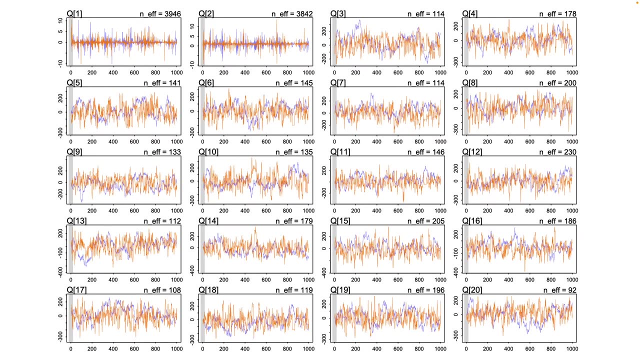 This is what you're looking for with a good, efficient Hamiltonian Monte Carlo chain, is that it looks like this. This isn't a guarantee that it's the correct posterior distribution, but this is what you want to see. This is what a bad chain looks like where it's wandering around. 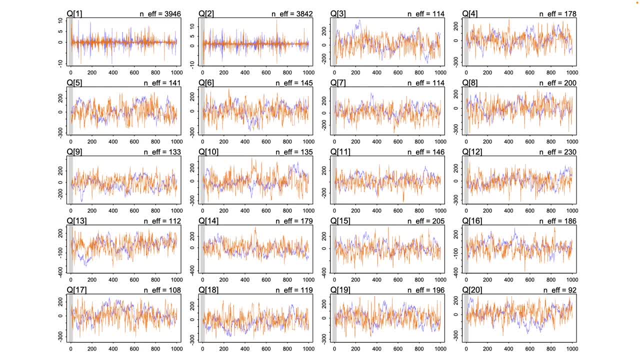 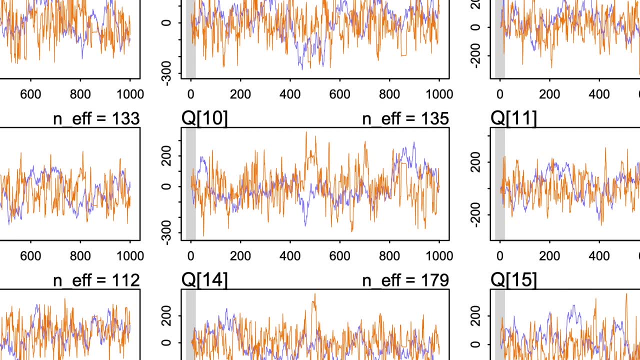 It doesn't look like a hairy caterpillar, or maybe it's a decaying hairy caterpillar. Zoom in on one, You get an idea. You'll see. there's only two chains here and they're not exploring the same space and they wander around the space. 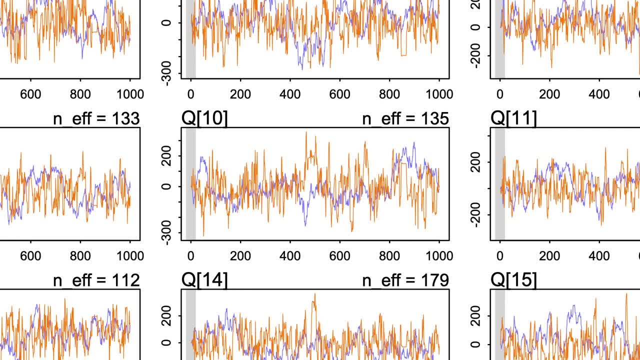 They don't look a fuzzy caterpillar at all. This kind of chain is usually- well it's at least- highly inefficient. This is very inefficient exploration of the posterior distribution. It might also still be valid, Often, with chains that look this bad if you ran them long enough. 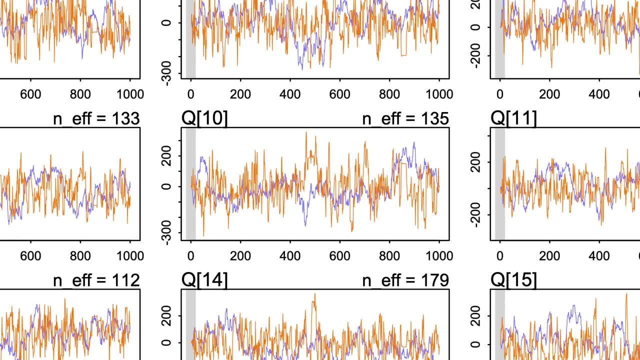 you would still get a valid approximation of the posterior distribution, but we don't want to wait that long. Often with Hamiltonian Monte Carlo chains you only need a couple hundred samples to get a good picture of the posterior distribution, because it explores the distribution so efficiently and quickly. 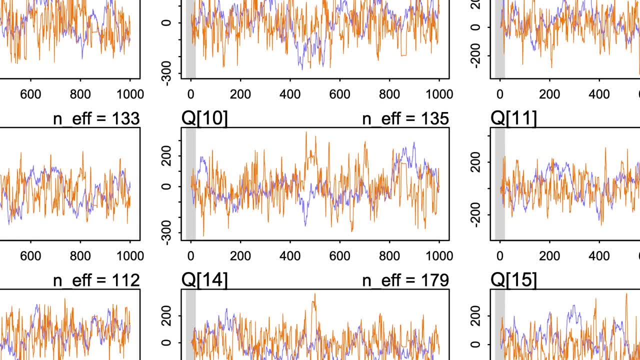 I'll say that again, Often with Hamiltonian Monte Carlo, if it's configured correctly, you only need a couple hundred samples to get a good picture of the posterior distribution. But if your chain looks like this, you need thousands and thousands, and that's why you'll sometimes see, with Bayesian, particularly phylogenetic analyses. 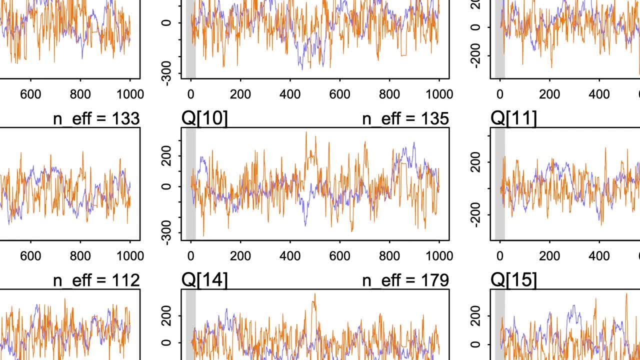 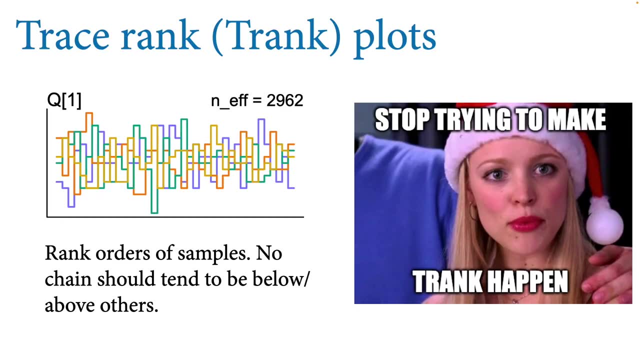 people taking millions of samples, and that's because the Markov chain algorithms in that software is not so good and also nobody knows how to explore tree space, And so they take like five million samples and then pray. We don't pray, We think. 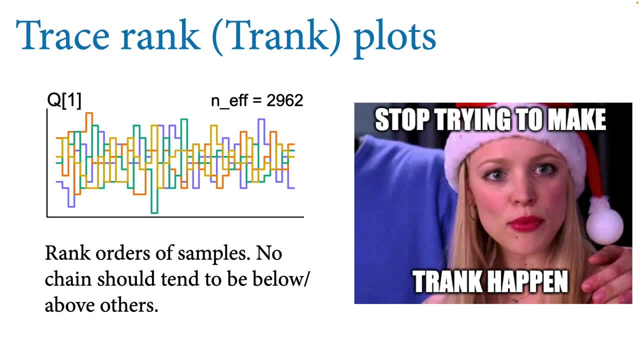 And another diagnostic you can use to look at the quality of your Markov chains is this thing I'm very fond of called trace rank plots. I call them tranq plots. I know nobody else does, but I'm going to keep trying to make tranq happen. 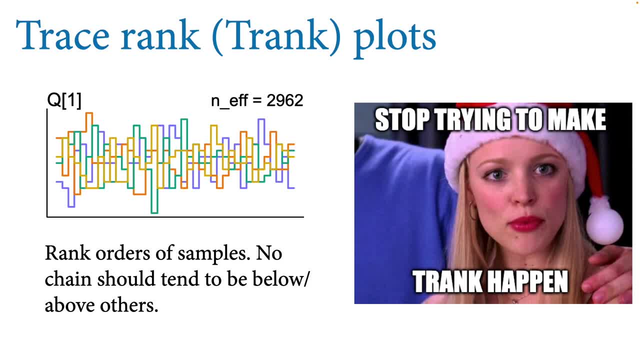 And what a trace rank plot is. it's the same data that goes into making a trace plot- the plots we just looked at- But now we take the rank orders of the samples, not their values. So what you do is you take for any given parameter. 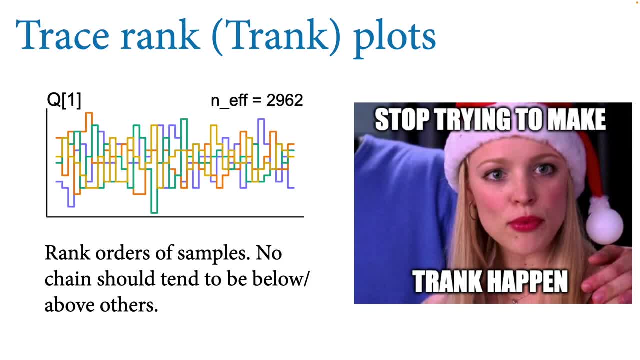 you take all the values from all the chains and then you convert them to rank orders and then you plot histograms of those rank orders for each chain, And that's what you're looking at here. It makes this weird geometric shape, but the point is that the pieces 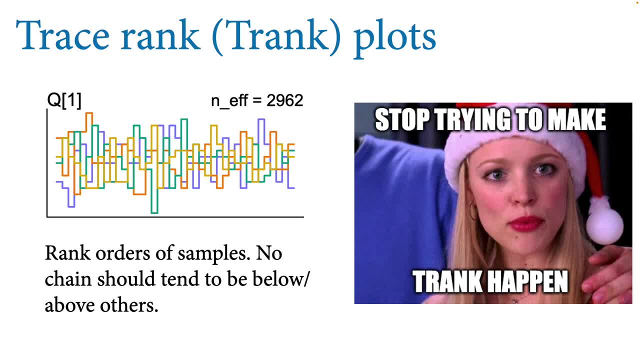 the peaks of those little bars are the peaks of a histogram, And what you want to see is that all the chains are basically in the same place, that they're uniform, so that the rank orders- low ranks and high ranks- are not located within any particular chain. 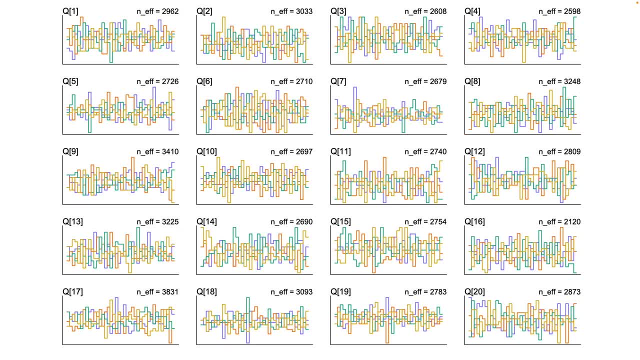 And that's what you want to see. So if it's all jumbled up, that's good. So here's what good is for the model we just ran. Here are the tranq plots for all of the 20 q parameters: the wine quality chains. 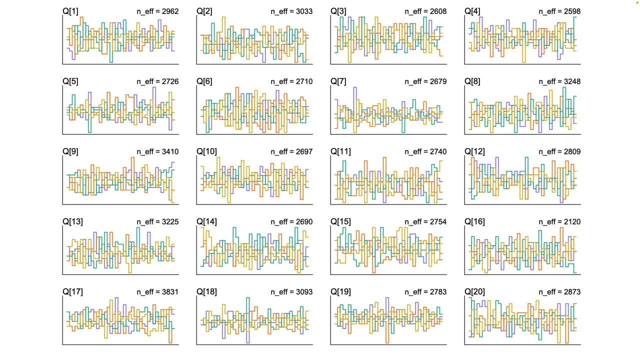 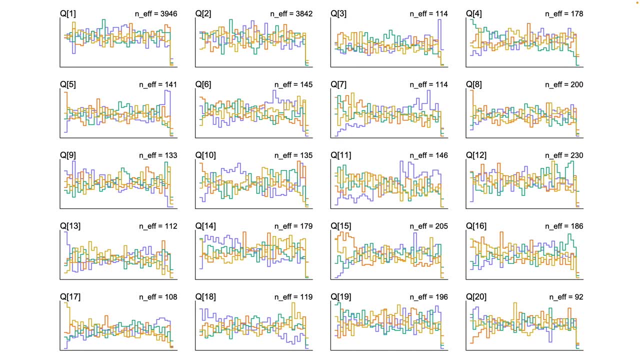 And what you'll see is there's no particular color for these configurations which is consistently above or below the others. This is what it looks like when it's bad, So I messed up the algorithm and reran it, and this is what you get instead. 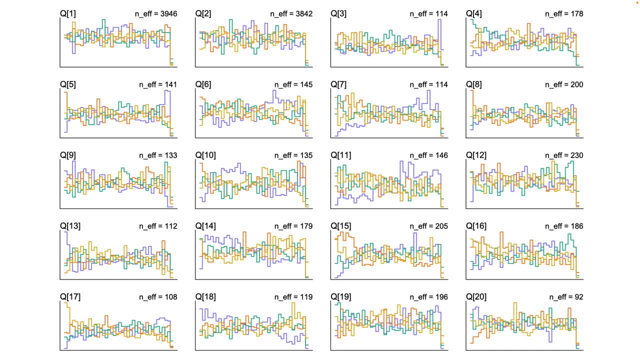 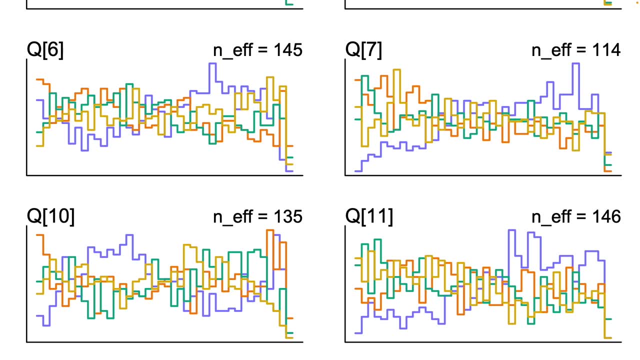 You get this case where it's still jumbled, but it's jumbled in a more sorted way, So we can zoom in and you can see for these in the middle. you'll see that, for example, the blue chain tends to be either above or below the others. 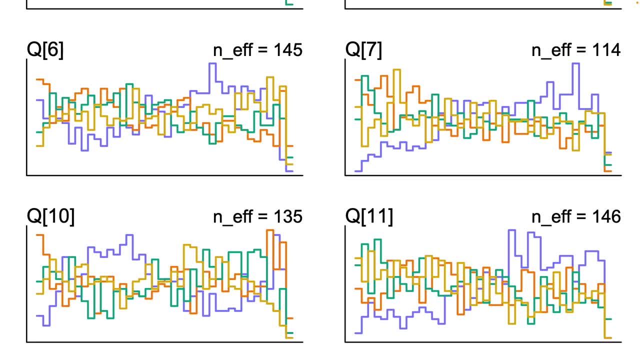 And this indicates poor exploration. Again, if you ran this chain long enough, maybe it would give you a perfectly valid approximation of the posterior distribution, but we'd rather have something that's efficient, because that's much more reassuring. Okay, There are also new numerical things. 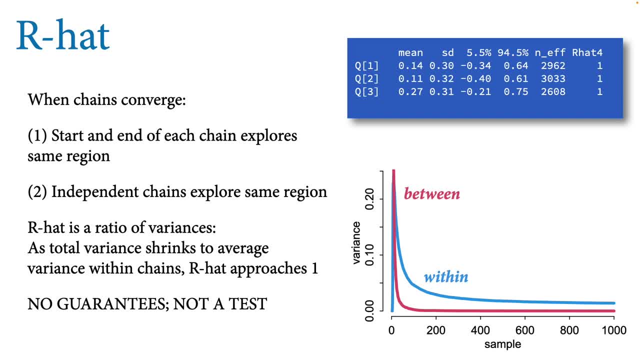 the things that appear in the Precy plot, I mean the Precy table, like R-hat, the most famous of them. R-hat is a chain convergence diagnostic And the way to think about it is, it's like a variance ratio. 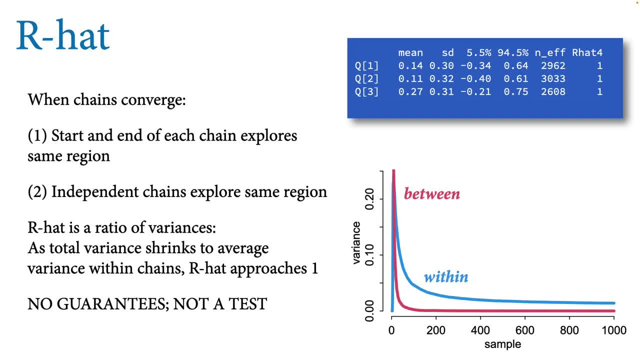 like an F-statistic- those of you who know F-statistics- Here's the idea. So if chains do converge, the beginning of the chain and the end of the chain are exploring the same place. The chain has not wandered into some new territory. 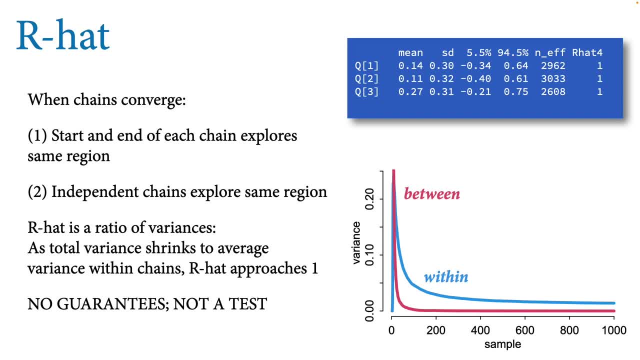 as time goes on, It keeps revisiting where it started. That means the chain is stationary and it's hopefully in the right place. Okay, You also want to see under convergence that the different independent chains are exploring the same place. They're returning to the same places. 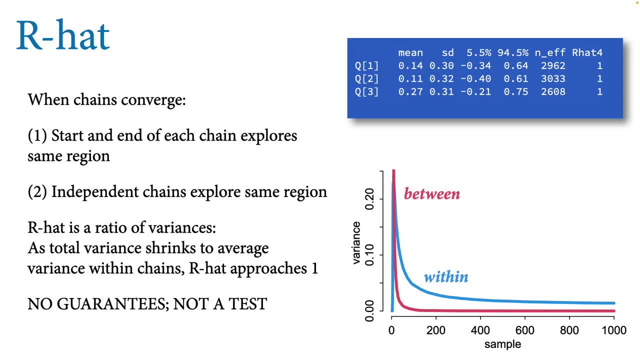 And R-hat is a ratio of variances that assesses these things. So as the total variance shrinks to average variance within chains, R-hat approaches one- I'll say that again- As the total variance that is among all the chains. 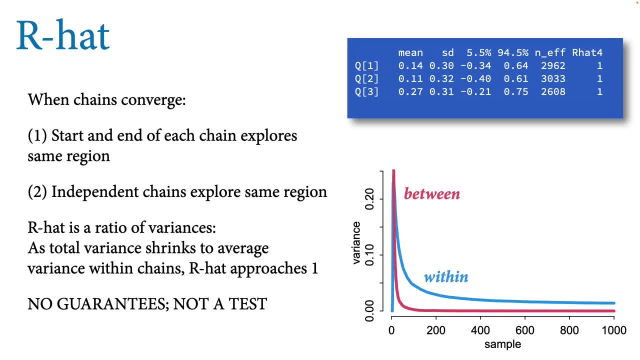 shrinks to be the average variance within chains. R-hat approaches one. If this wasn't true, you'd have the total variance. if the chains are exploring different regions, then the total variance will be bigger than the variance within chains. Yeah, the average variance within chains. 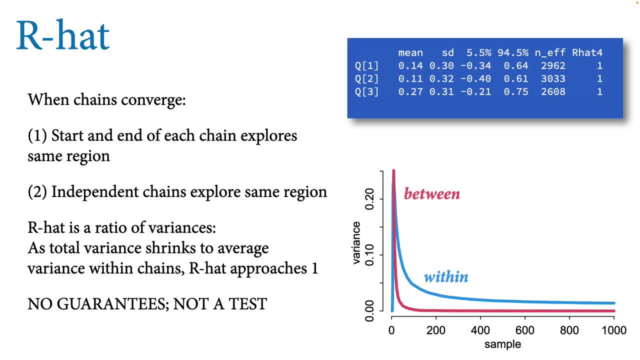 So, if you think about, you look inside one chain and you compute the variance of the samples within that chain. You do that for each chain and then take the average. That's the average variance within chains. It tells you how much chains vary internally. 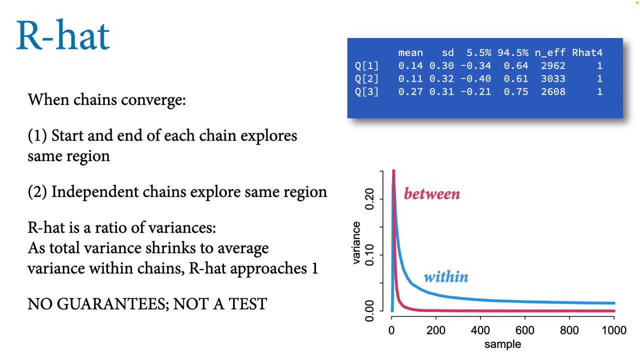 And then you look at the variance across chains. That's the total variance in all the chains. If that ratio approaches one, then that indicates convergence. Now it takes infinity to exactly get to one, But in practice this often happens very quickly for a good functioning chain. 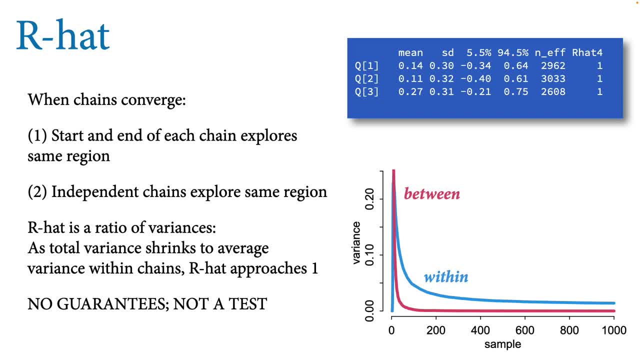 This is not a test. There's no magical value of R-hat which guarantees convergence. It just isn't. But if it's a big number- over 1.1 or 1.2, you might need to at least run the chain longer. 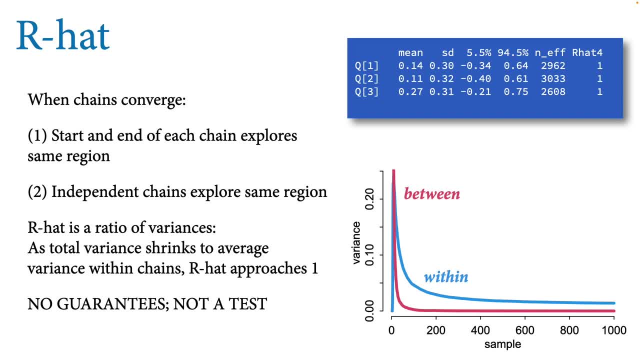 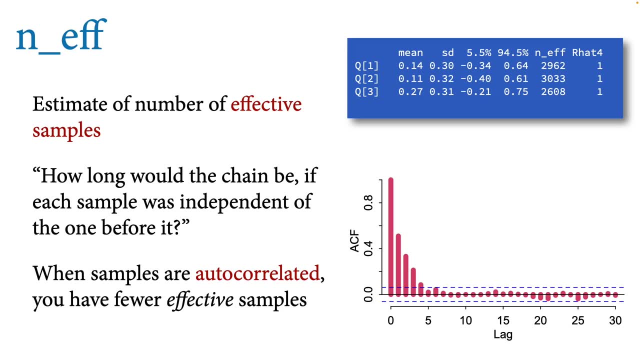 But you might also want to do some fiddling to make things more effective, or maybe there's a real serious problem. The other thing you'll see in these tables is nf- the number of effective samples- And people call this slightly different names all the time. 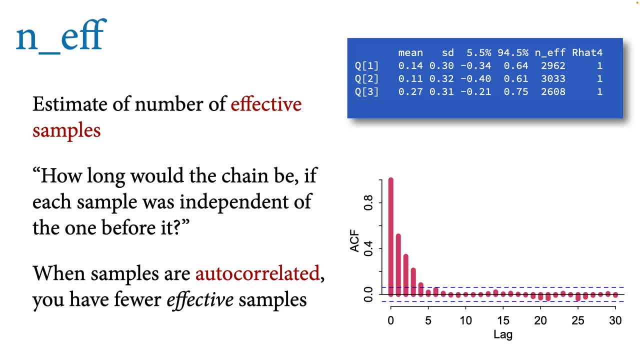 and have opinions about that effective sample size and so on. What you want to take away from this is the idea that this is an approximation of how long the chain would be if each sequential sample was completely independent of the one before it. So let me say that again. 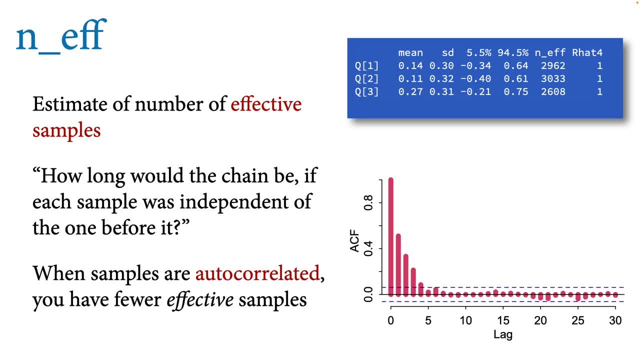 You ran a Markov chain and say it was 2,000 samples long. Okay, And then the nf is: Well, let me do the real example. So we ran four chains here and got 4,000 samples and say the nf for Q1 is 2,962.. 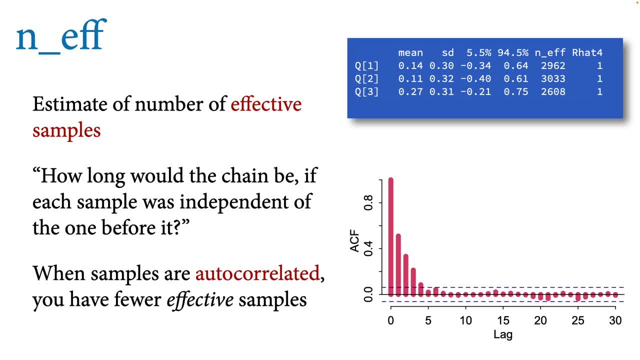 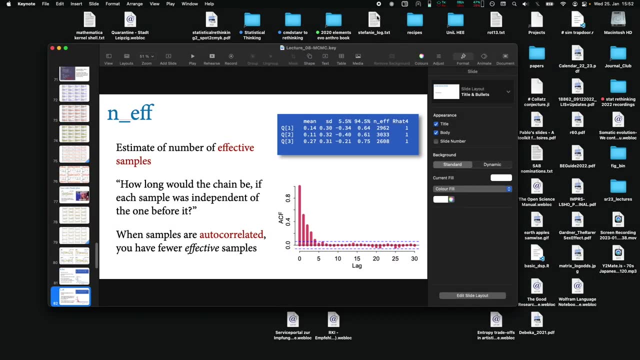 Okay, So what that's saying is approximately: this isn't a promise, right, It's a guide. an approximation is that there's as much as information in any. Oh sorry, I've done this all the wrong way. I got to do that. 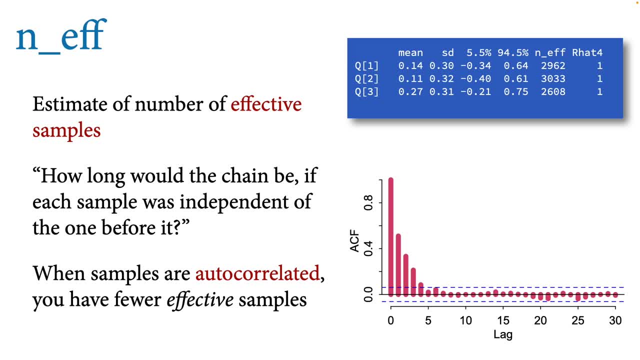 Okay. The other numerical diagnostic you're going to see in the Precy table output is this thing: nf. I call this the number of effective samples. Some people call it effective sample size. What you want to take away from this is that this is an approximation. 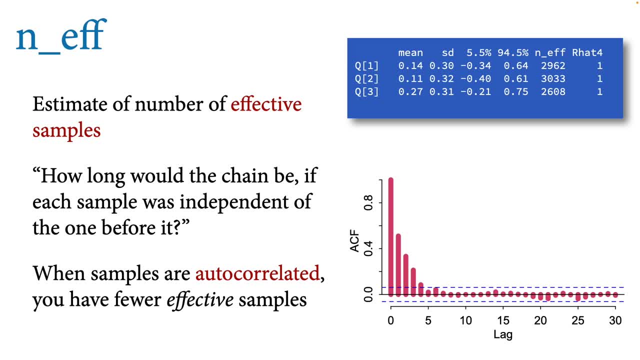 that says how long, how much information you've really got in your samples And it gives you that measure of how much information in terms of a counterfactual, of how long the Markov chain would be if it were in some sense perfect. 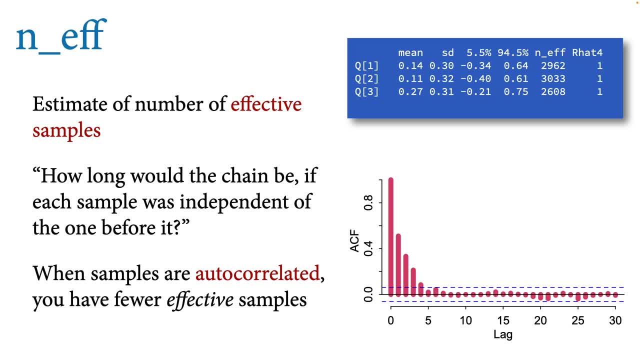 perfectly uncorrelated, That is, sequential samples were totally independent samples from the posterior distribution, as if you had simply used a perfect random number generator. So, for example, if you wanted to simulate Gaussian draws in R, you would simply use R norm and every draw from R norm. 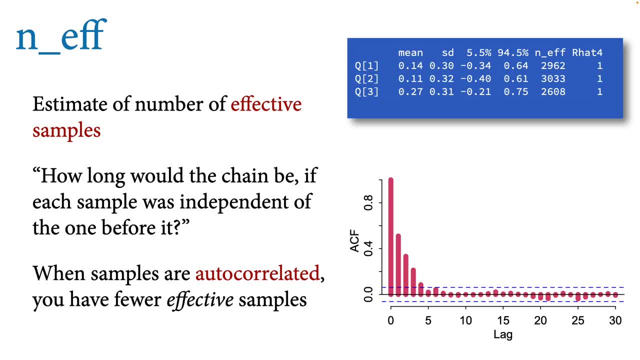 is independent of the one before it. Okay, So in some sense that's your ideal efficient Markov chain. Yeah, Your chains won't be that good usually, But if we can assess how long the chain would be for the information you've got, 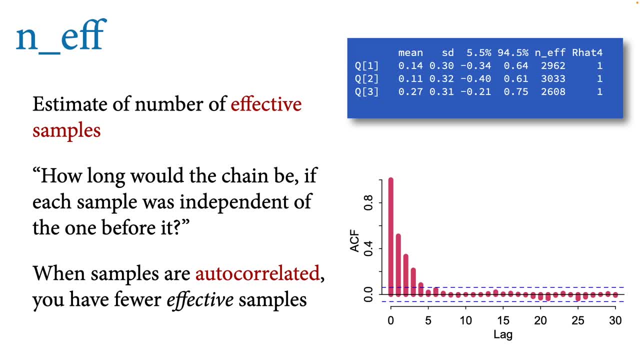 in your actual samples that you drew, which are correlated sequentially with one another. how long, effectively, is your chain from a shorter? So typically, nf is smaller than the number of samples you actually took, because the perfect chain will need fewer samples. I'll say that again. 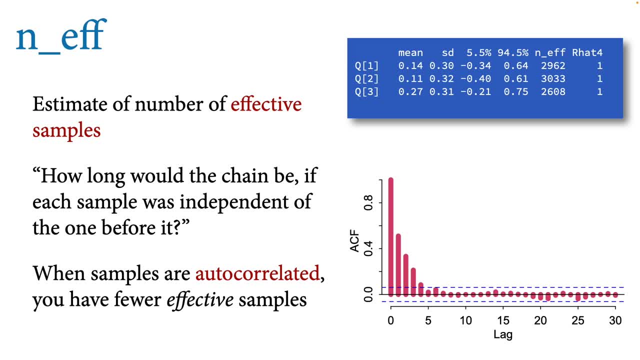 Typically nf is going to be smaller than the number of samples you actually took, because the perfect chain will be shorter. wouldn't have had to run as long to get the same amount of information as you got in your more correlated chain. So when samples are autocorrelated, 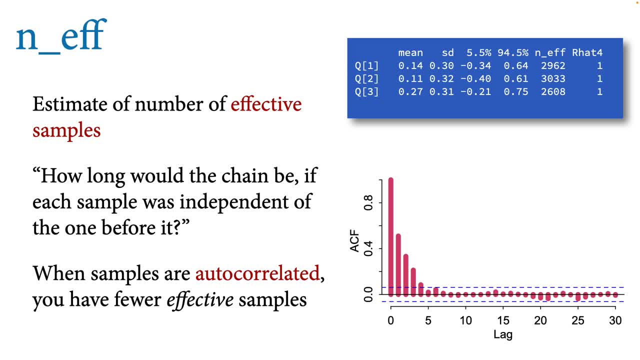 you end up with fewer effective samples because the sequential samples share information with one another, They're not independent draws. There's this thing called the ACF or autocorrelation function, And you can just dump Markov chain samples into this and get an assessment, like I have here. 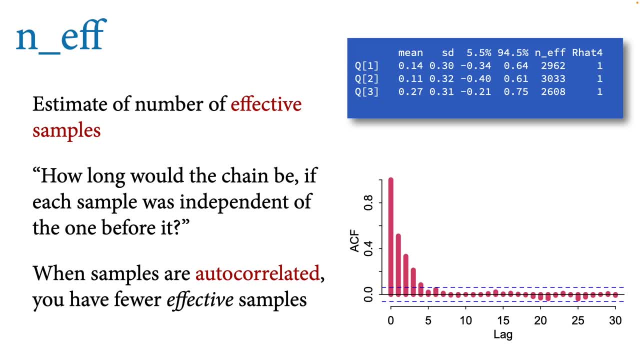 of the autocorrelation, of sequential ones, And so typically there's always some local autocorrelation, like you see here that going from zero, which is any particular sample, and moving back in time, they're similar but it fades very quickly. 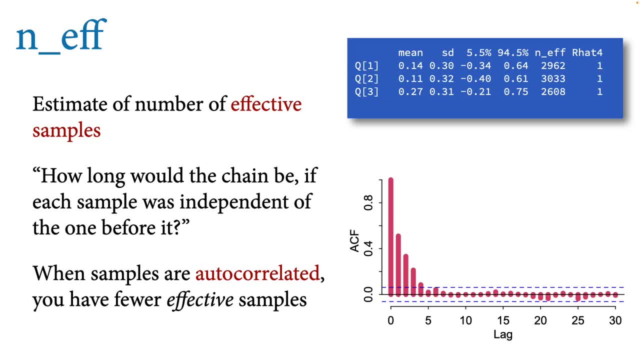 It is possible for some Markov chains for the effective number of samples to be bigger actually than the number of samples you took, And that's because sometimes Stan is so clever and Hamiltonian, Monte Carlo is so efficient that it does better than completely random and independent. 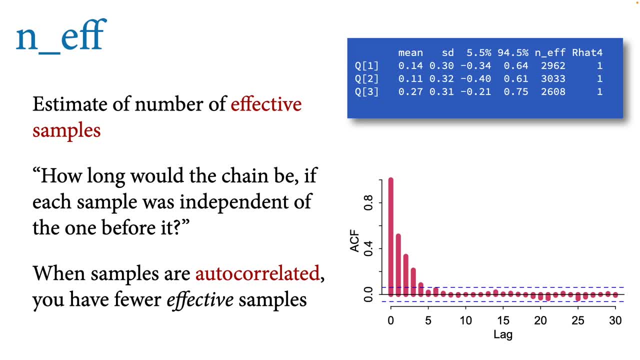 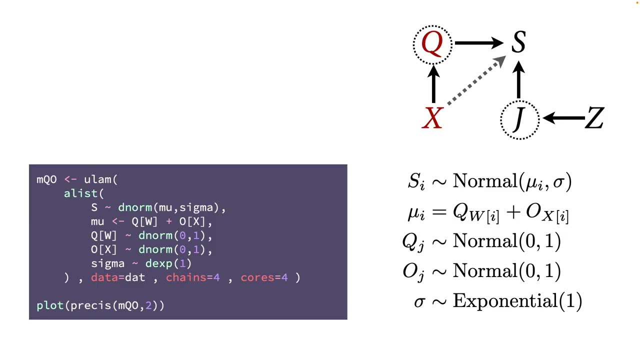 It finds dispersed parts of the posterior distribution which are better than independent of one another, so it can explore even faster. That's an amazing thing. So when you do see that, if you do see it, it's not a bug. Okay, Let's come back to our model. 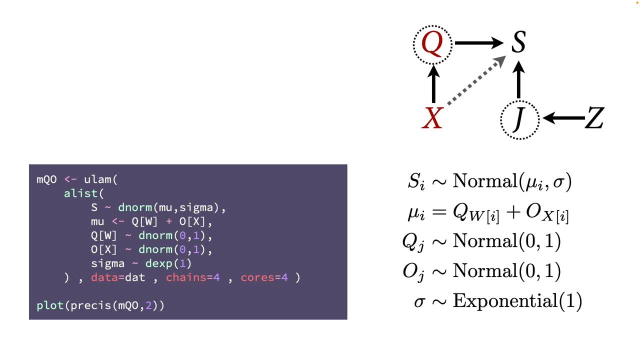 We need to add, we need to stratify by the origin of the wine, this X variable, which is an index saying whether a wine is from New Jersey or from France, And we're going to do the simplest form of stratification here. 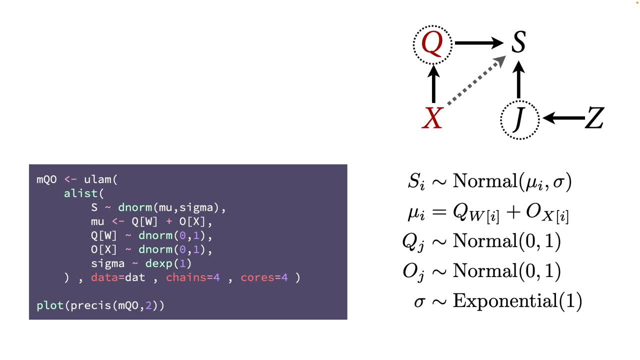 I'm going to add an offset O of X, where O is a parameter. There's one for New Jersey and there's one for France. That is an offset. how much better, on average, wines from that origin are Okay, And you can think of this as a mean. 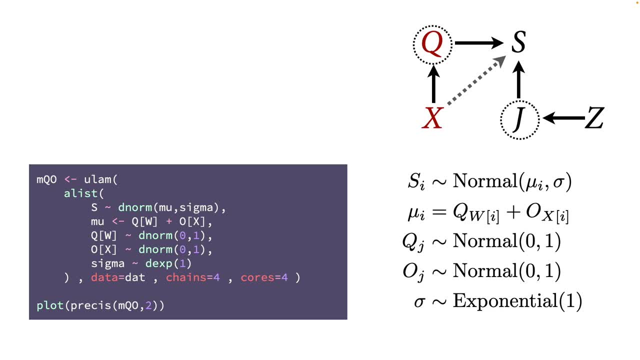 and then each of the cues is an offset from each nation's mean And I'll again assign this normal 01 prior. We can look at the plot, the PRACY output this time, and make one of these caterpillar plots and make. we got a lot of parameters. 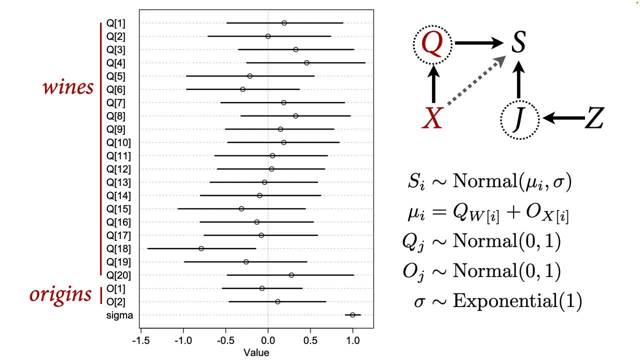 might make more sense. See all those cues. those are the wine qualities. You can see the wines definitely do vary on average, particularly in wine number 18, not so great, I don't know that people didn't like that one. Some of the others get higher ratings. 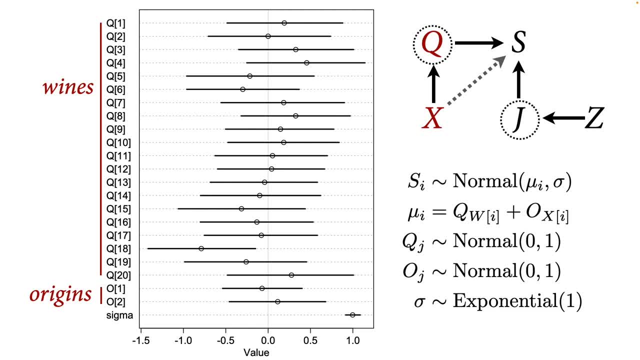 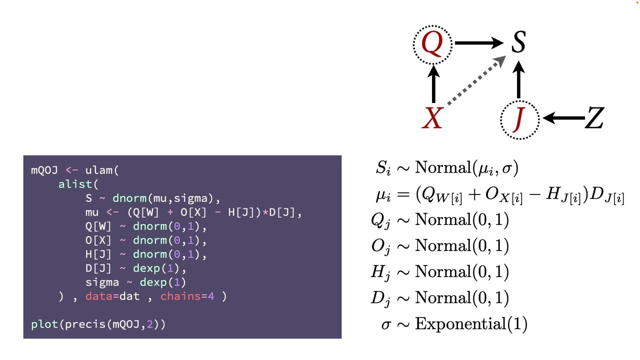 And then the two origin parameters down there at the bottom. their posterior distributions don't differ very much. There's not much evidence here that, on average, New Jersey wine is worse than French wine. Last step: now we're really going to make this into a fully grown up item. response. 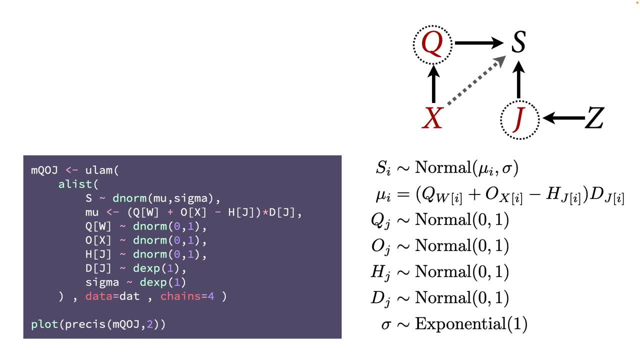 kind of model or judge model. What I want to do now is introduce judge effects. So judges vary in how picky they are, both how hard they are on wines and how discriminating. So we're adding two parameters in here, and I know that I've modified the mu line. 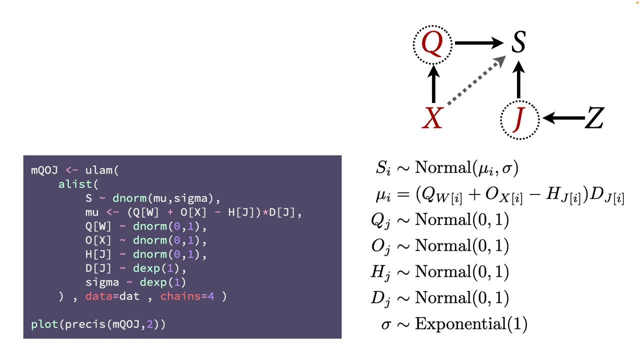 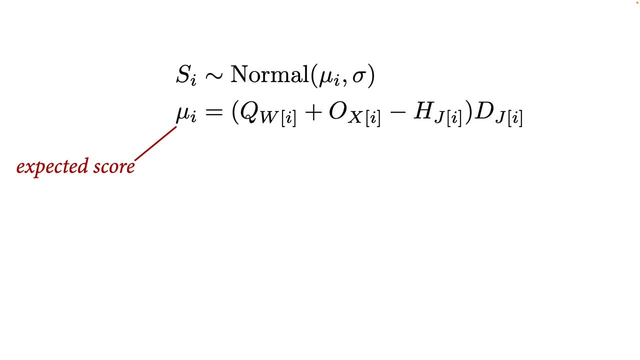 both in the mathematical version of this model and in the code, And I've added two new vectors of parameters H and D. It takes a little bit of time to explain these by zooming in on the mathematical version of the model. We can talk about it. 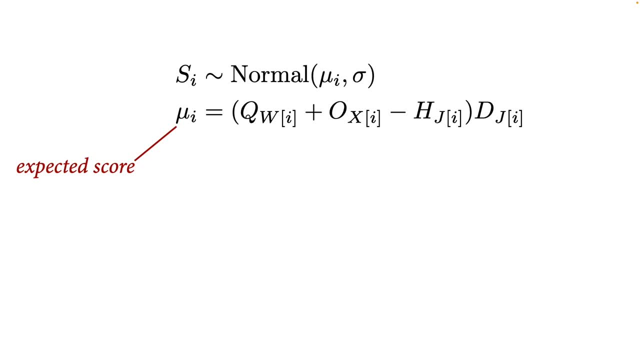 So the line for mu just defines the expected value of a score for any given combination of the predictor variables. As always, the Q parameters are wine quality, as we've seen before, And the O parameters are the origin offsets, And these are the two I've just added. 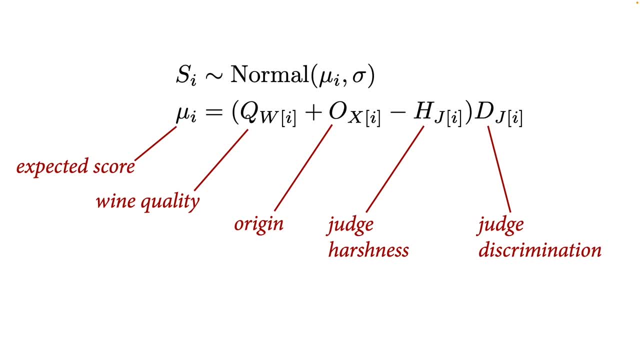 The first is H. This is a judge's harshness, Each judge J, so H sub J of I is the judge on row I. It has an H parameter and this H parameter indicates harshness, the harshness of a judge. What does harshness mean? 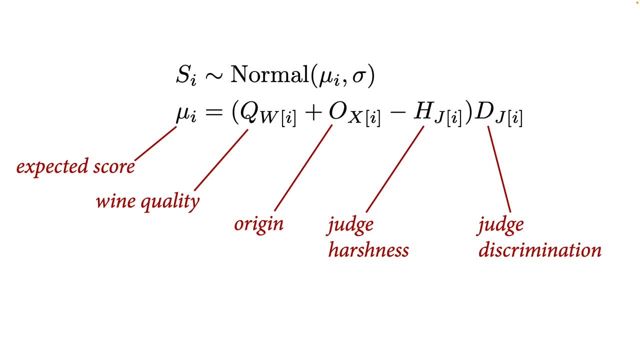 You'll notice, it's being subtracted from the quality of the wine and the origin offset. What that means is the harshness is how good a wine needs to be for this judge to rate it as average. I'll say that again: The harshness is how good the wine needs to be. 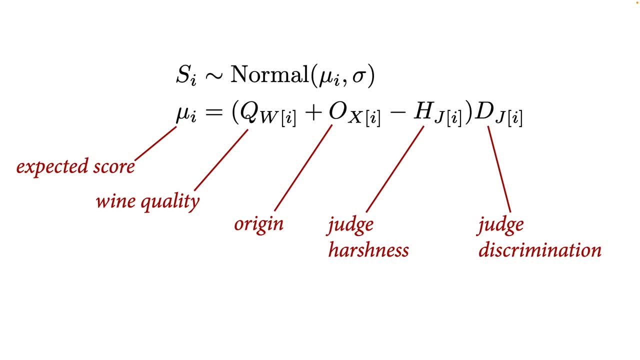 for this judge to rate it as average. So say, a wine had quality 2 on this latent scale. If a judge has a harshness of 2, that means it essentially subtracts two points from the wine, And so a wine of quality 2. 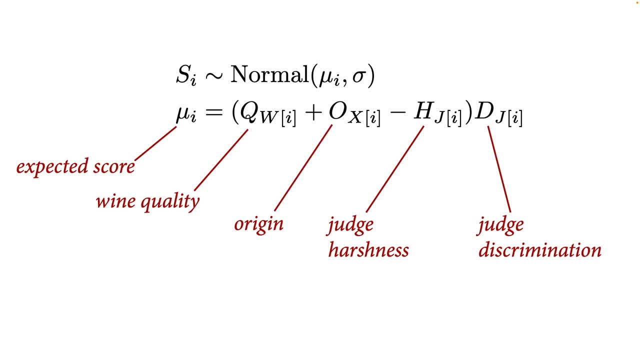 would be rated only as average, And a wine of quality 3 would be rated as quality 1, and so on. Judges can also have negative harshness right, And they can like everything and give everything the maximum score. And then all of that stuff is in parentheses. 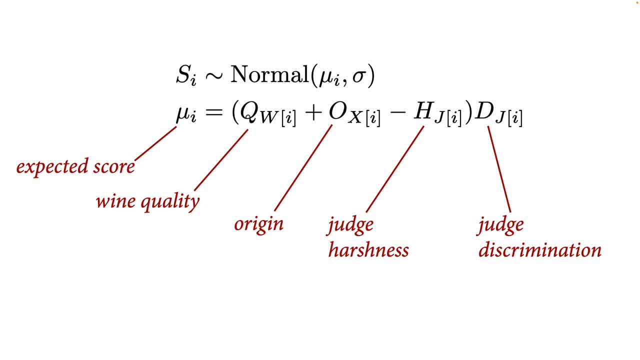 And so it's that sum, and the difference between the quality of the wine and the harshness of a judge is multiplied by this thing. d? d is a parameter, again specific to each judge, that measures the judge's discrimination. And what does that mean? Well, some judges make a big deal out of small differences in quality and give really dispersed scores to wines that are even a little bit different. Those are discriminating judges. Other judges are not very discriminating and they tend to give even quite different wines similar scores. 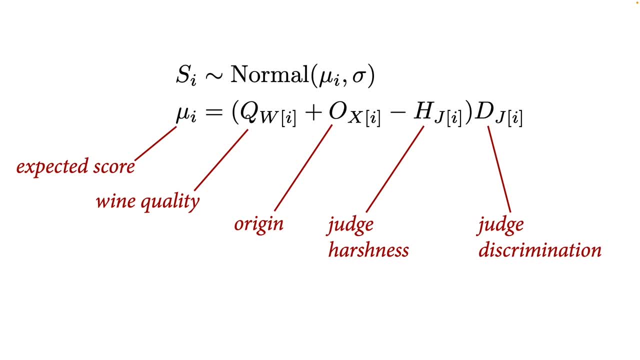 And that's what d does here, Since it multiplies the difference, It either magnifies. for big values of d, it magnifies the difference and results in a bigger score or a smaller score, as the case may be, And for small values of d, 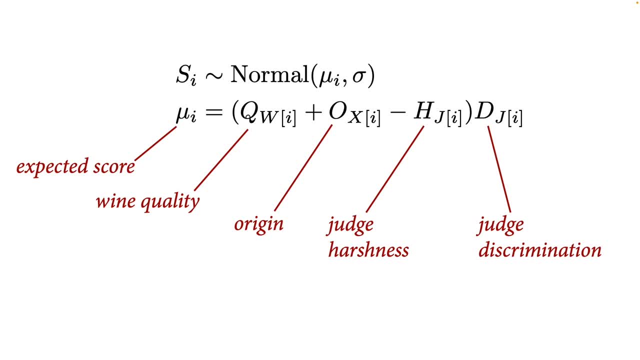 and the limit 0, which is the lowest d can get. a judge with a discrimination value of 0 assigns all wines to be average. I'll say that again: A judge with discrimination value 0 assigns all wines to be average. Yeah, 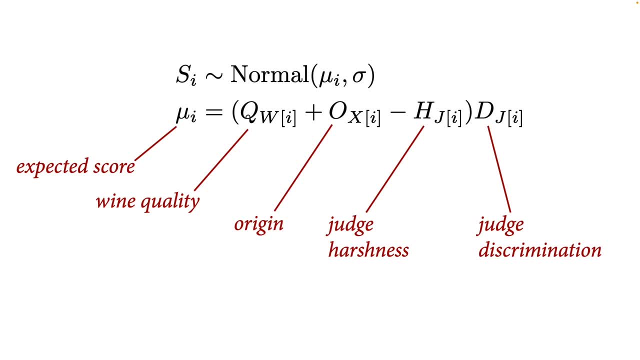 And we all know someone like that. So, but these are professional judges. They make discrimination, But still they can vary in their discrimination And this structure that you're seeing on the slide- this is a very common way to do- a judge model. 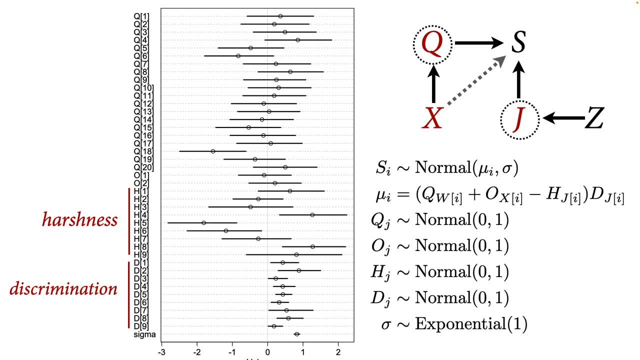 or an item response model. Okay, And the idea we go through this extra machinery of the harshness and discrimination parameters because the judge's biases are a competing cause of the score And if we can model those things we can get more precision. 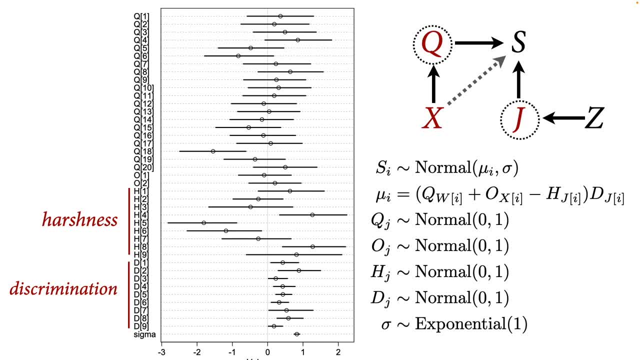 in estimating quality. So we run this model Again. I put some normal 0-1 priors on harshness and discrimination. In a few weeks I'll show you we can do better than these priors, but I don't want to overload you today. 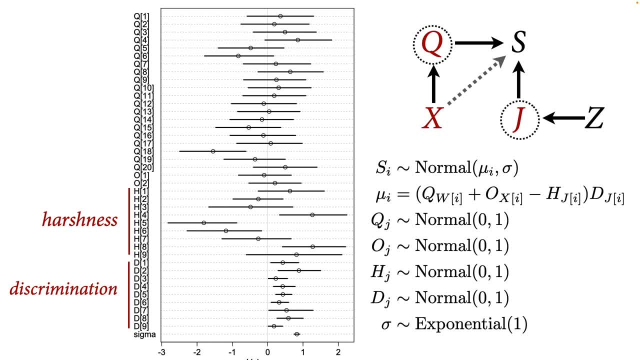 And then I show you the pricey plot on the left-hand part of this slide, Again, all the cues at the top, all the wine quality estimates. Again you see wine 18 there below 0, deep underwater And I think that's a New Jersey red. 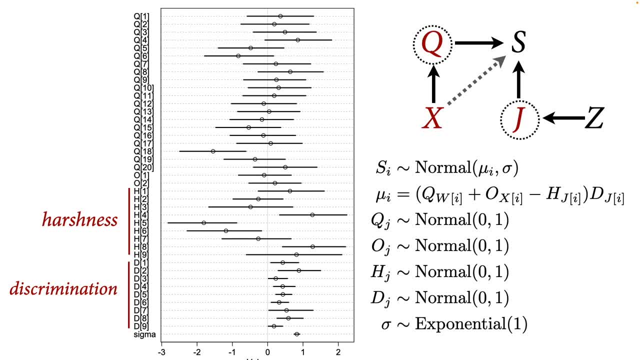 actually, but most of the New Jersey wines are just all in the mix and indistinguishable from the French wines. And then you see the judge parameters- at the bottom the harshness parameters marked H- And you'll see that those vary quite a lot. 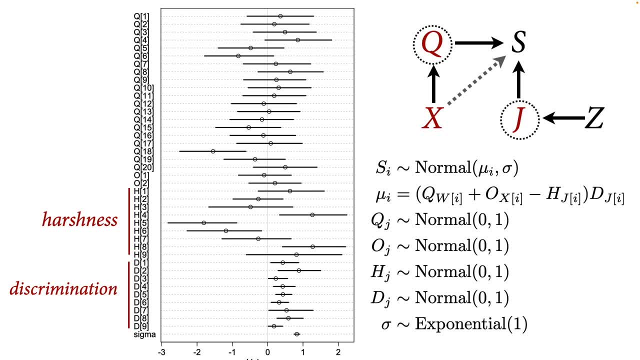 The judges really are very different from one another. Judge 4,, for example, is very harsh. It's a positive harshness value. Judge 4 gave lower ratings than the other judges on average. Judge 5 and 6 are the flip side. 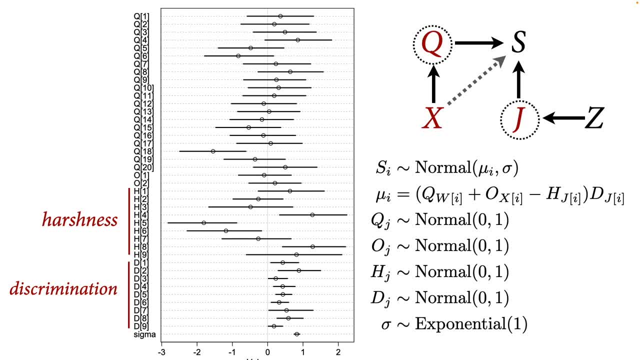 They're, you know they're easier judges. They tend to give higher scores to other things. And then Judge 8 again is quite harsh, And then the discrimination values also vary. They vary less than the harshness estimates as well, But some judges 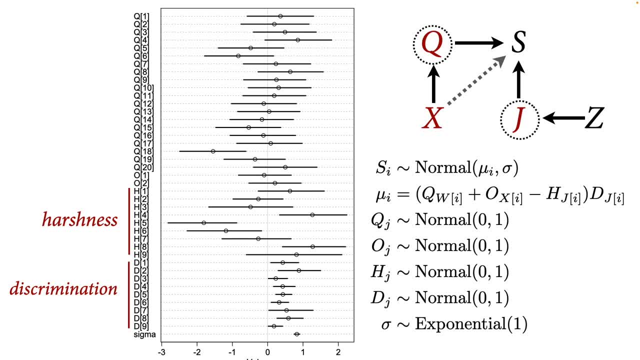 particularly Judge 9, are not nearly as discriminating as some of the others. particularly Judge 2 is very discriminating And their scores vary more. They score the different wines much more differently from one another than the other judges did, Including those effects. 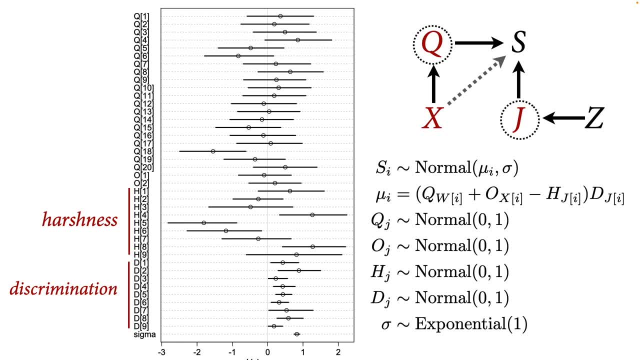 again, we didn't go into this caring about the judges and their personalities, But since this is a competing cause of the score, the idea is we get better estimates of the underlying latent quality of the wine if we can deal with the features of the judges. 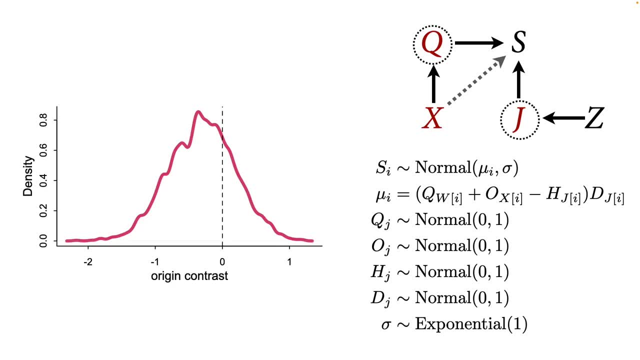 Finally, here's the posterior distribution of the contrast between the average New Jersey wine and the average French wine, And there's a lot of probability both above and below. Knowing a wine is from New Jersey makes hardly any difference In your expectations of how good it is. 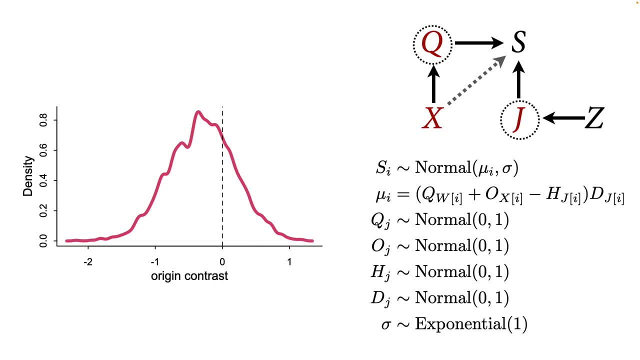 at least for really good top shelf wine. When this judgment at Princeton was done and the results were released, many of the French judges were deeply embarrassed by the results that they did not know And they rated New Jersey wines as equal to some of the best French wines. 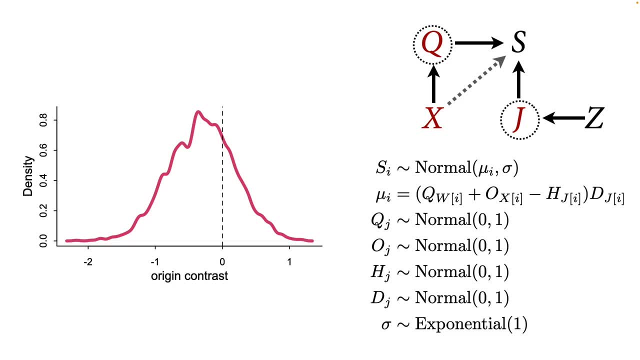 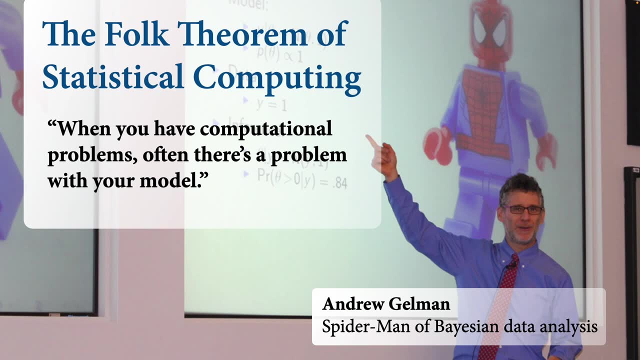 But that's how it is. It's a brave new world. Okay, I'm going to wrap up this lecture. I know there's been a lot here. When we start using more complicated models and Markov chains, it's routine to have problems. 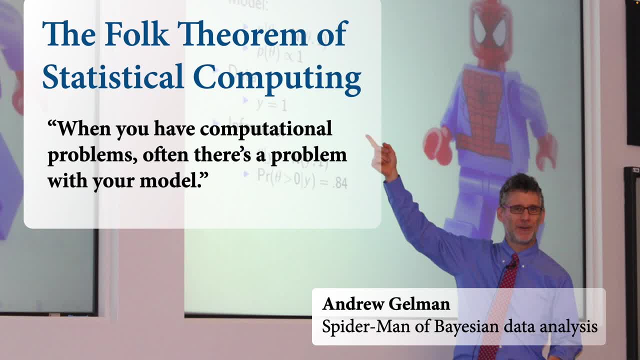 getting the chain to work at first, But we work through it and you get better at it and you fix it. And what I want you to understand is that often the chain is not working not because of some technical issue or some problem with your computer. 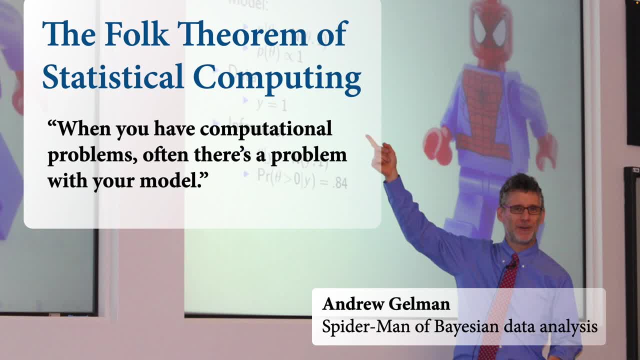 or even with you. It's a problem with your model, That is, there's something about the scientific design of your model which is bad, But we've missed it, either because of a mistake or because we didn't think deeply enough about the relationships between the variables. 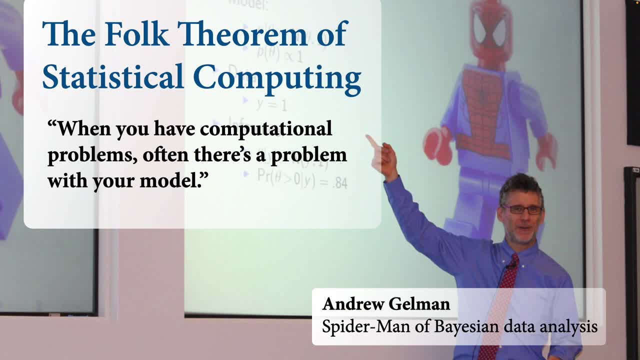 And so it's good, when you're having malfunctioning software, to loop back to your basic scientific questions as well, or assumptions, because those are reflected in the model And it may be that the posterior distribution is having trouble sampling because it doesn't make any sense. 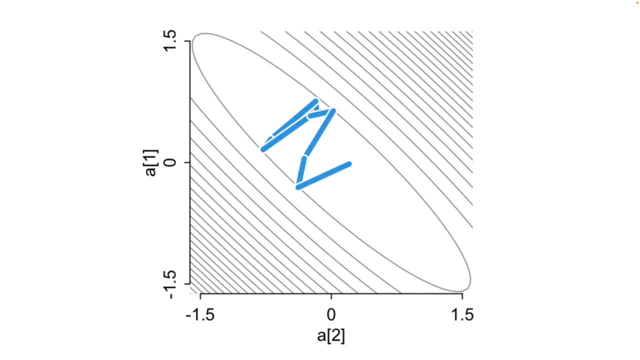 And one of the signs of that is this thing called a divergent transition. Divergent transitions are rejected proposals for Hamiltonian Monte Carlo. Now remember Metropolis. the Metropolis algorithm- or the Rosenbruth algorithm, we should call it- makes proposals and rejects a lot of them. 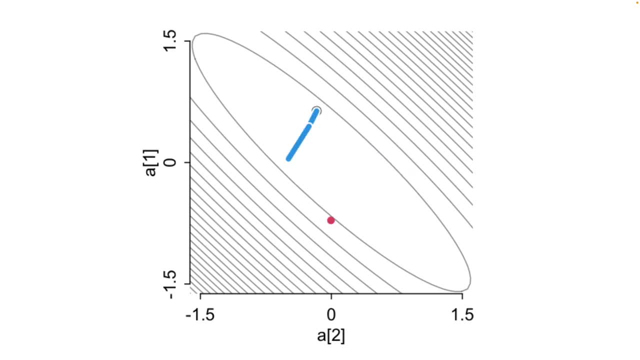 In fact, in many cases most proposals are rejected. But Hamiltonian Monte Carlo is efficient. It doesn't need to run nearly as long because typically nearly all of its proposals are accepted, because they're always within high probability space, because they're rolling around the surface. 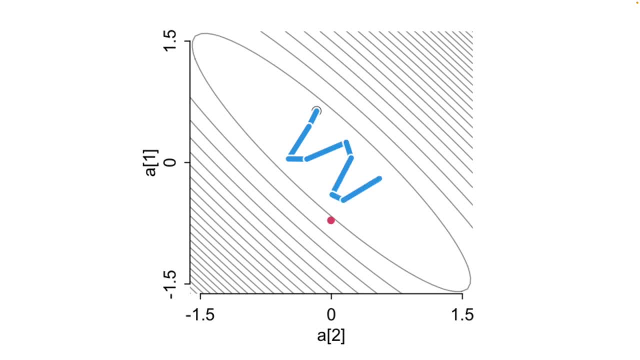 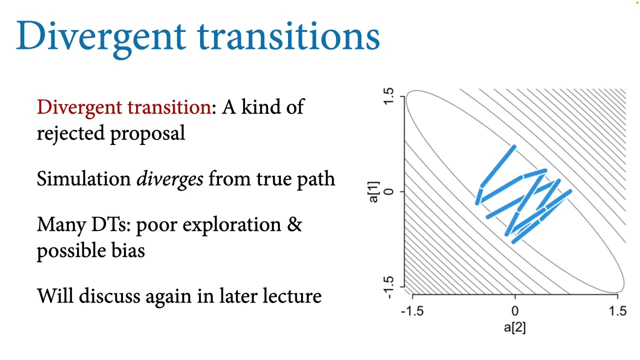 of the posterior distribution. But sometimes they get rejected And in this animation I'm showing you the red samples are rejected proposals and these are called divergent transitions And they happen And they don't mean necessarily that anything's broken. But if you're getting a lot of them, 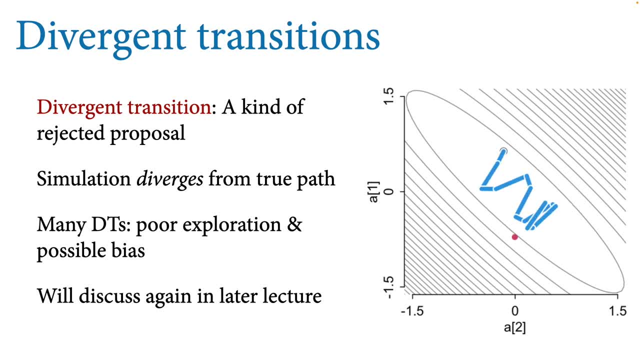 then the chain is exploring the space of the posterior distribution inefficiently and it may be missing, completely missing some regions of it, and that could result in biased evidence, In biased estimates for some of your unknowns, And so you usually want to work to get rid of divergences. 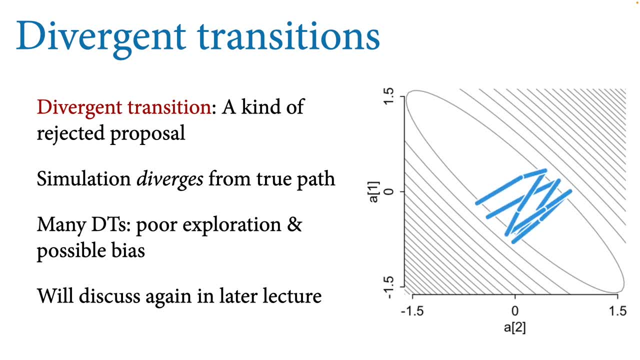 Remember, they're just rejected samples and when Metropolis runs, it rejects most of them, So there's nothing about rejecting a proposal that means the chain is bad. It's just for Hamiltonian, since it can typically accept all of its proposals when it rejects any of them. 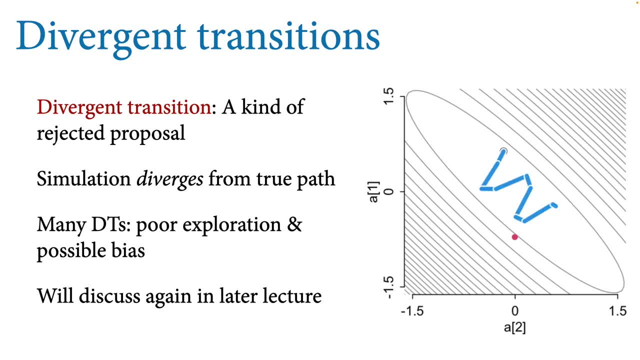 it's a bit alarming And it usually indicates there's something inefficient about it and we can address it. In the book I show you some examples of bad models that generate a bunch of divergent transitions and how to address those. Some of the more common causes of them. 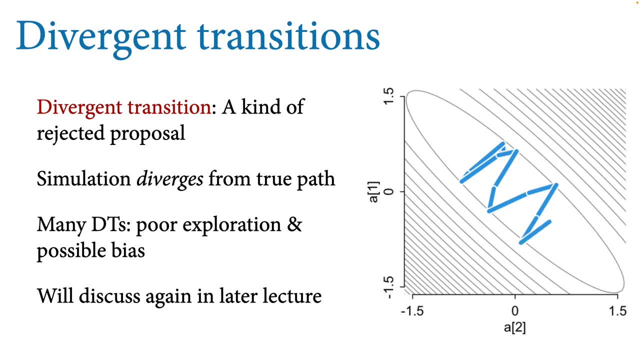 Often it's unrealistically flat priors. But in a later lecture, when we start doing hierarchical models, multilevel models, we're going to talk much more about divergent transitions, because they're much more common and they can do real damage. So just put a bookmark in that. 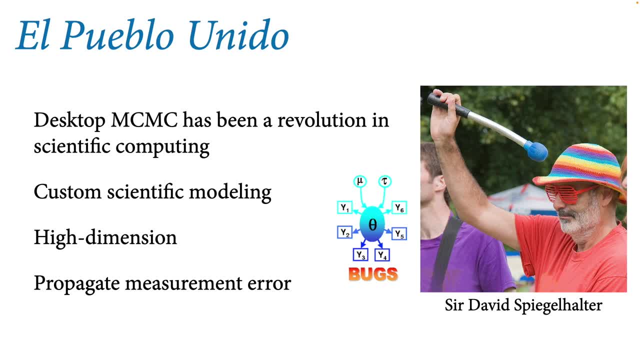 and we'll worry about it later. Okay, I want to sum up here. So, really, the the rise of Bayesian data analysis- applied Bayesian data analysis- in the late 20th and now early 21st centuries has been because of an innovation. 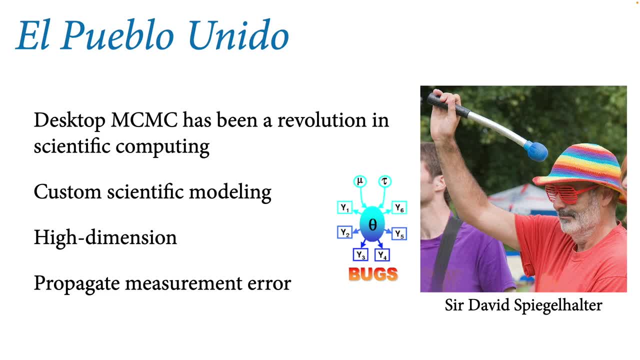 in software and desktop computing. This kind of software, like STAN, was really pioneered by a project called the BUGS project. BUGS is an acronym. It says for Bayesian analysis using Gibbs sampling. Gibbs sampling is like a variant of the Metropolis algorithm. 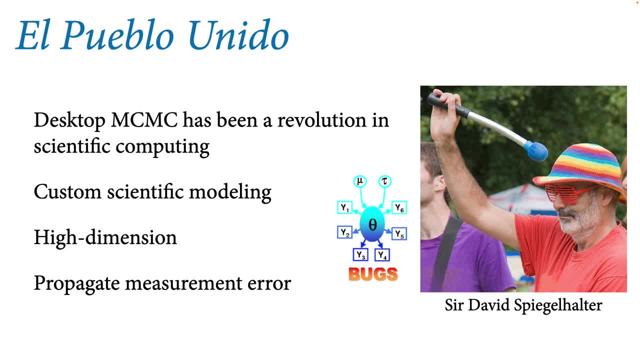 or the Rosenbluth algorithm, I should say. And a key member in this group is the fellow whose picture is on the right, Sir David Spiegelhalter. He was a well-known British statistician And the BUGS project really catalyzed a tremendous amount. 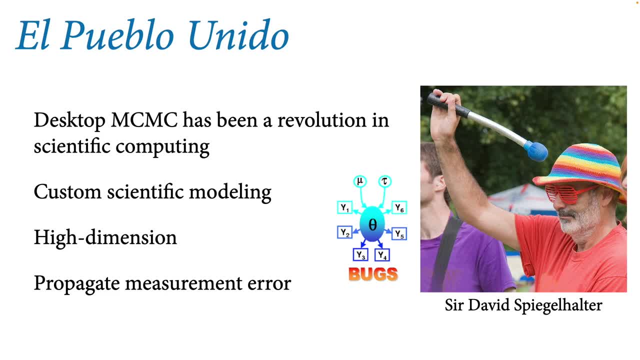 of scientific computing and development and algorithms and really sparked a revolution in allowing scientists to bypass a captive statistician and directly program and express their scientific models and draw samples from the posterior distributions of them. And this has been an amazing thing in the sciences, especially in biology. 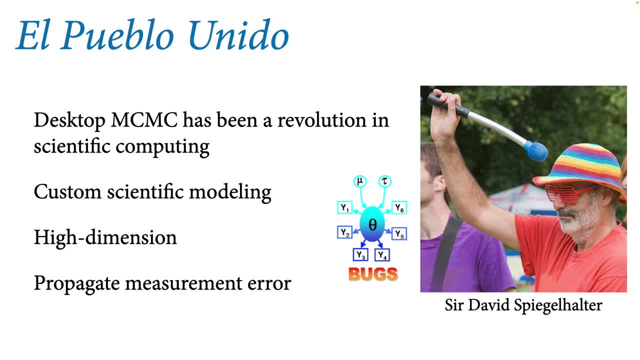 but in all the sciences, And it also allows us to do things that we always knew we should be doing, like propagating measurement error, but had no effective way to do, And so, as we go forward in this course, I'll show you how to do that as well. 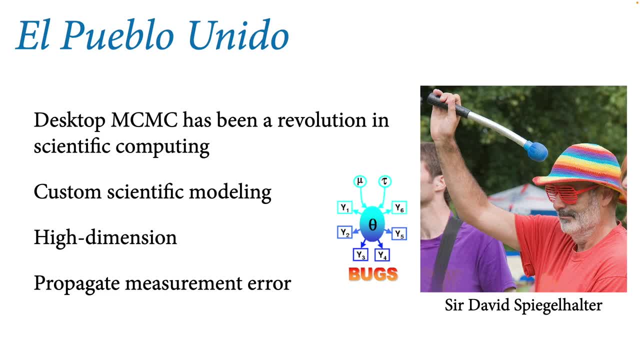 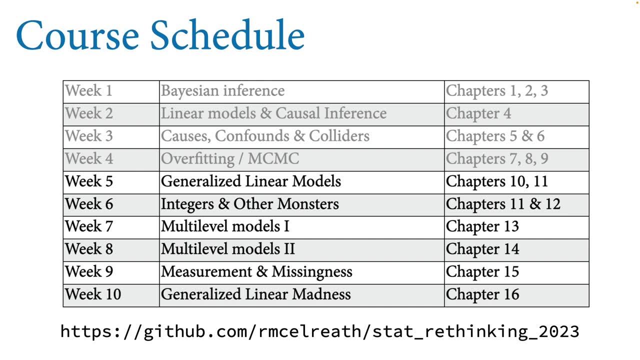 because the Markov chains will make it much, much easier. Okay, that has been week four. In next week we're going to start using Markov chains to visit new and exciting kinds of models. we can do, But most of the coding technology. 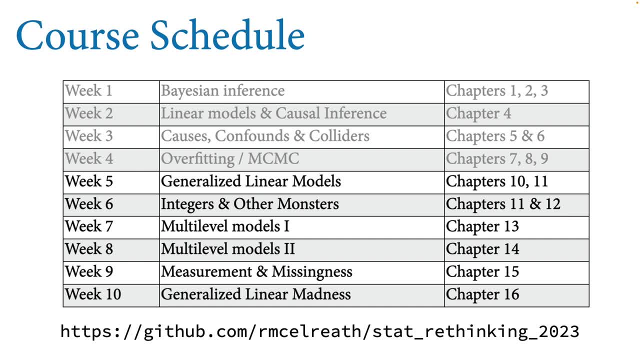 is in place. now for the rest of the course. There's no really new technical skills you're going to need to learn. The model formulas you're going to write are going to look very similar to the ones you've already been writing. They're just going to have 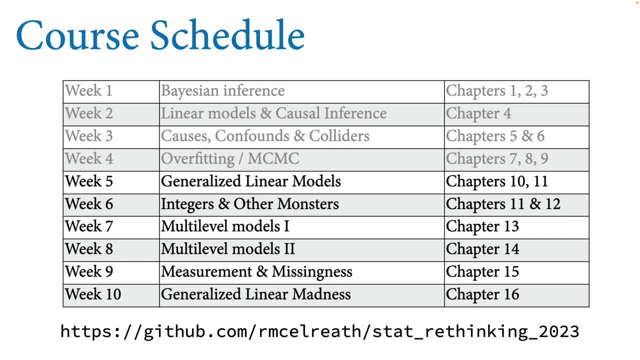 some more ornaments to them. Those ornaments are going to be expressions of scientific assumptions, So we're not leaving that perspective behind, And so I'll see you next week. 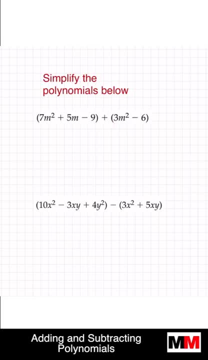 This 3m squared, the second set of parentheses. I'm going to write that term, 3m squared, under the one that matches with it, because they both have m squared And minus 6, you're going to write that and move it right under that negative 9.. That is just 7 plus 3, so that's 10.. You are not changing. 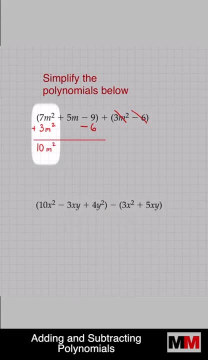 the exponent. Do not put m4.. That is just m squared. The 5m will just drop down and negative 9 minus 6 is negative 15.. When you have a negative in between the terms, you put a negative 1 here. 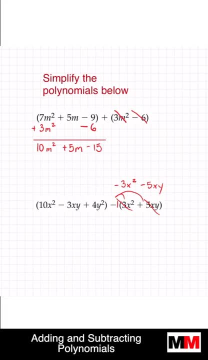 and distribute. And now it's just a matter of matching like terms, So that negative 3x squared matches with this 10. And negative 5xy matches with negative 3xy- 7x squared. do not change that exponent. Negative 8xy and you're left with 4y squared. Easy peasy. Like and subscribe.